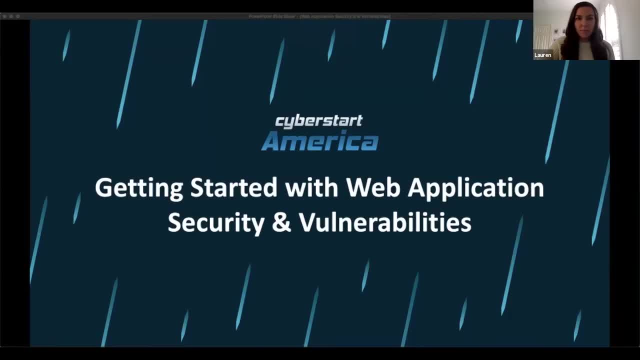 All right, we are going to get started in just a minute. Okay, Welcome everybody. Thank you so much for joining us today in our webinar. Getting Started with Web Application Security and Vulnerabilities. Today in this session, you will be introduced to the topic of web application security and vulnerabilities. 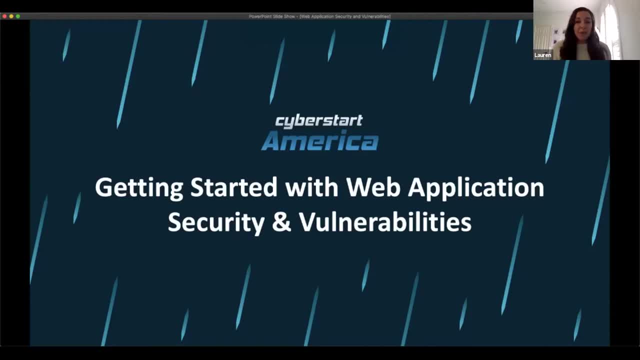 And have a look at examples and demos of real-world web application flaws worked on by cybersecurity professionals in the field. We're also going to show you how CyberStart America teaches you web application security through fun challenges and then also get an exclusive tour at a CyberStart game, learning all about the bases, the levels and how you can use. 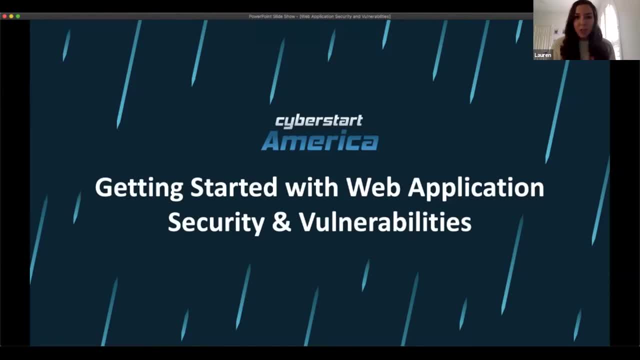 the field manual. Now, if you have any questions throughout this webinar today, please use the Q&A box at the bottom right-hand corner of your screen. Don't put your questions into the chat box, but put them into the Q&A box and we will answer as many questions as we can. 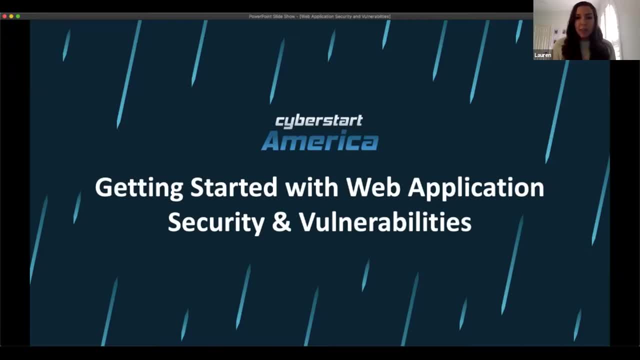 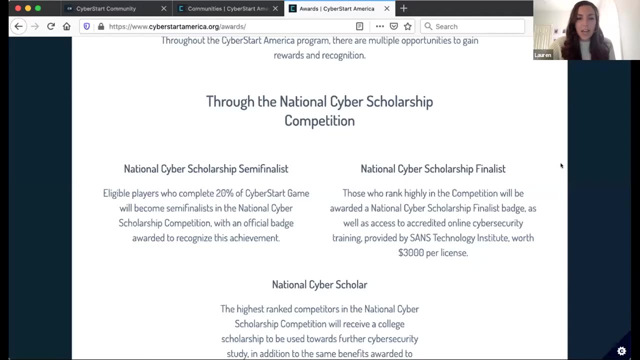 throughout the presentation, And then we'll also try and answer some at the very end. So before we kick off on things today, I just want to introduce myself. My name is Lauren, with SANS Institute, and I want to make sure everyone here is aware of what awards and opportunities come along with. 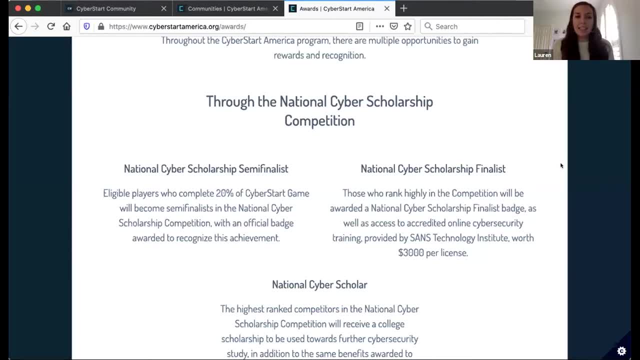 CyberStart America. So you get access to CyberStart Game and when you complete at least 20% of CyberStart Game, you are automatically qualified to partake in the National Cyber Scholarship Competition. Now, that's going to take place online on April 5th and 6th, and it doesn't mean. 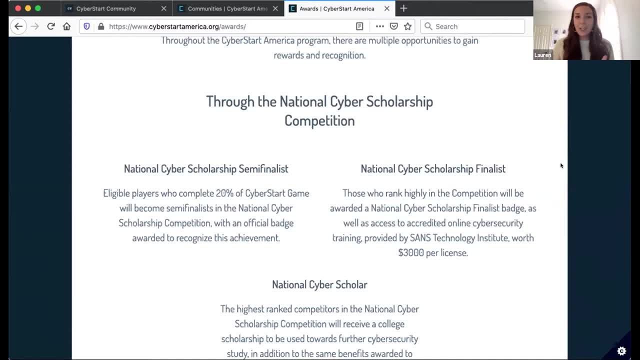 if you complete 20% game that you just end there. We highly encourage you to keep on playing throughout the competition and see how far you can get within CyberStart Game. The more you play, the more challenges you overcome, then the better you'll be prepared for the competition on April 5th. 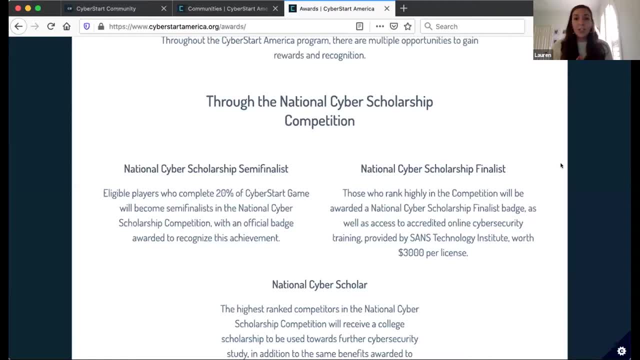 and 6th. Now, if you do really well in the competition, you will be ranked and be awarded a National Cyber Scholarship finalist. Now, what comes with that is that you'll get a finalist badge, as well as access to an accredited online cybersecurity training which is worth up to. 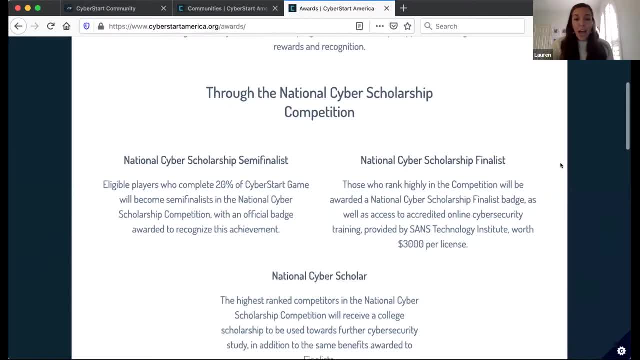 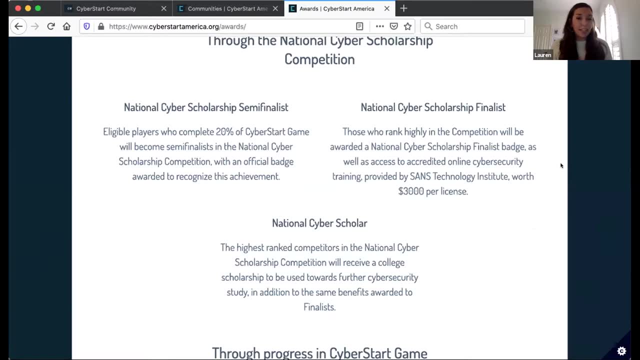 $3,000.. Now, if you are within the top of the competition, you are a National Cyber Scholar. Now that means you get the benefits of a finalist as well, as you will win a scholarship to an accredited university or college of your choice. Now you do have to be a high school. 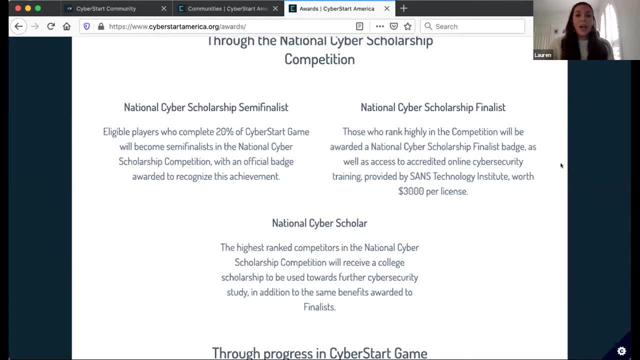 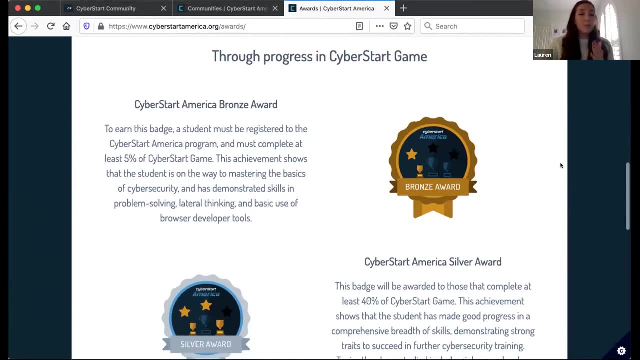 junior or senior to be a National Cyber Scholar. In addition to those awards, while you're playing game, you get access to a bronze award, which means if you complete just 5% of game- which I know everyone who is attending today can absolutely accomplish that- and then if you 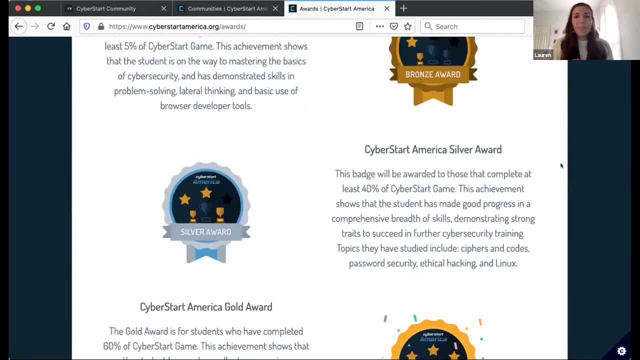 accomplish a bronze award, you get access to a bronze award, which means if you complete just 40% of cyber start game, that means you'll get a silver award. So that means you've covered things such as ciphers and codes, password security, ethical hacking and Linux. Now 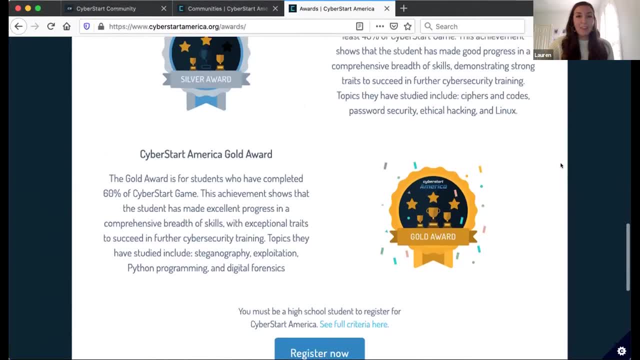 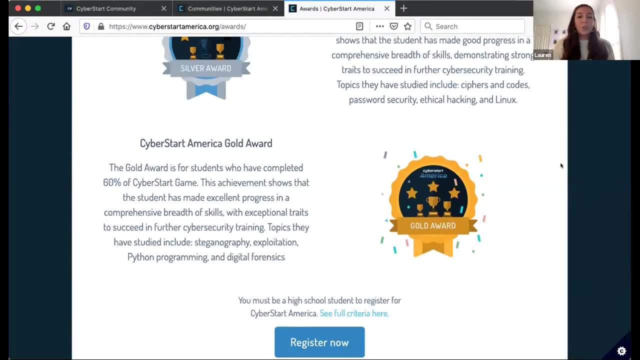 if you are really good at cyber start game and you complete about 60% of it, you will get access to the gold award. Now you might be wondering: well, what can I do with these awards? Well, you can put them on your social media. You can put them on your LinkedIn profile. You can put 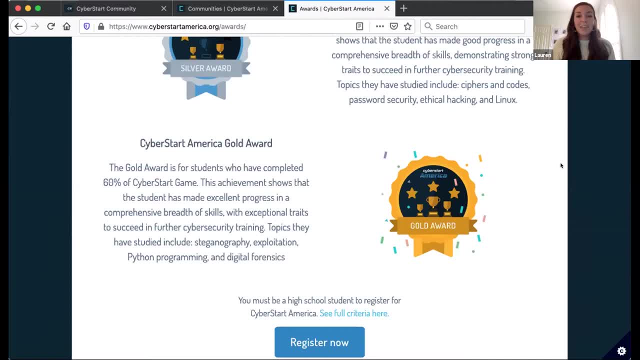 on your applications for colleges. This is the kind of stuff they want, This is the kind of stuff they want to see, and it really shows off how great you are. So, in addition to the awards, when you join Cyber Start America, you are also invited to be part of a 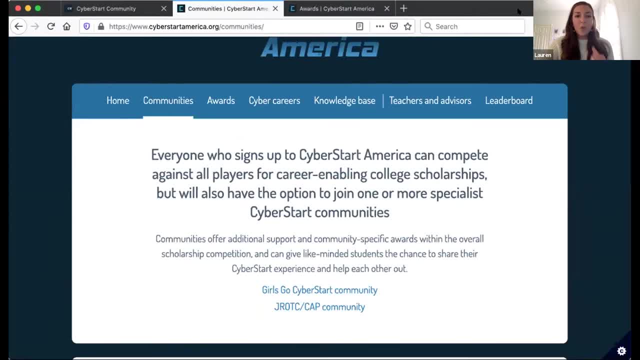 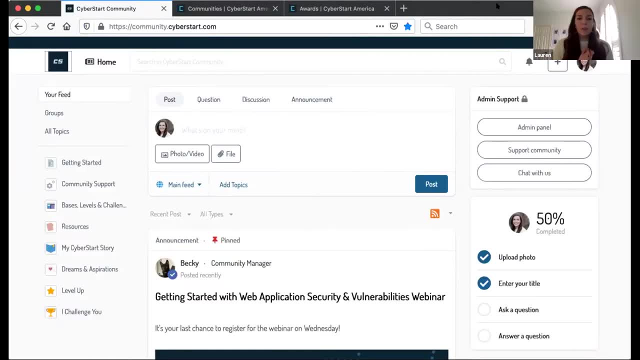 community. Now there's two communities that we have. One is the Girls Go Cyber Start community and the JROTC community Within communities. you are invited to a platform like this, as seen here on my screen, and it kind of has like a Facebook vibe to it, But here you're able to access the 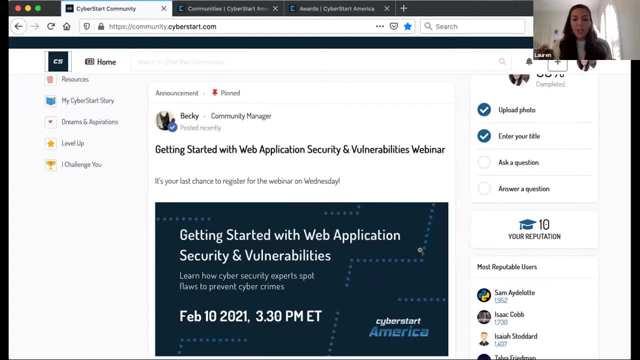 information that you need. You can ask questions with other students involved in Cyber Start America. You can work out problems together, You can post funny memes and create polls, but ultimately, it's here for you to be able to network, And so with that, we also want to point. 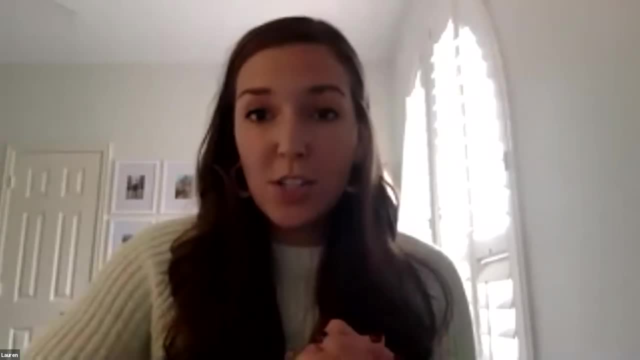 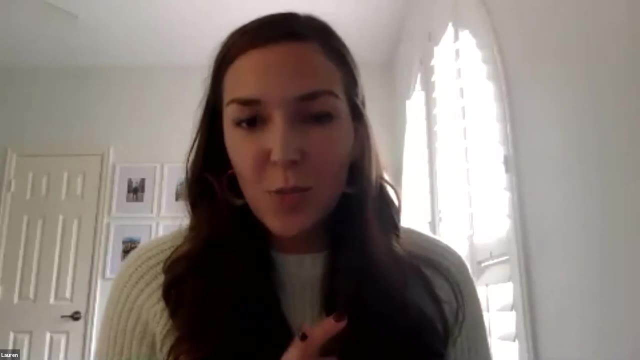 out that you can go and follow us on Cyber Start USA on Instagram and throughout the next couple weeks or in the coming days, we are going to be announcing a new giveaway. So if you follow us, you can go and follow us on Instagram and you can follow us on Twitter and you can follow us on. 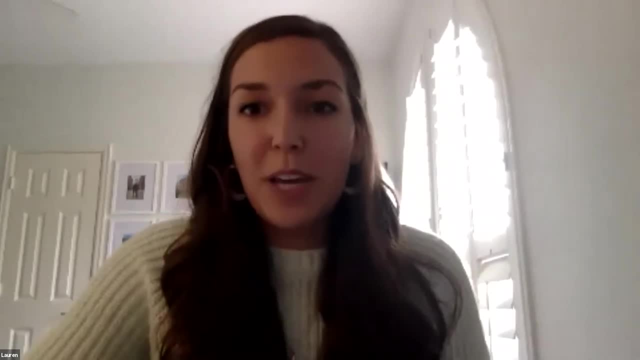 Twitter and you can follow us on Facebook and you can follow us on Instagram and you can follow us on Twitter and you can follow us on Facebook and you can follow us on Instagram and you can win some really cool prizes, And so we hope and encourage you to follow us there as well as join. 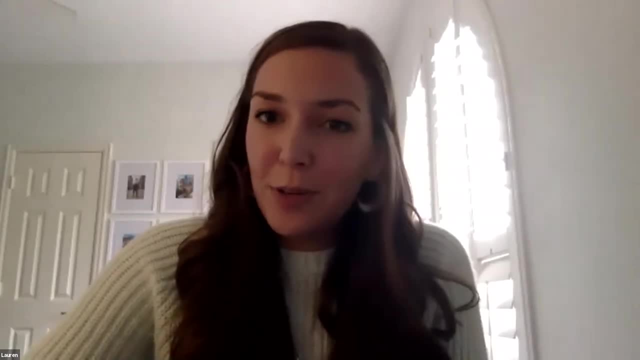 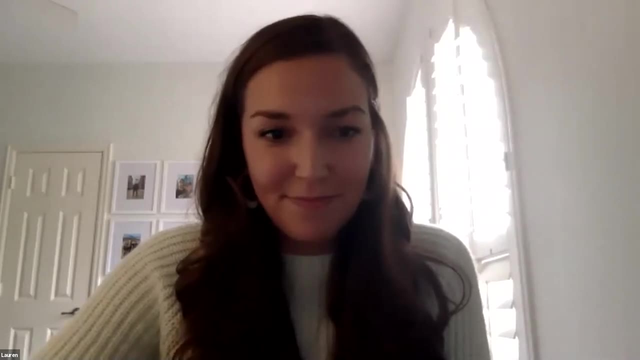 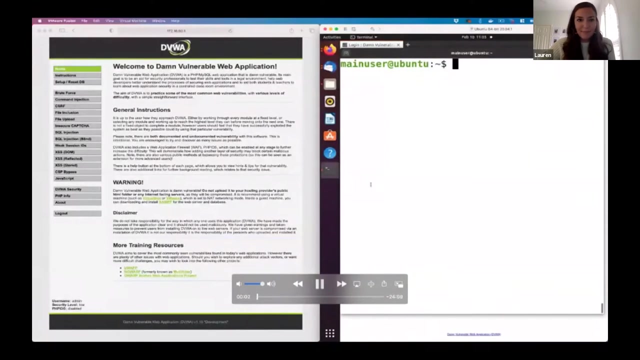 the community. So now we're going to play for you a recorded demo from the creator of Cyber Start himself, Mr James Lyne. Hello everybody, and I'm sorry I'm here in a pre-recorded context, but looks like today. 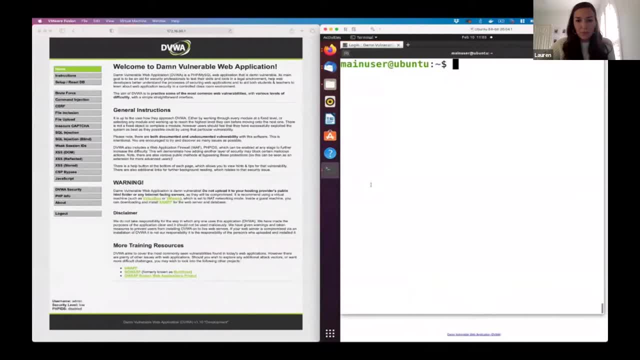 Wi-Fi is set. I'm going to be taking a moment to step out of Cyber Start game and show you some real-world examples with real-world applications, albeit in a slightly contrived context, where we can slowly increase the difficulty, looking at the various mitigations developers can. 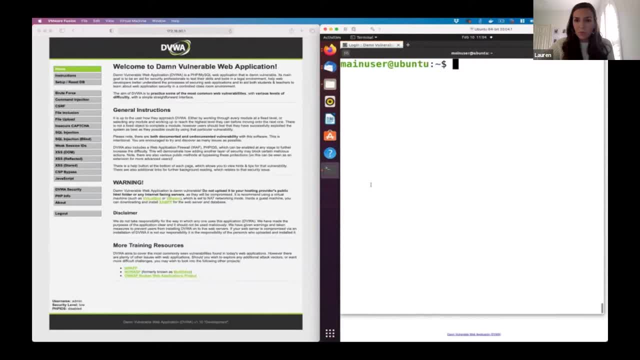 bring in where they think they've fixed security problems but in reality, have still left the door open to attackers. What I'm running here is a copy of DVWA, the Damn Vulnerable Web Application, and it was designed to be well, really vulnerable. 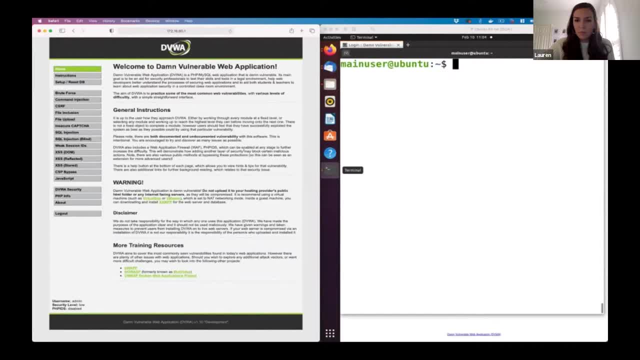 It actually includes lots of real-world attack vectors and you'll find challenges like this in-game as well, but the reason I've picked it is in this webcast, just to step away from game for a moment and show you some real-world tools and techniques that we use as security. 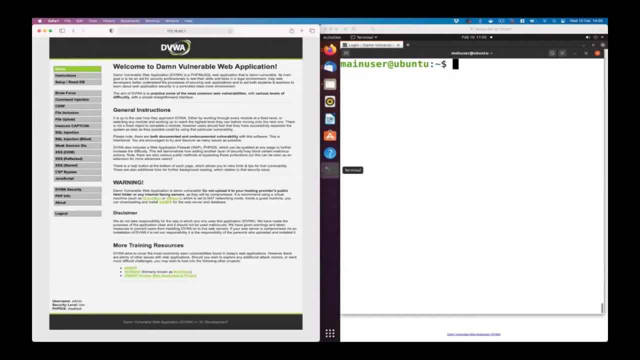 professionals. It'll show you where you're going in, what you're learning in Cyber Start game and what you can build up to Now. for some of you who are just getting started, some of these will be easier where. later on we'll look at some examples that are a bit different. 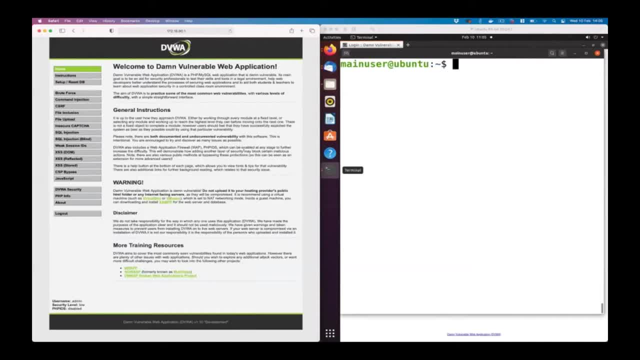 Some of them will be a bit tougher, and don't panic if you don't understand all of it immediately. This is something you can progressively build up to and you'll be able to watch this webcast numerous times. I've also got a Linux system over here which is highly useful for me to be able to run. 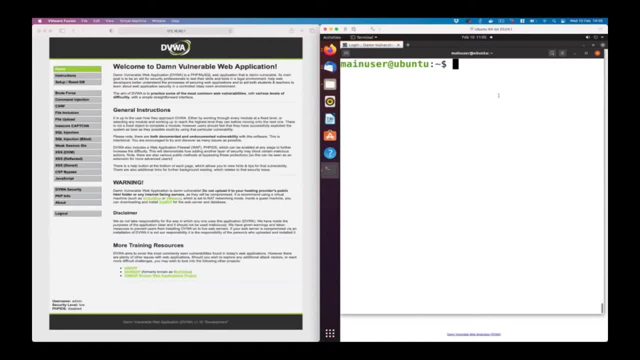 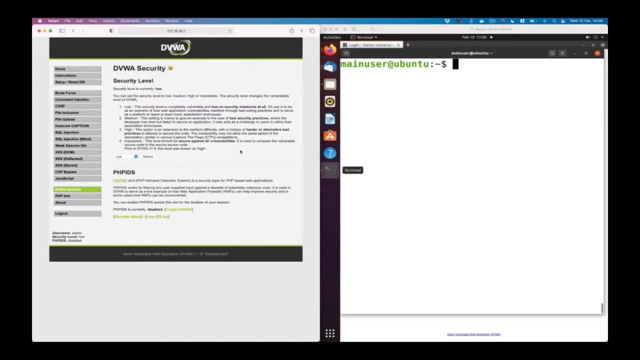 my various commands and queries here to help me with this testing process. So let's dive into a little bit of setup on DVWA to understand what it is we're going to be doing with this target. So we're actually running a copy of DVWA in Docker and there are setup instructions. 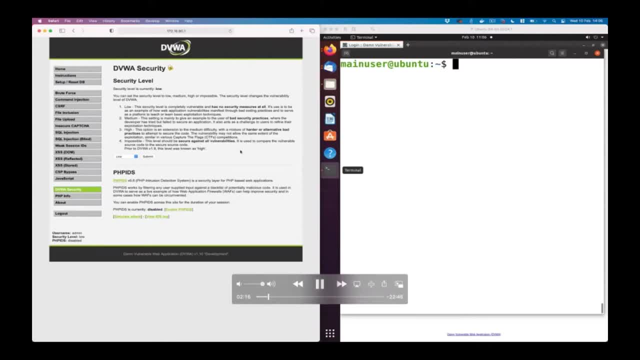 for this that you can find online. if you want to have a look at this yourself, It can also be run in a virtual machine, or if you're not feeling comfortable with either of those things, yet again, double back to Cyber Start game. 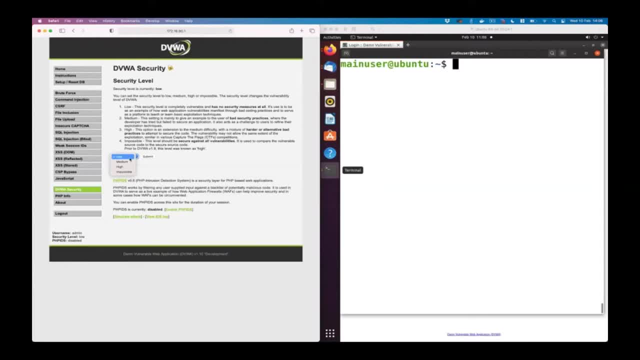 There's a security level that's set here that enables us to choose between low, medium, high and impossible, and this is reflective of the idea of really bad security through well-intending work. There's a lot of work from the developer that doesn't actually make it unhackable to. 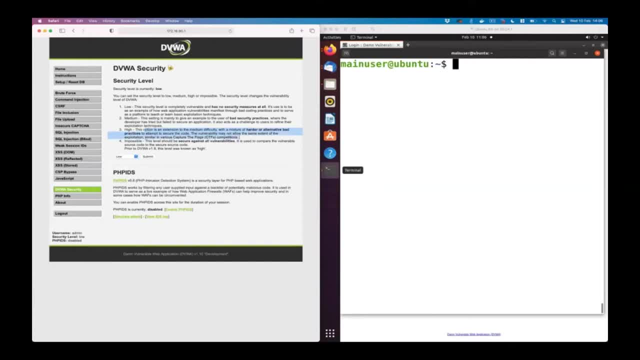 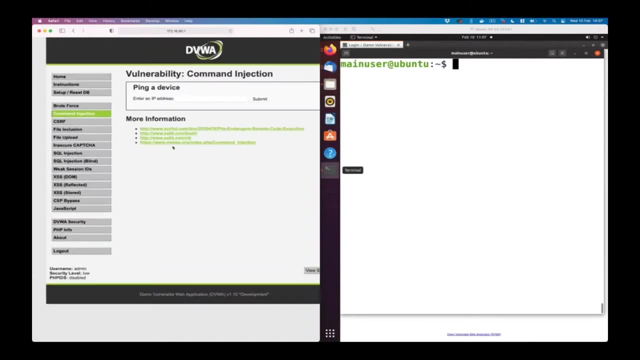 really quite hard to compromise but still possible. and then, in theory, what should be actually impossible to compromise, so we can look at the security fixes provided. Well, let's start here by just looking at a command injection example. and in this command, 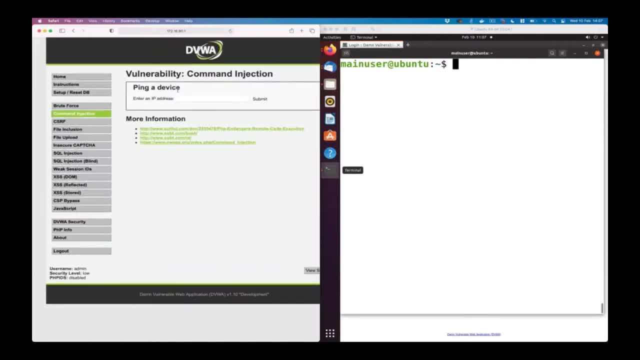 injection example. we are given a window where we can ping a device. so the idea is I could send a text like 1-2-7-0-0-1,, hit submit and it sends a ping to this particular IP address. 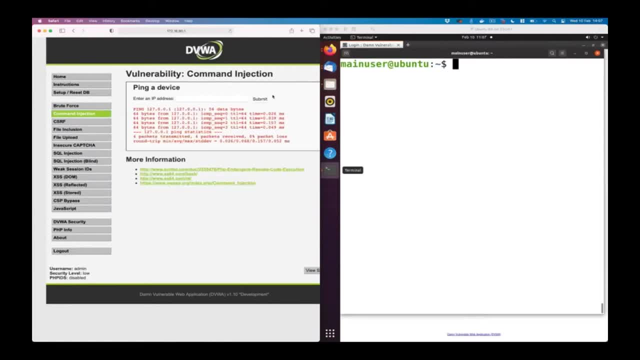 and returns the results. There we go. that's a ping. right there, we've got four pings to my local host and in theory, this could be a system on the internet as well. Well, what's happening here is this particular text field is getting assigned as a variable. 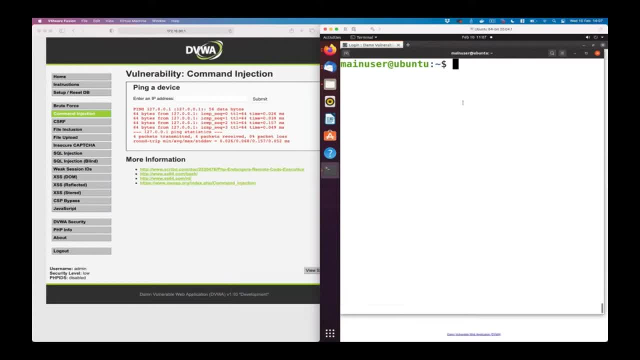 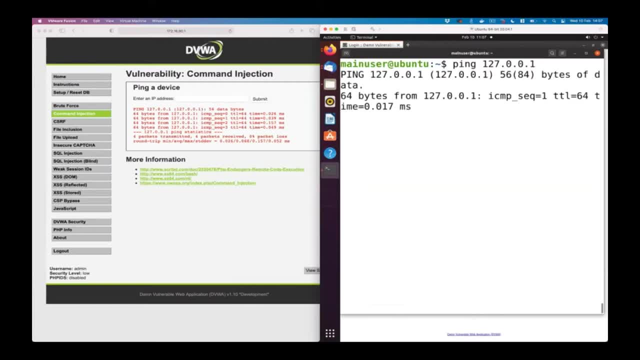 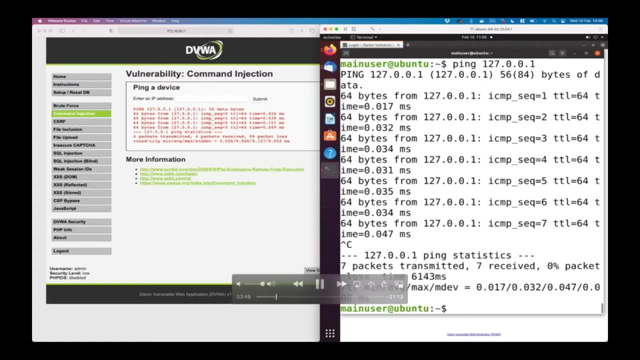 It's called a text field. It's called a text field. It's called a text field In fact. if you look at that, you'll see the text is remarkably similar. Of course, in this instance it's actually running forever, so it might be the command. 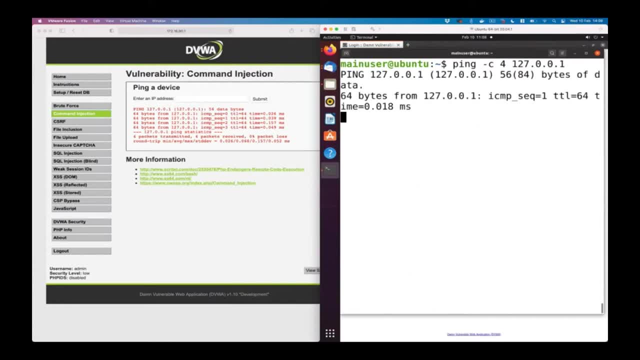 actually being run is something like ping c4, which is four counts of a ping before it's returned. In reality, this actually means we're doing ping c4- user input, where user input is something like this, something that we control. Well, this gives us an opportunity as an attacker here, If 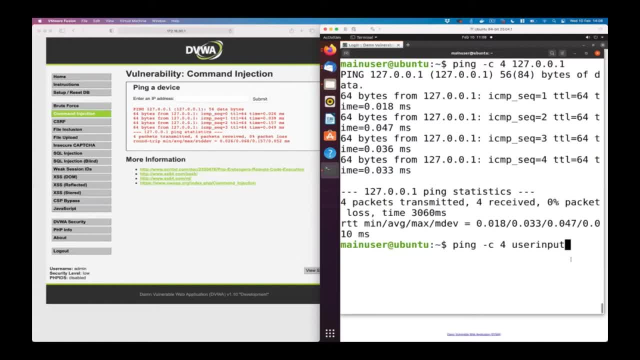 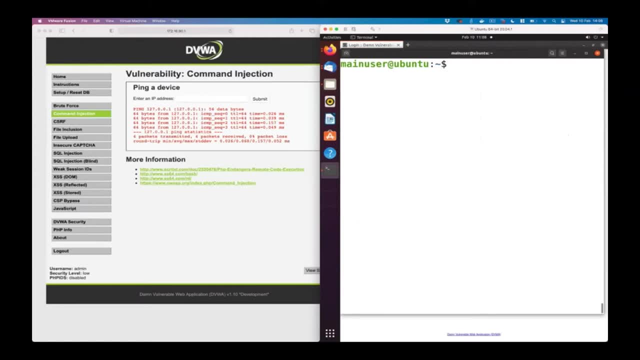 we know this is actually running via a shell. it's potentially vulnerable. Remember, in Linux, as well as alternatives in Windows, we can run one command after the other with a semicolon. For example, we could do something like echo hello, followed by ls, and when we run this, 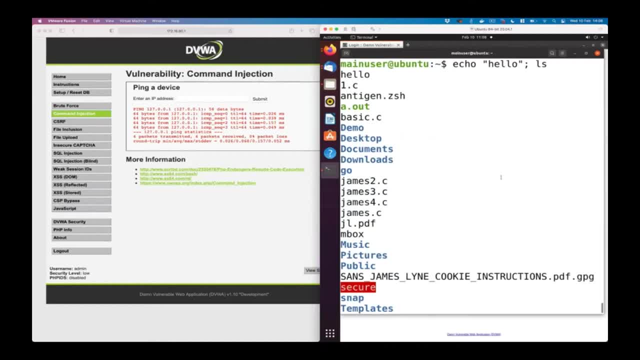 it runs one, then the other, We get the echo and we get the ls as well. So if we can do that, going back to our ping example, what would happen if we used semicolon ls on the end? Well, in theory it'll run the ping and then run the ls, and that should work on our target. 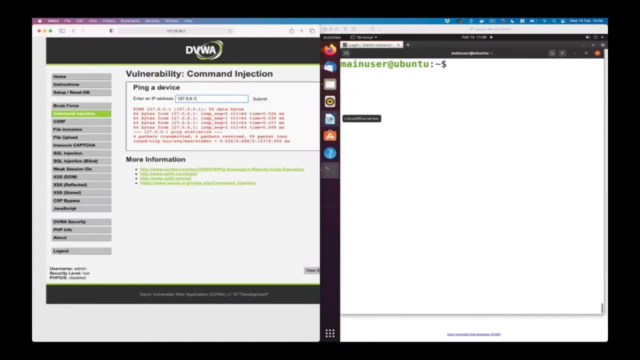 system here as well. So let's do that: one, two, seven, zero, zero, one semicolon ls. Let's submit it, Wait for the pings to complete in the background and look at that. The ls runs and we see help, index, php and source. So we could do something like one, two, seven, zero, zero, one cat index. 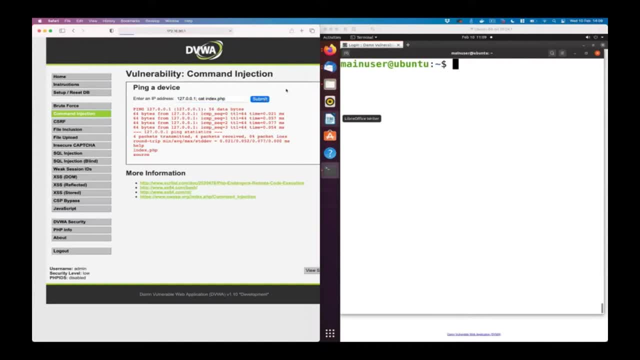 dot php, and now we should be able to see the code behind this page. Look, it looks really familiar. you can actually. you can actually see some of how it works, albeit looking a bit strange. We might also be able to access privileged files on the system. One, two, seven. 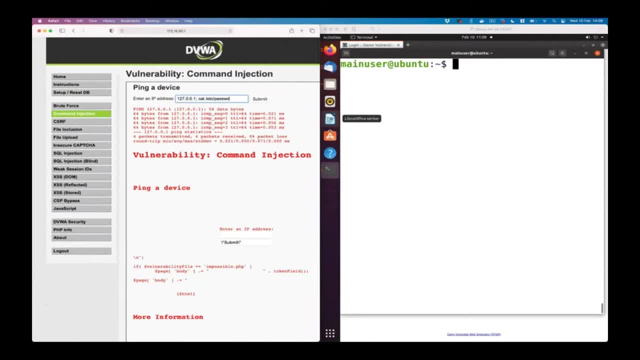 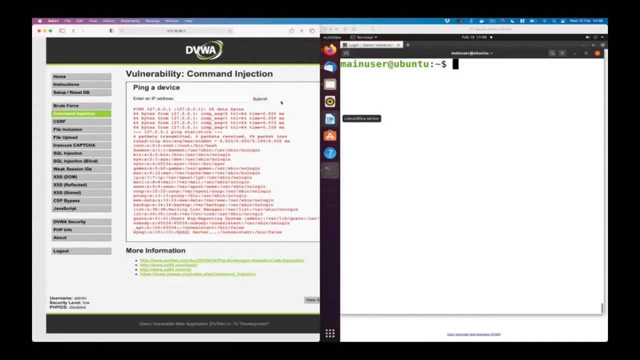 zero zero one cat slash exe, slash password, which is a file that has a list of users on a Linux system, And in this instance we can trick the web server into showing us this user list. We could also get into tricking it into opening a back door. So the mistake. 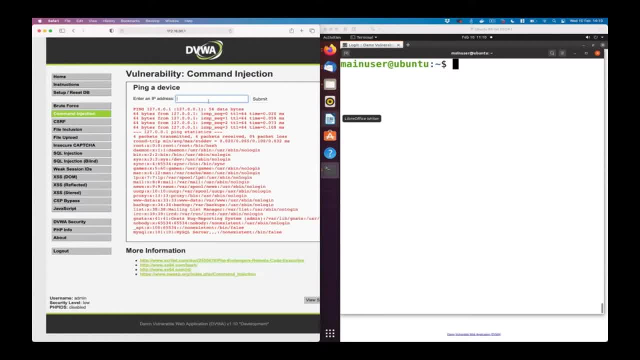 here is a seemingly useful piece of functionality for network checks. being passed to a shell enables us to be able to trick it into running other things, And this is where the device developer needs to filter their inputs to make it so we can only supply the expected. 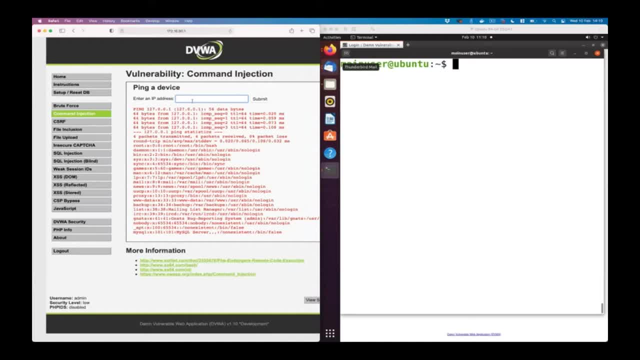 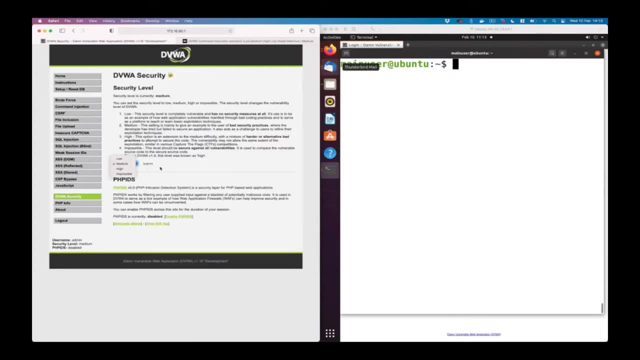 data. A pretty neat little example of command injection. Okay, let's step this up a gear. Let's just jump over to the security level here, and we've got it set to medium instead of low. So that means now that the developers done some work. 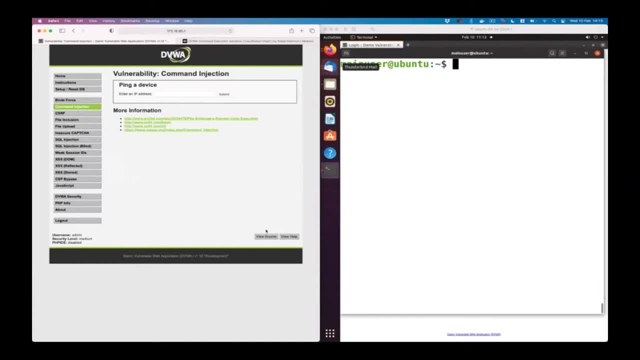 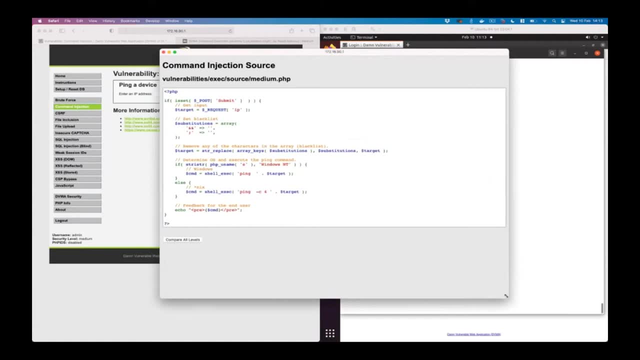 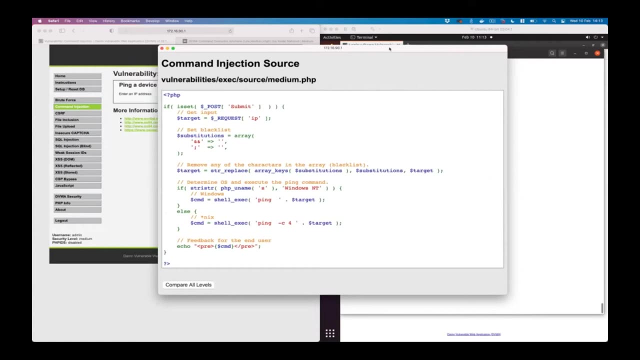 to make this attack a little bit more difficult? Well, let's kick view source here. and this shows us the server side code that is behind this particular page. Now, normally we obviously don't get to see that. Of course, in modern day security testing we're often given the 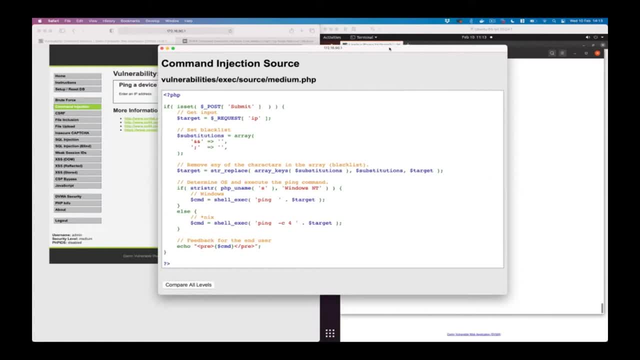 code to be able to help a client to test their implementation. so we can go quicker than guessing like a raw attacker. But what's interesting here is this piece: If we look at this, this is the piece that's been added between the server side code and the server side code. 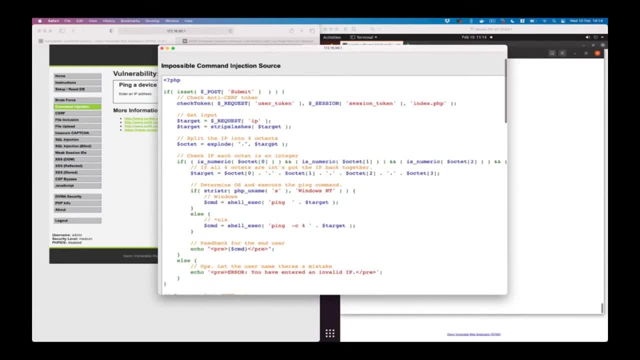 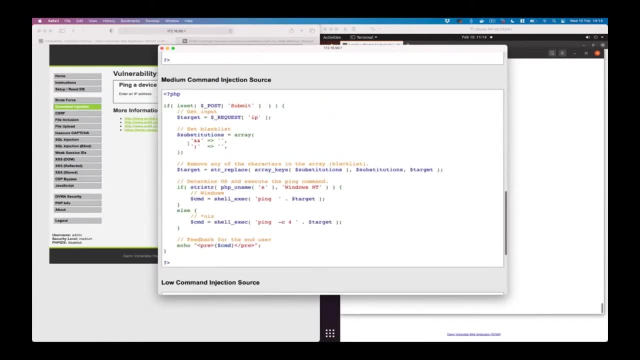 We can actually click compare all levels if we want to. This is the impossible. This is the high, This is the medium And the low. here lacks this section, which is a blacklist. You'll notice here the semicolon and ampersands have been added, And this is the classic thing. 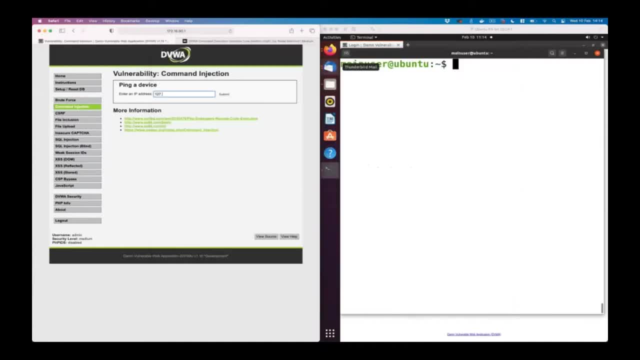 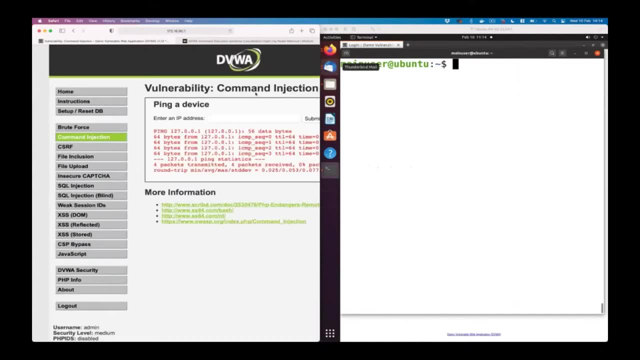 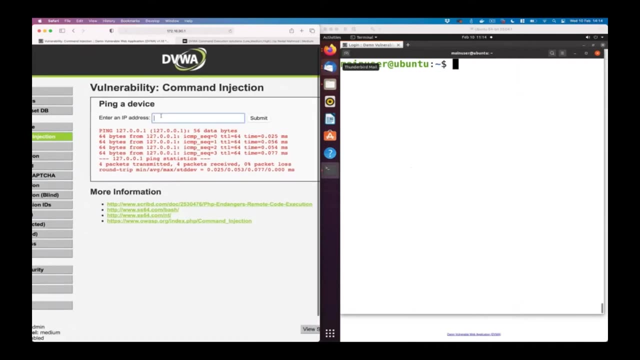 a developer will do to try and fix the problem. So if I now do one, two, seven, zero, zero, one semicolon LS, We get our ping results, but we don't get an LS result. It's been filtered. Well, the answer here is to find a way around it, to evade it, If we do a little bit of searching. 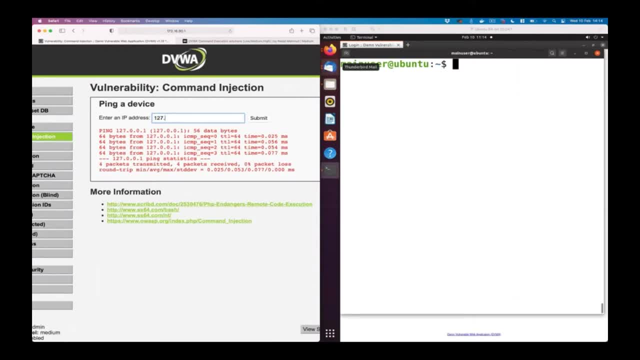 we'll find. there's multiple ways to be able to get this to work. For example, we could do one, two, seven, zero, zero, one, like this, and we could pipe instead. This character, instead of the semicolon, enables us to pass the output of the previous command through to the next. 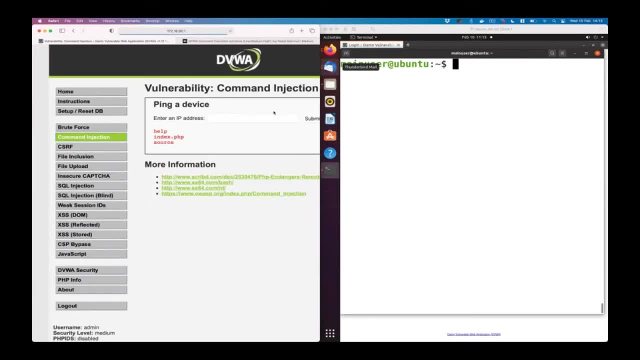 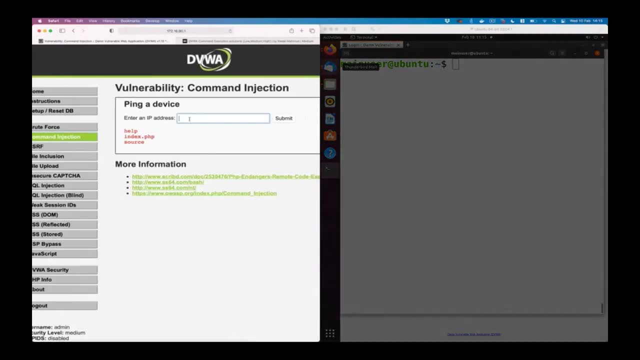 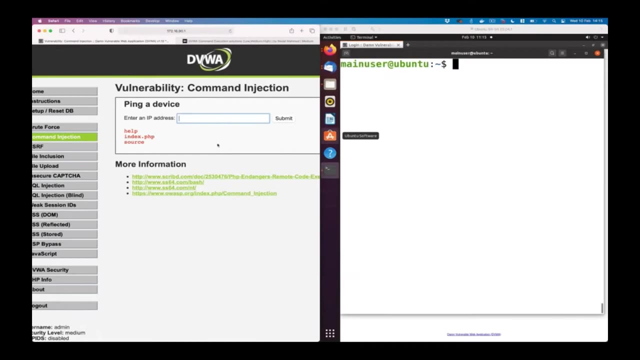 And that isn't on the filter list, but it's another way of chaining things together in Linux. And look at that, We have our index PHP, So once more we can run LS or we could run cat, just like before. So this shows us that it's really important when we're behaving. 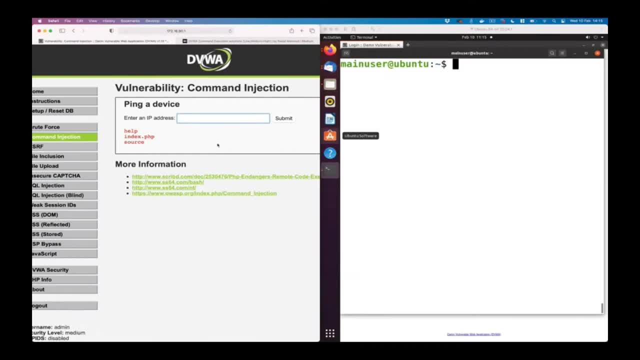 like a developer here trying to write secure solutions. It's not about blacklisting things we know are bad, but often it's about whitelisting the known good things. We are likely ought to be validating that you can only enter an IP address, the expected types of data or 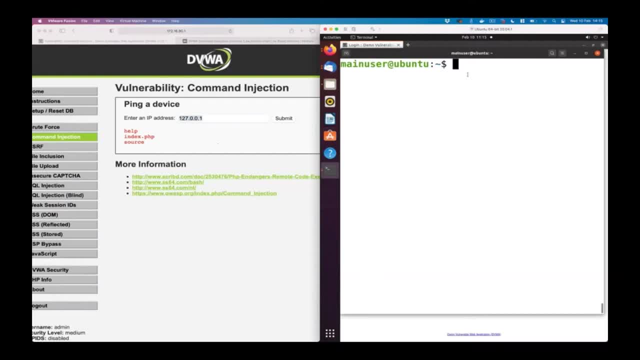 better still, not passing this via a shell prompt at all, where these numerous types of workarounds can be found. As security testers, we get to be creative, finding multiple ways to bypass the restrictions that are put in front of us, And this is a pretty neat example. 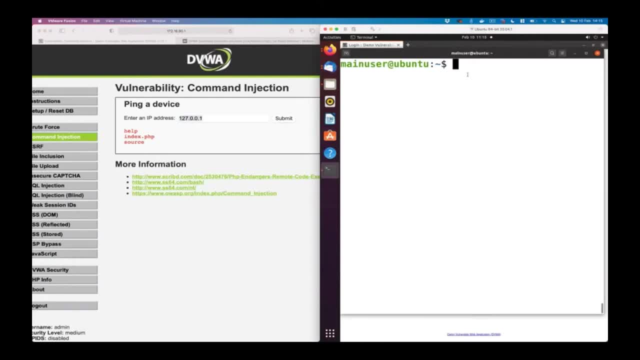 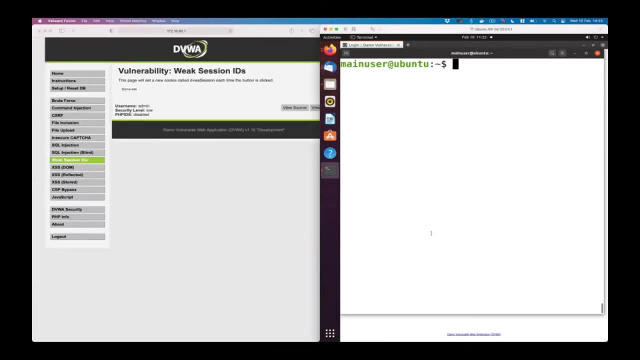 of the dangers that come with a blacklisting based strategy, and how command injection and a web application can provide us with access to a server and the ability to navigate data or even spin up a backdoor. So let's just take a quick little look at session IDs and 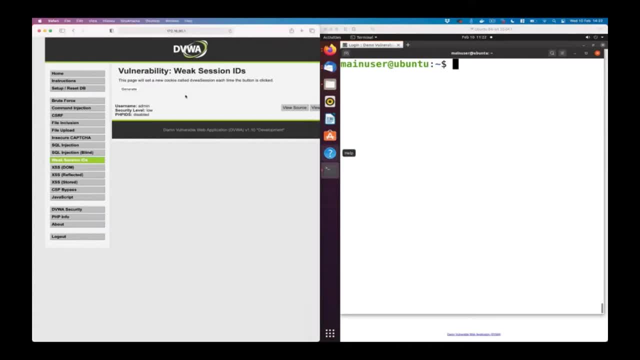 then we'll round out in SQL injection. The idea of a session ID is: it's a piece of information, typically stored in a cookie on your computer, which enables you to be identified as you. So when you log into a website and you provide a username and password, You can use that. 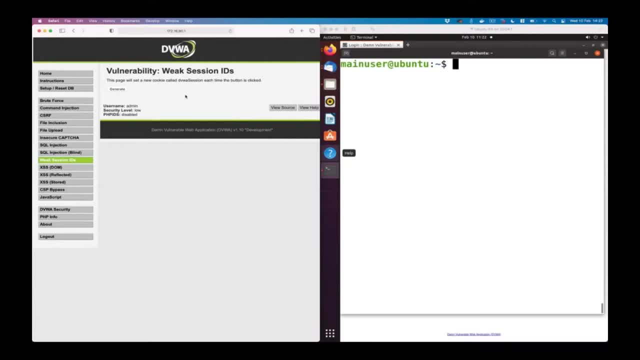 password. It's a value that's unique that you present to the system to say: hey, that's me. That means when you come back to that server again and again after logging in, it can still identify you as that user. Well, let's have a look at a simple example here. 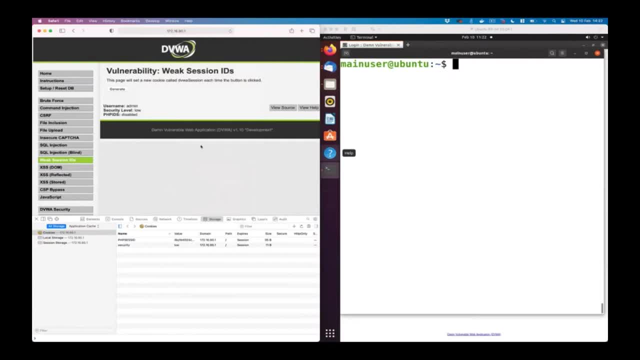 of where this can go horribly wrong On this page. here, I actually have a browser tool brought up that enables me to look at the cookies that have been set. There's one called PA HP session ID and one called security, and they're a little tiny here, but it won't let. 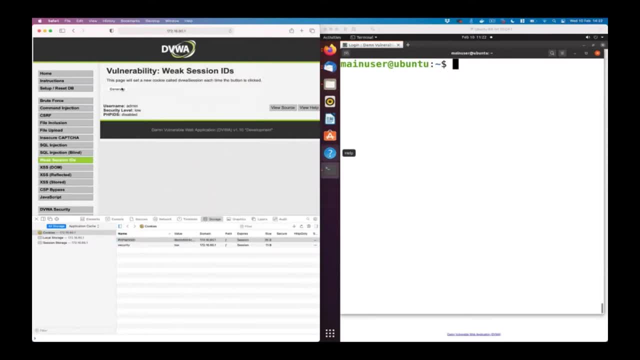 me zoom them up Now. if I took this generate button, this particular application creates a new session called DVWA session. It's stored as a cookie in this first line and it has a value of one. If I click this, it goes to two, then three, then four, then five and six. 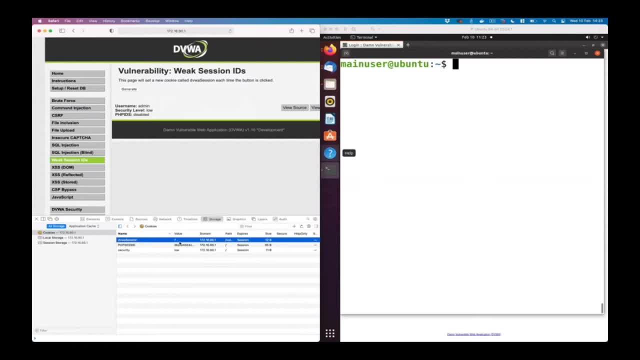 and seven. Now, this is particularly dangerous because it means the session IDs are very predictable. They're very easy to figure out. That's dangerous because if another user comes to this site and simply sets their value to seven, my session ID, they become me the administrator instead of them. So of course, there are more impressive schemes that are 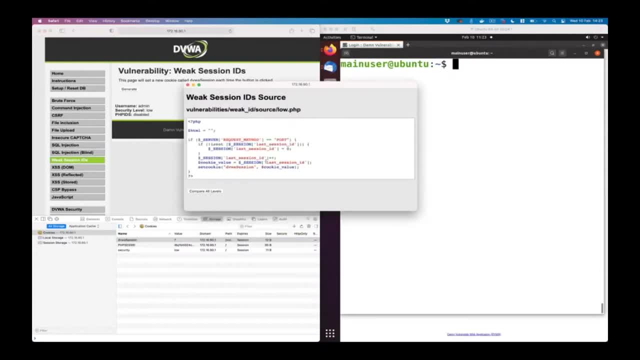 available here which can generate more randomized values. This one is simply augmenting by one, But other examples of this include maybe setting it to one and then putting it through a hashing algorithm. As long as the data is predictable in some way, you may be able to identify this. 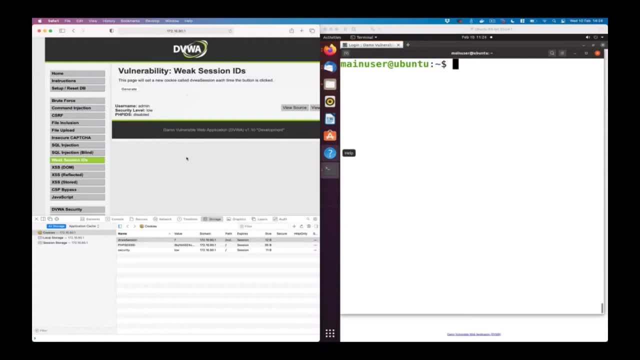 likely value, set it and then hijack the account of that person. And this is an example of having a little play with yourself, maybe even escalating the difficulty a little bit and having a look at how it varies if you're using a slightly harder setup. 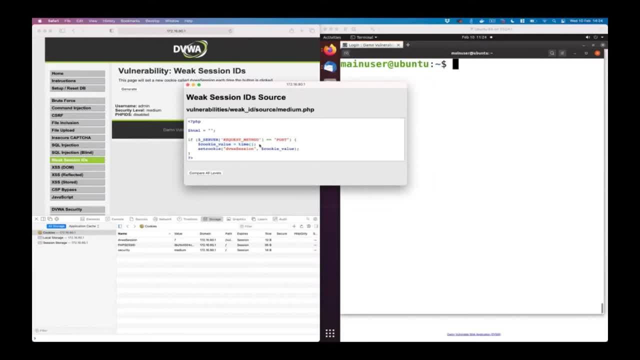 This one uses time. Now again, time seems like a good idea. I generate it and the time value is written here as a decimal. But time isn't actually that hard to guess, If you think most people will have logged in the last 24 hours. I could iterate through trying each of these. 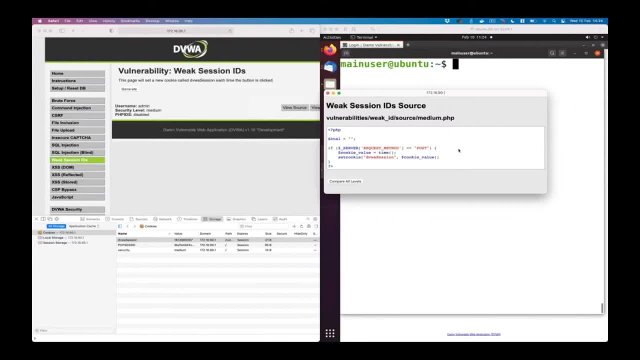 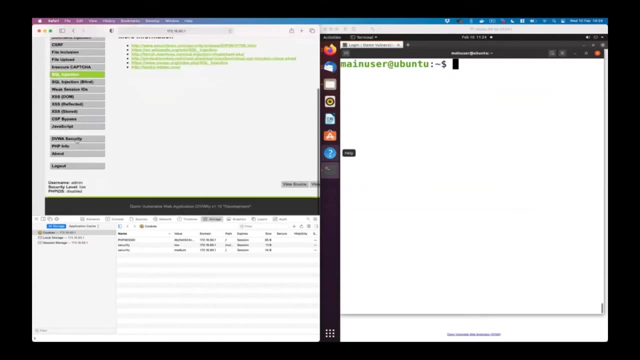 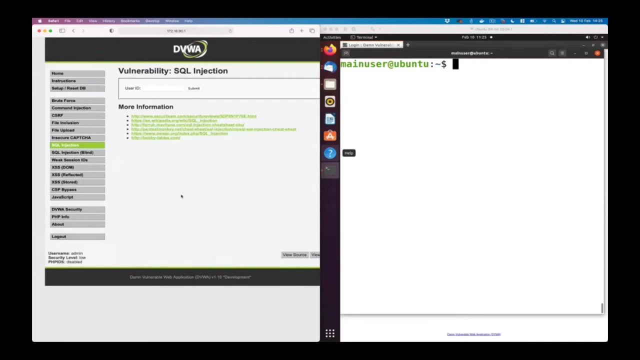 values, one after the other, What seems like a secure implementation quickly falls apart. But on that topic of what seems like a secure implementation, let's look at something really a lot more advanced here, and let's look at SQL injection. Now, if you've no experience of SQL at all, I strongly recommend a starting point here of 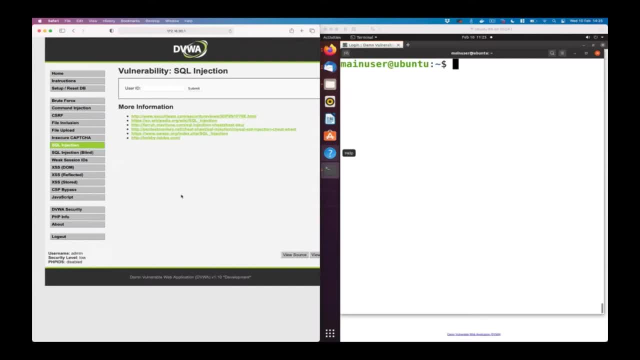 actually just going and looking at some basic SQL examples. SQL provides us with a database and a way to run queries. So, for example, if we have a database with a table of information called users, we could do things like select first name from users where last name equals. 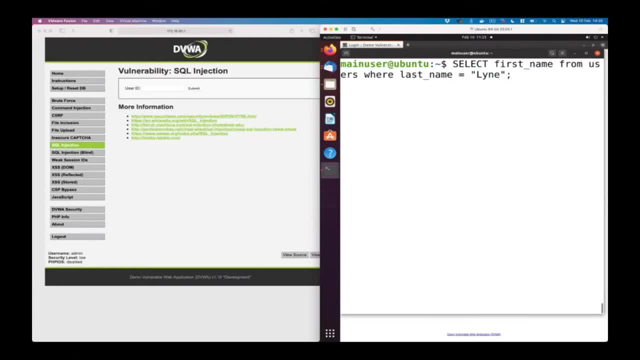 James Lyne. Now, this is actually just being typed into a bash prompt here rather than sent to a database, But it would go to that users table where information is contained with lots of users, and it would select the first name match based on the condition. last name: Lyne. 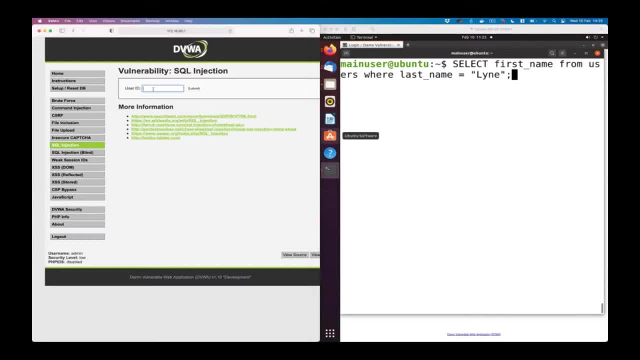 And that's exactly what's happening with this little search here. If I put in a user ID of one, I get admin. two, I get Gordon Brown. three, I get hack me. So it's presumably the case that a query like something like first name, last name from users where ID equals one, two or three is being executed And 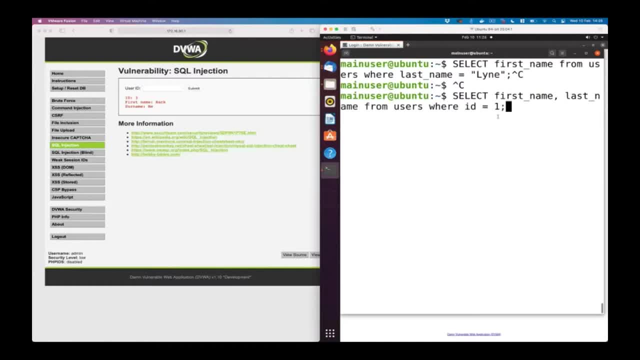 this is just a nice, convenient way of asking for something, So let's go ahead and do that. Let's go ahead and do that. So this is just a nice way of asking for something, So let's go ahead and do that. And then this also helps us out a little bit in the way of asking the database for information. 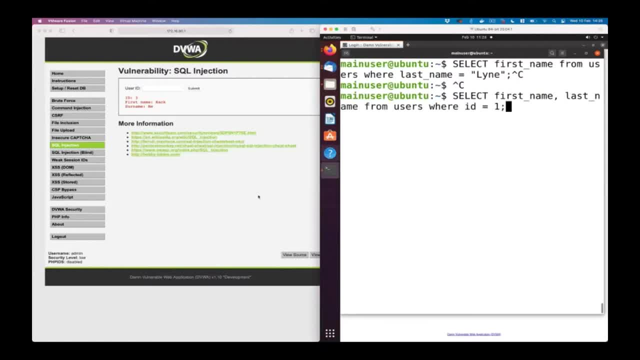 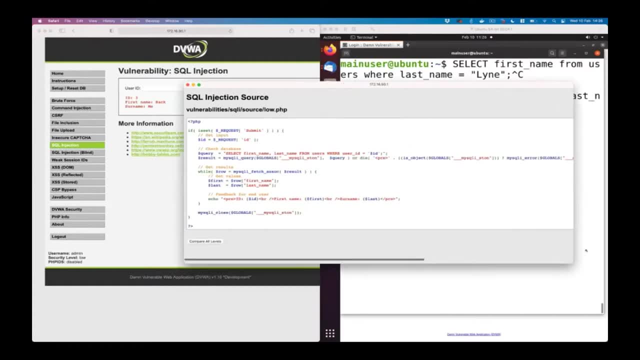 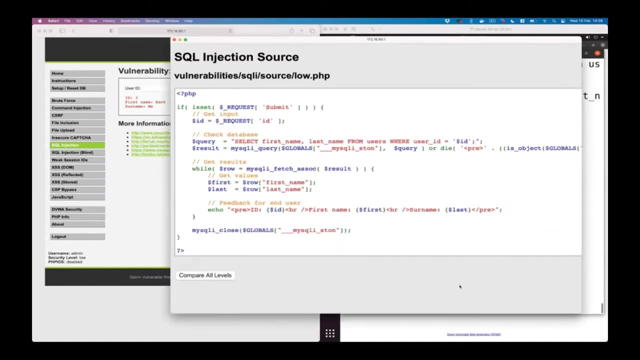 And that in of itself doesn't seem that dangerous. But again, filtering issues can lead to real problems here. Let's have a quick look at the source under the covers of this web page to see what might be going on and then how we might compromise it. Well, this looks a little bit more. 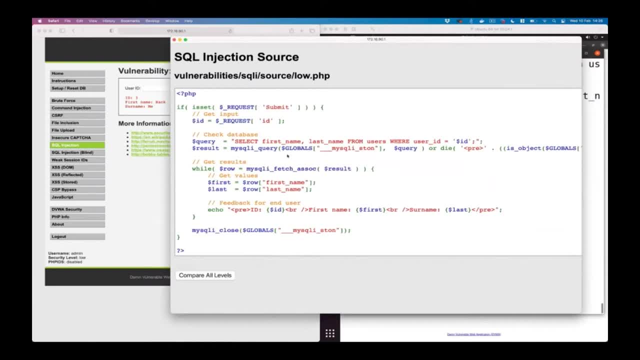 complicated than before, But, like any good security professional, we're not going to panic. We're going Get the ID value from the user's input. So that's what we're providing here: the 1,, the 2,, the 3.. 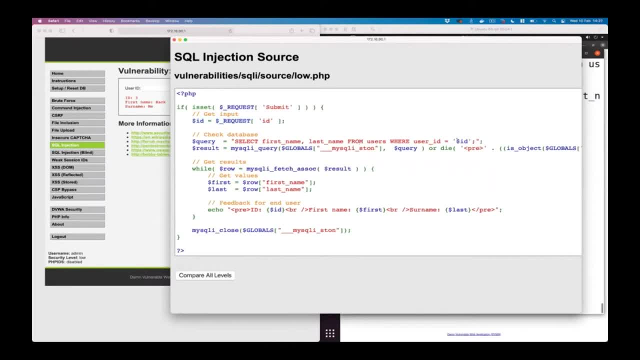 Select first name, last name from users where user ID equals the ID value we provided. I was so close to correct, just guessing before we looked. Well, this then returns results and grabs the row data first and last and shows it on the page. 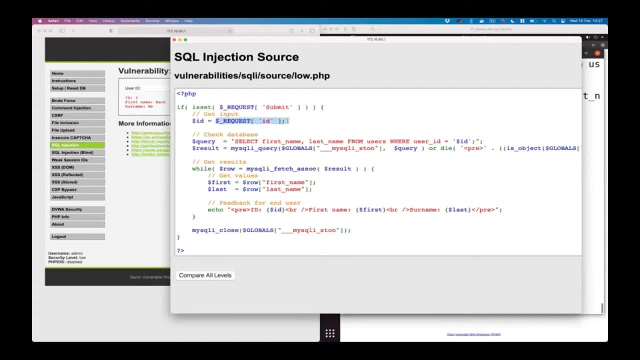 The problem here is the ID value is controllable by me, the user, and it goes directly into the SQL query. But we might be able to trick it into running other queries. For example, we could say: select this query where user ID equals XYZ. 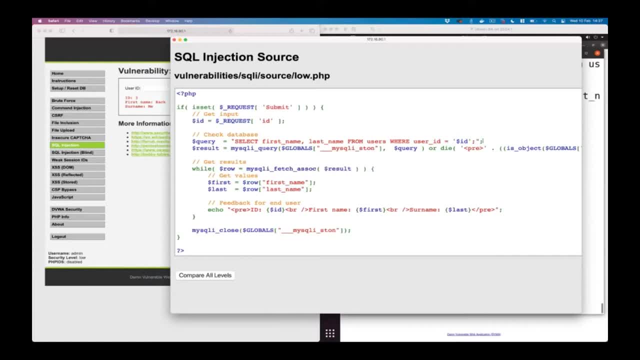 and then append a kind of AND. please also query this other information, because we control this piece here To test that theory as well. note here that when we try and run the query, it'll actually throw an error if the query is bad. 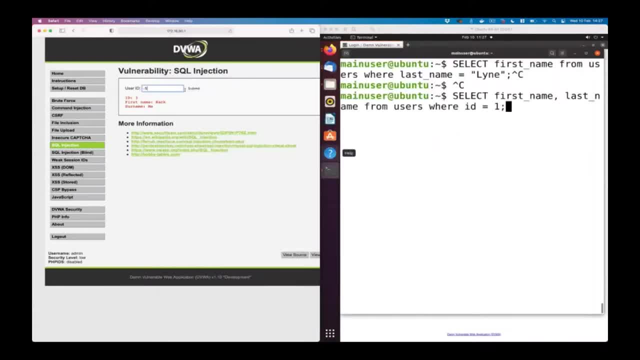 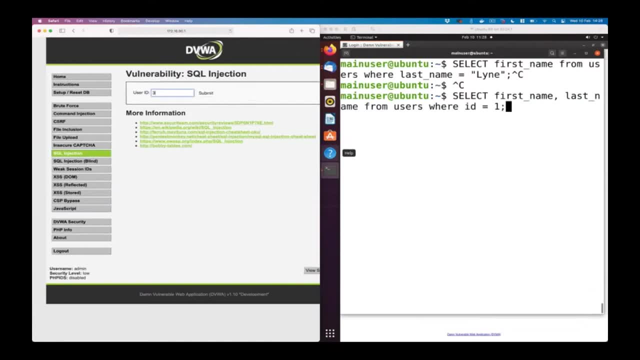 So let's round this out. Let's add a user ID of minus 1.. Well, we don't get any returns because there's no user ID of minus 1.. Let's run 0.. Let's run 3,, 4,, 4.. 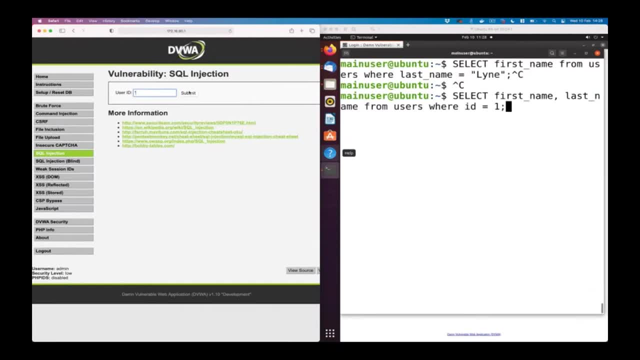 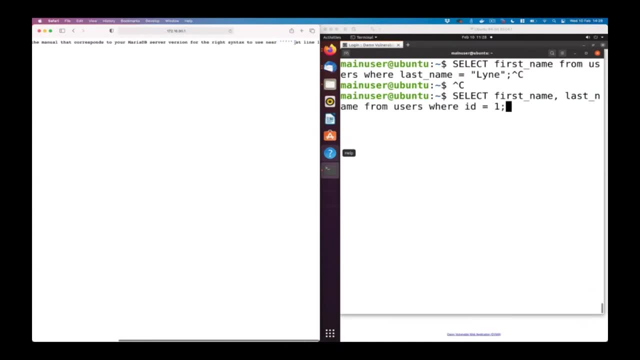 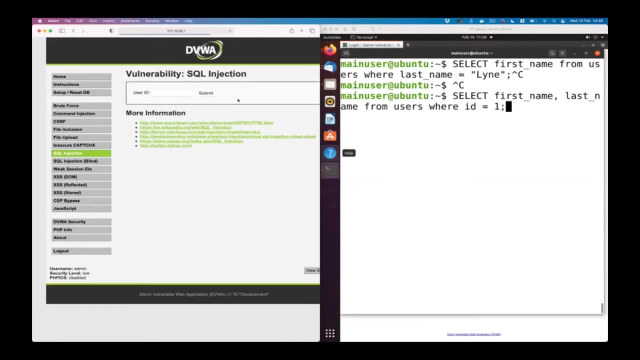 Nothing, But what about just the apostrophe Interesting? We get a SQL error. We get a SQL error near tick, tick, tick, tick, tick. What about the dash? And that did nothing? What about the semicolon? Okay, 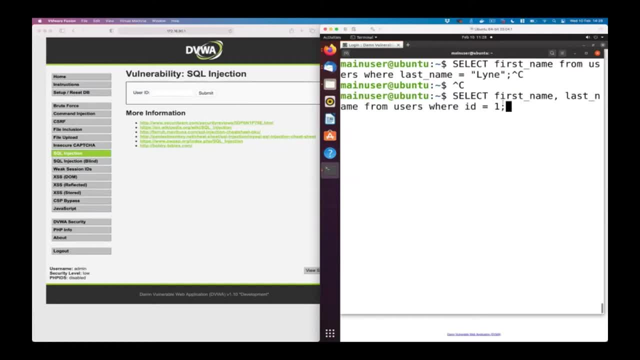 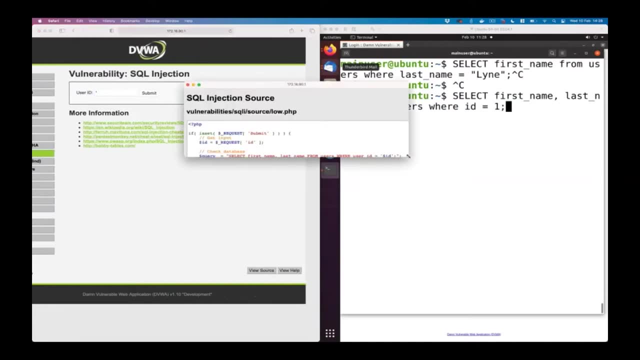 So certain characters related to this query cause it to throw an error, namely something like this: Well, that's because, again, if we go look at our source code here, what's happening is it's creating a query like select first name, last name from users. 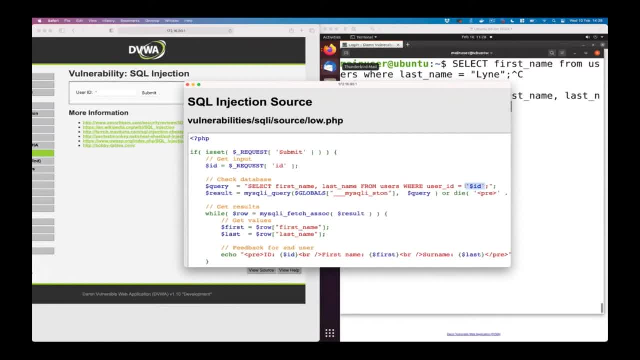 where user ID equals apostrophe, apostrophe, apostrophe. Well, that's three apostrophes, leaving the query unbalanced. It causes an error because it's bad syntax. So that shows us that we ought to be able to control this query in some way to get out data. 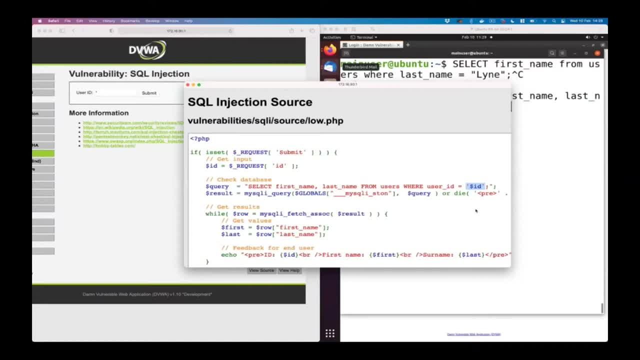 Well, we could go and do this manually, but given we have limited time on this webcast, I want to jump a little bit to having a tool. do this for us And then Caitlin will show you some challenges where you can build up to doing this on a more manual basis. 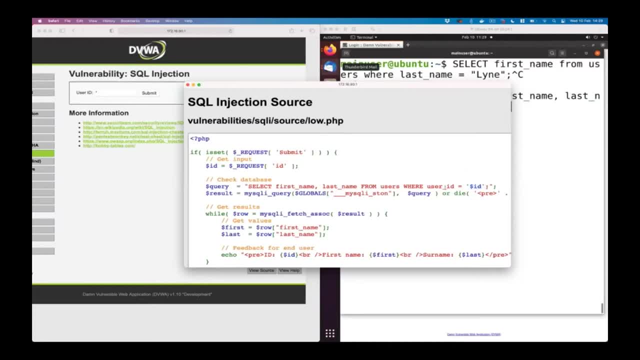 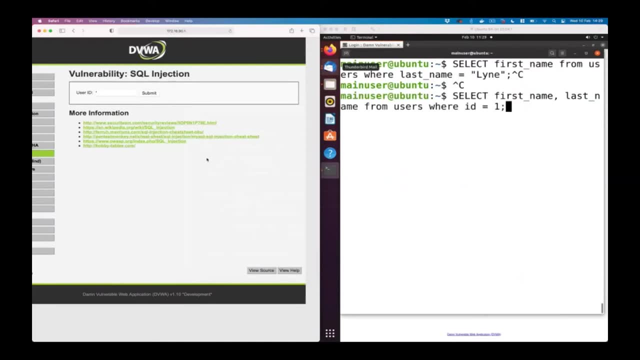 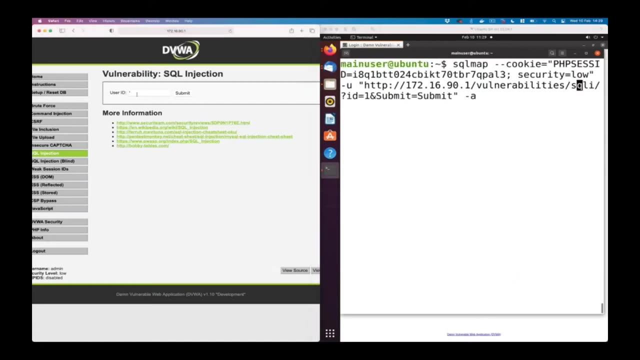 We know if we can control this, there's a way to get the SQL query to give us more information than it should. So let's do exactly that. Well, here's a command using a tool called SQL map, which I prepared earlier. 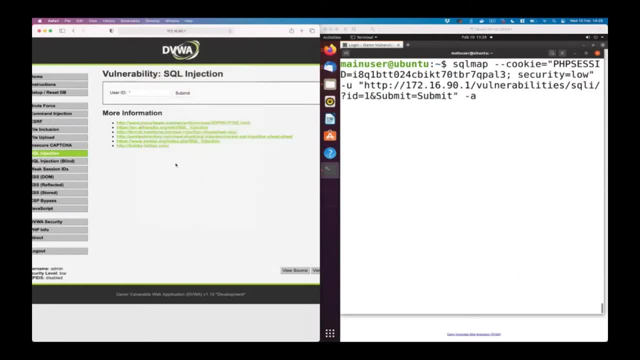 I'm going to explain now, but just need to update to work with this website here. SQL map is designed to find SQL injection flaws and automate the process of recovering data, So it's going to figure out what we can set this ID value to that enables us to retrieve information. 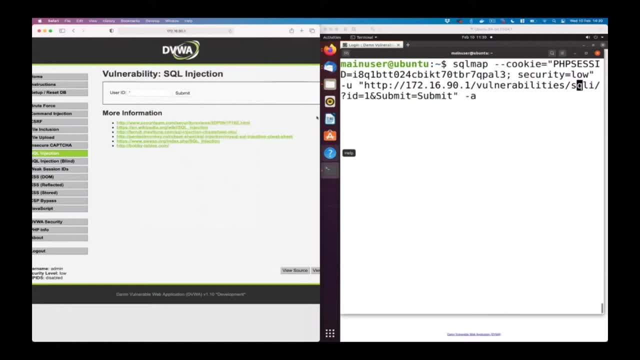 In order to be able to retrieve information, it needs to be signed in as us. So, as we were talking about with our session guessing, it needs a copy of the PHP session ID, which is this data Here, And in this instance, I've pasted it in to this cookie argument. 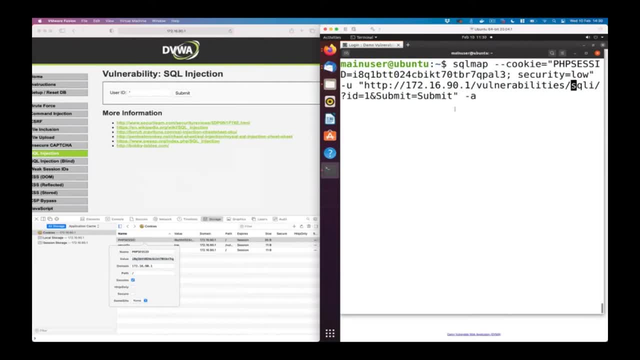 That means when SQL map connects to the site, it's going to be signed in just like our web browser. Okay, So even though it's running on the command line, it's going to seem like it's the same as what we see in our web browser. 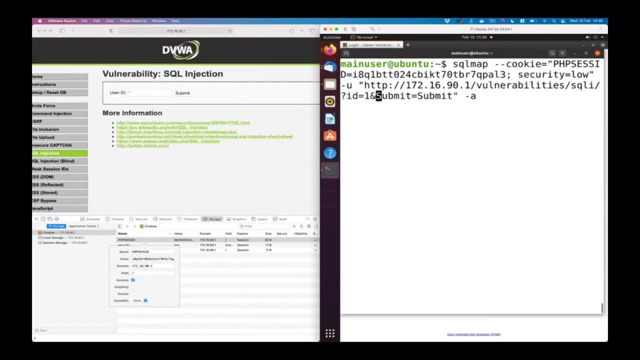 I've provided the URL, vulnerability, sqli, and an ID of one to get us started. The dash A which says please download a whole copy of the database. So this is pretty cool. It's actually going to try and steal all of the information from all of the users in the background. 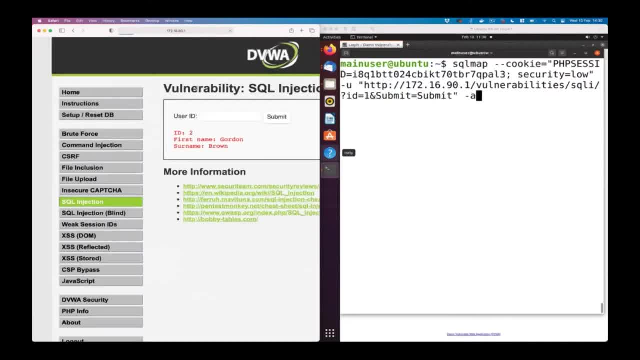 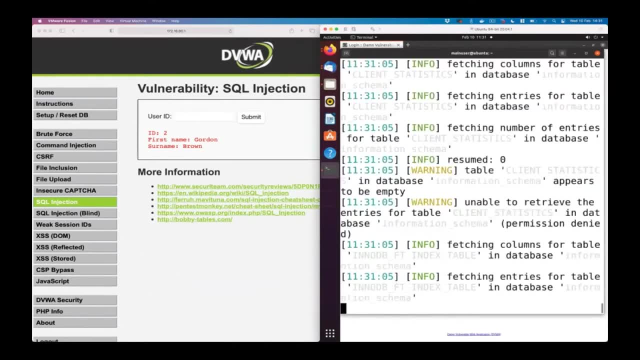 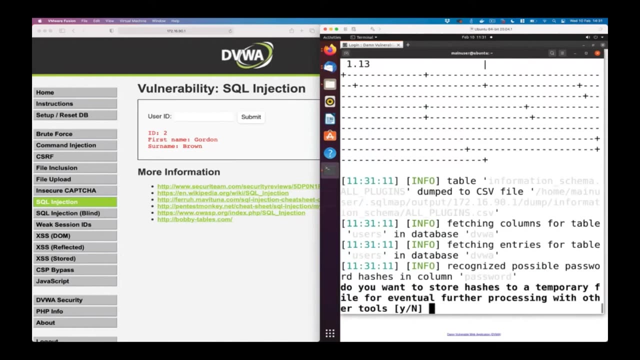 Way more than what we can get our hands on by just putting one or two. So let's run this command. Woof, Lots of information. Well, let me describe the process that's occurring here And also show you this a little bit slower. 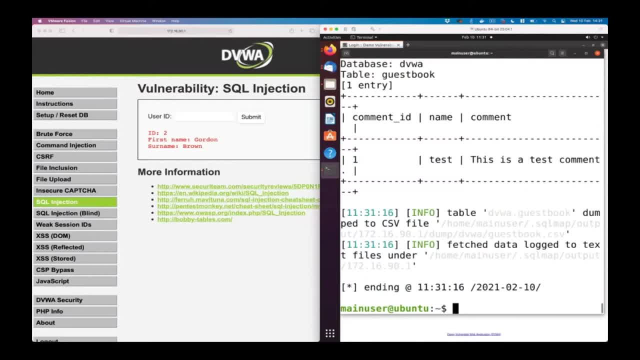 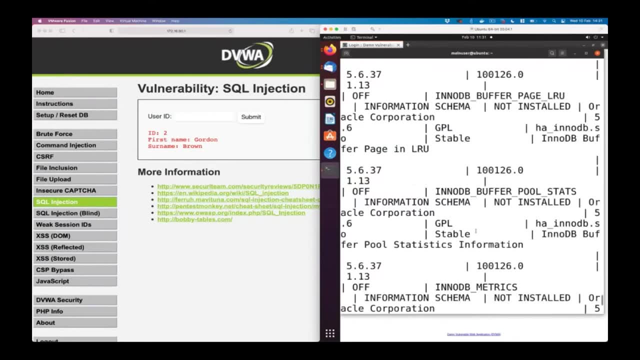 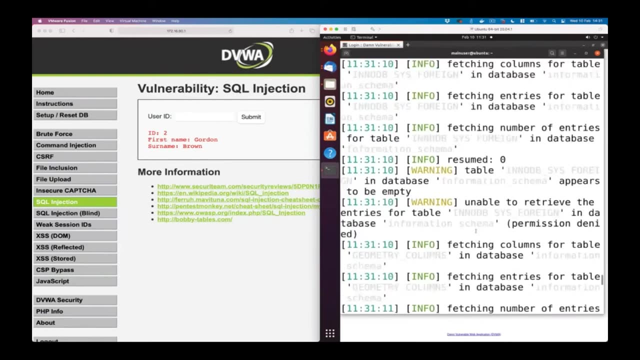 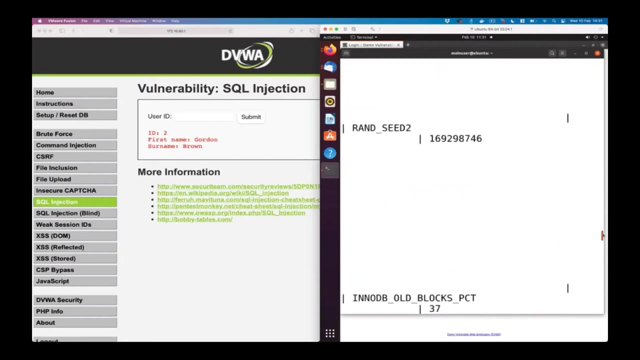 Let me save the results first. What's happened is it's found an injectable parameter. In other words, it's found that this ID is something that the user controls, And then it's constructed a series of thousands of very, very clever queries to be able to steal information from this database by manipulating it. 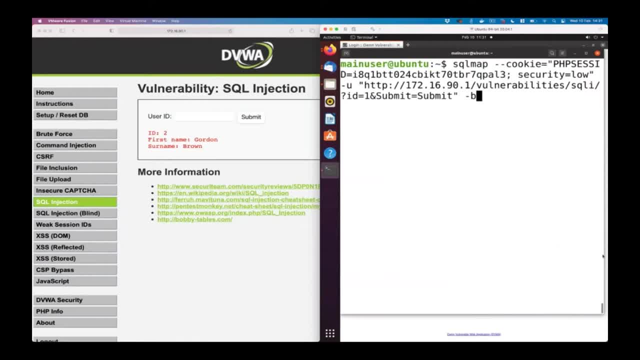 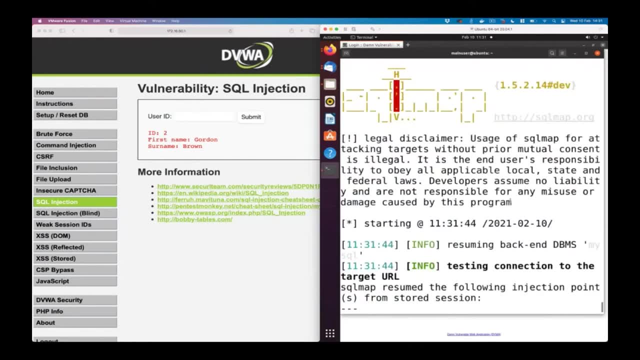 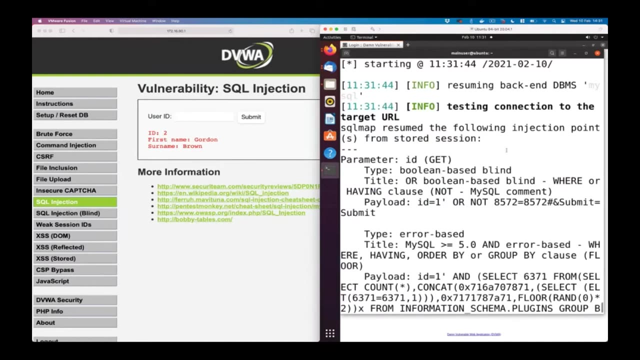 Let me run this again, but this time just with the dash B argument. That just shows us less information. Here we go. This is pretty complex stuff, but shows the power of tools Testing connection to the target URL. parameter is ID. It's selected a style of attack. 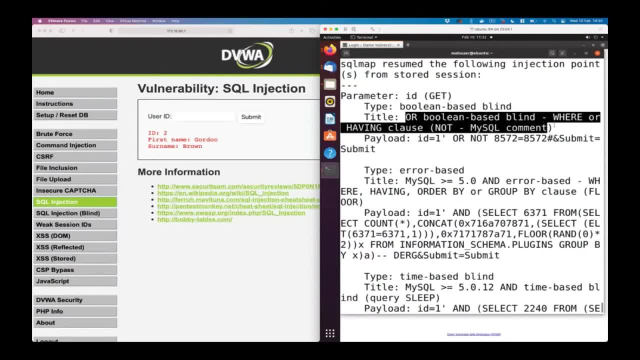 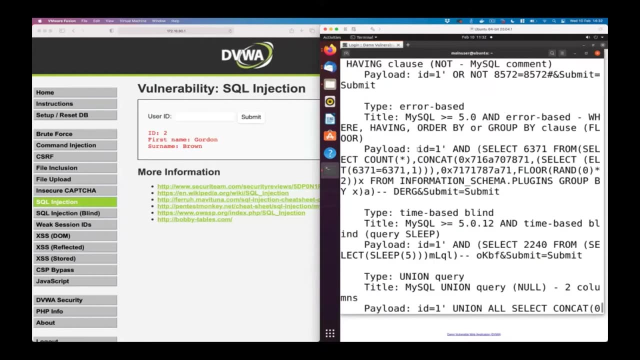 and it's using an or billion based blind where or having claws. That's not easy to say, but what it's really doing is exploring different ways It can trick this ID parameter and the database into giving us information, And these are actually complex SQL queries that it's running to try and extract data. 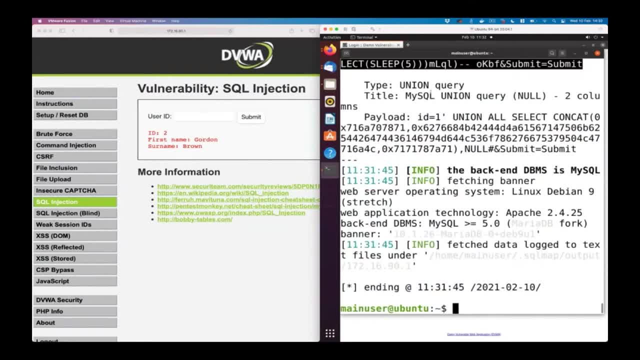 And we see here it has succeeded through running these various queries and identifying the back end Database is a MySQL data database and it's running on Linux system, on Apache, and extracted this information. So let me go To the location where it is stored, this data. 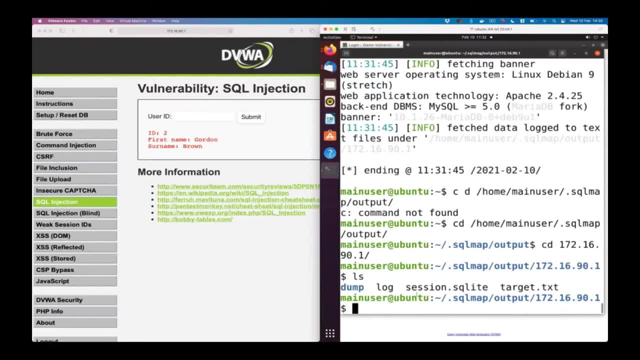 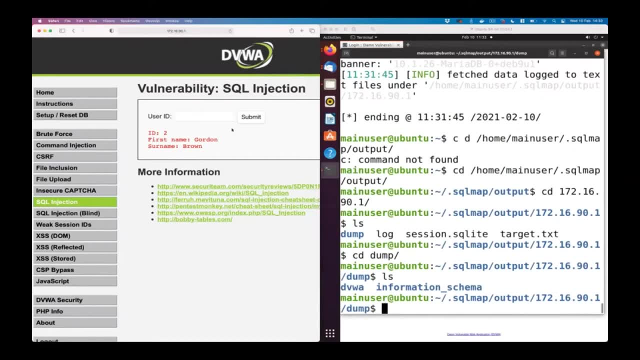 Here we go. We're going to log file that shows everything, but let's go into the dump folder. This is actually a copy of the data from the web server, And this is how these big data breaches happen when a floor like this is left open on a website. 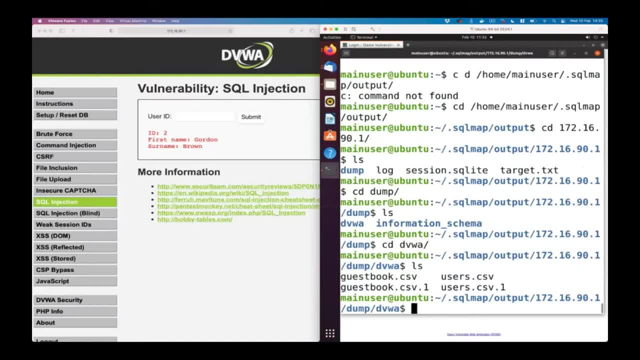 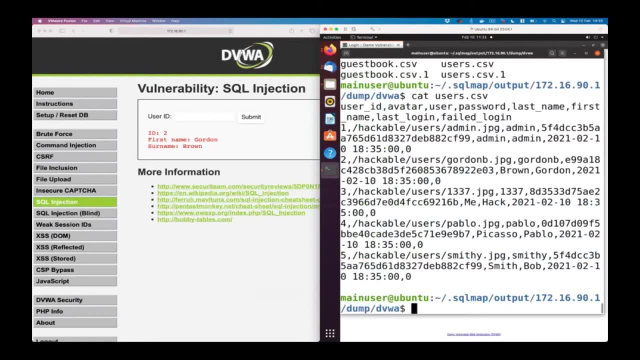 Hackers can use it to steal information from the database They shouldn't be able to access. So, for example, users dot CSV. This is a copy of all the information about the users. Remember this? admin, admin Brown Gordon. So let's go for three. 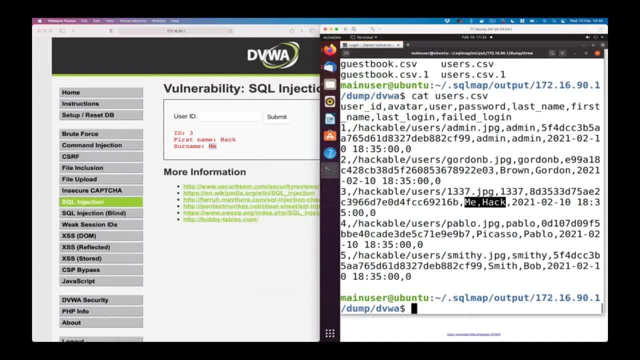 We see hack me, which is the user here, But we also see lots of extra information, such as what is very likely a password hash that we could try to break. We see information about their profile picture, So we're clearly getting access to way more information than we ought to by using this tool here. 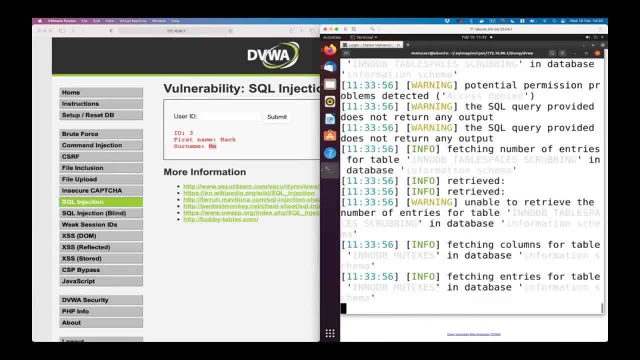 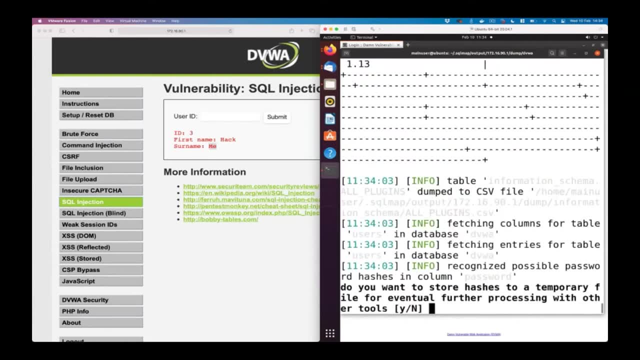 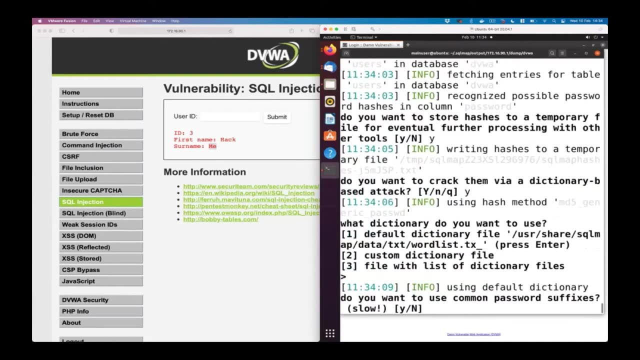 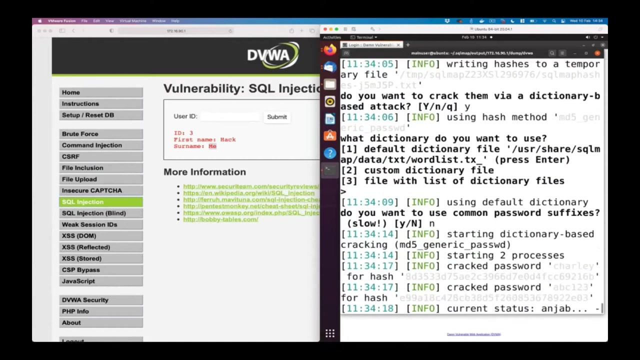 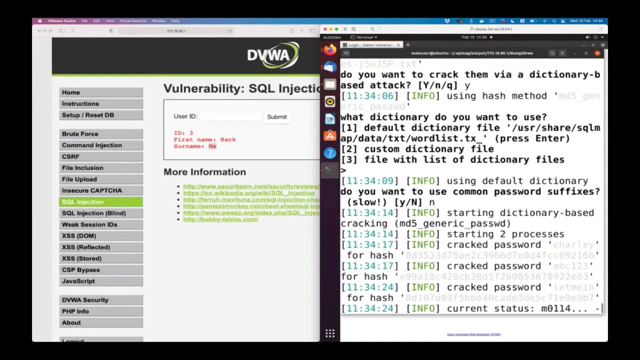 Run it one more time. I'll actually see if any of these passwords are easily retrievable in this particular instance. There we go. So this tool is even kicking off a. can I recover the password? And yes, the passwords unfortunately being used in this database are pretty bad. 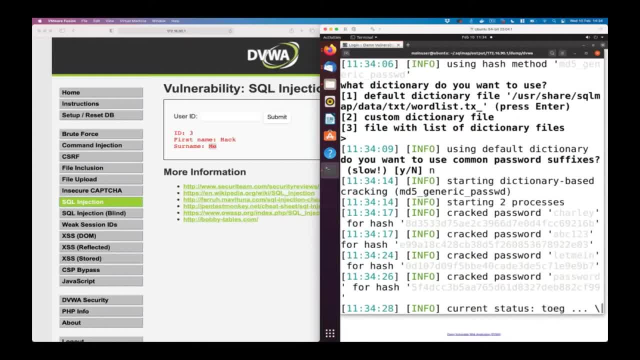 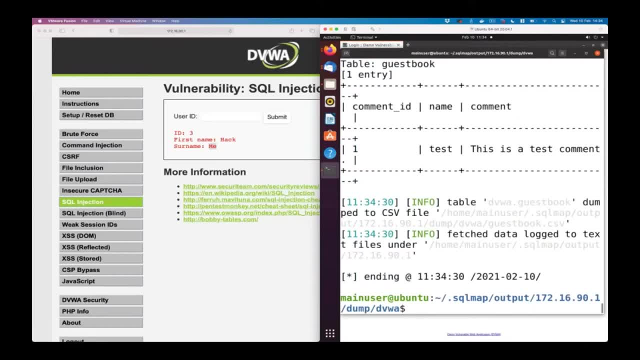 Let me in Charlie ABC 123 password and so on. So this shows you how a little mistake in providing users with the ability to submit information that then put into a query can be really dangerous. We could, with more time, manually execute this attack and form this query. 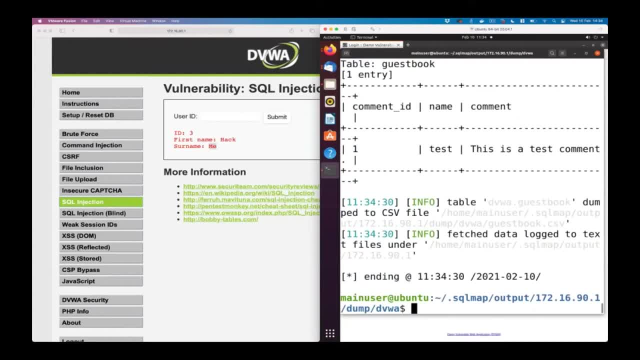 But this tool has automated the process of thousands of operations and given us access to many users data, much more information than we can get from the website. This could include credit card information, passwords or all kinds of sensitive data, depending on the application We were targeting. it shows you the power of sequel injection. 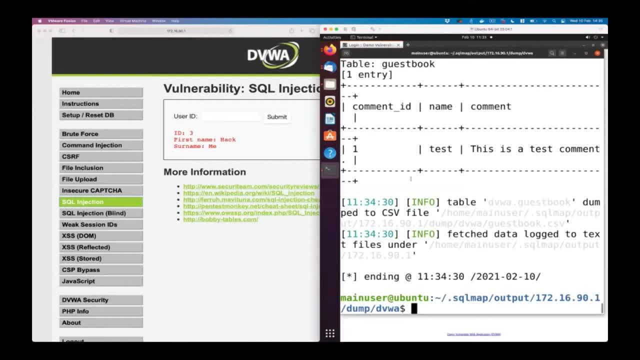 And, of course, there are multiple Levels of difficulty and escalations that can be applied here to and lots, lots more to learn about in the high levels of cyber start game and, of course, in further cyber security training. Now round out with one very important detail. 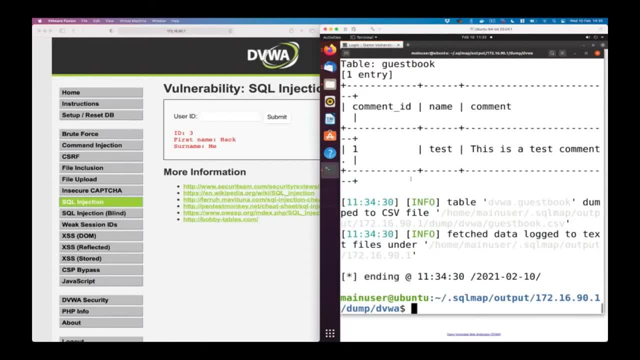 This is, of course, incredibly important stuff. by being able to understand these vulnerabilities, We can help developers write code that isn't vulnerable to leaking information like this on the internet. This also illustrates why it's really important to use Unique and secure web password per website. 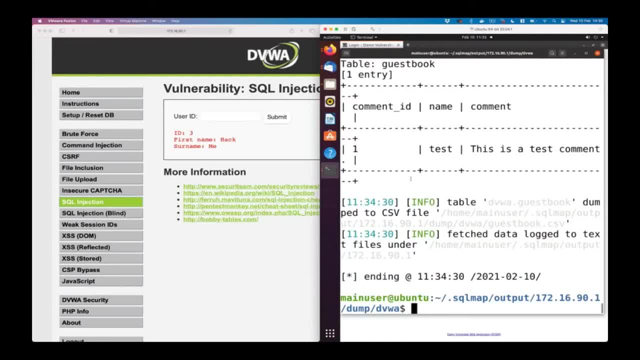 You visit. if you provide a password to a site like this and they have one of these floors, your password may be trivially recovered like this, And whilst that sites compromised, you want to make sure another website doesn't have the same password so that attackers can't reuse it site to site. 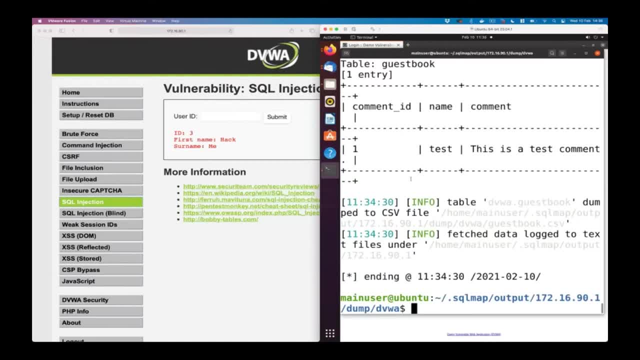 But most important of all, whilst learning this is incredibly fun and I recommend trying it in cyber start game Or even a mini lab like this on your own system, It is incredibly important to adhere to the code of ethics and, of course, to the law. 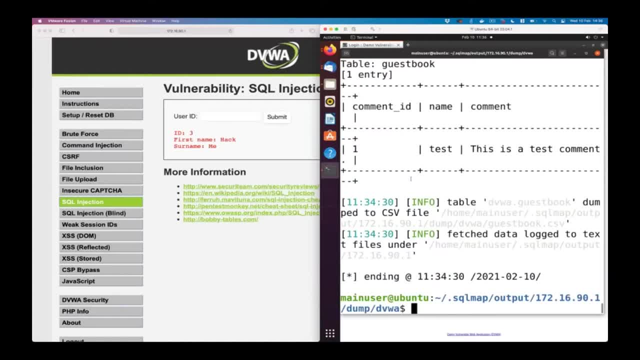 You can't go running these tools on random web pages on the internet without permission. Should you download data from the website because you find a floor, even if it's incredibly simple, even if it's something you can do just in a web browser like this command injection. 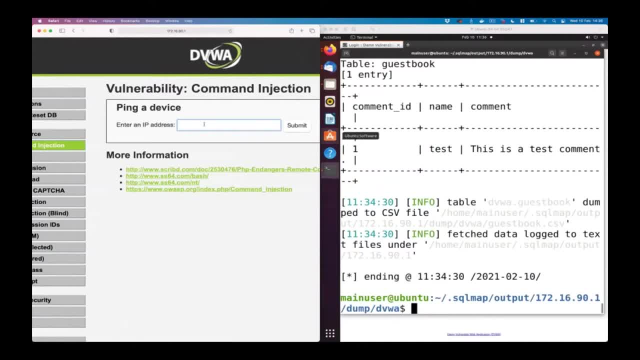 That is an abuse of the computer misuse Act in the UK, where I'm from, Or the computer Or the Abuse Act in the US. So it's very important- whilst this is fascinating and you can build a future career out of this stuff- to make sure that you're practicing safely in an environment where you have permission. 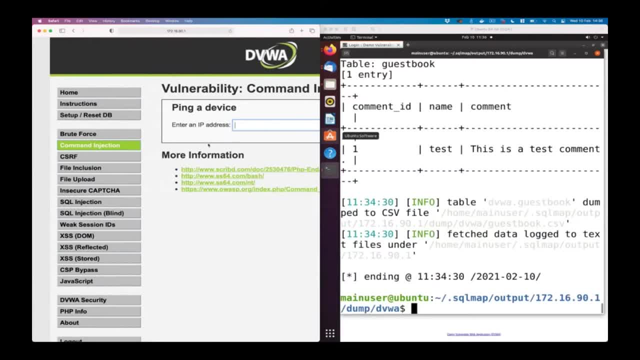 We're really just scratching the surface of fascinating web application floors here, and hopefully you've some idea now of what command injection means, session guessing and the power of SQL injection by being able to control and overwrite The intent of the developer with structured query language. 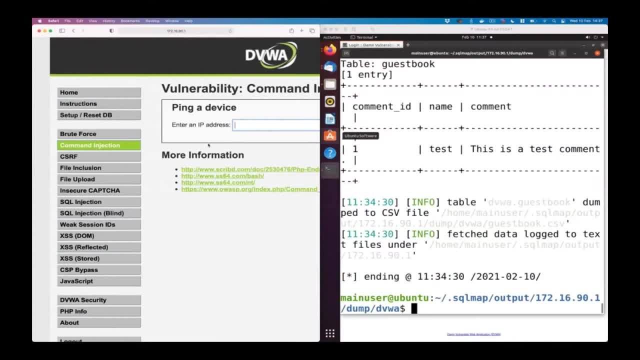 If you struggled with any aspect of this, remember you can learn more in game. you can find more online by researching. you can watch this video again. But most important, patience and practice. work through the more basic examples and in no time at all you'll be bypassing advanced SQL injection blind scenarios with filters. life really is hard for developers in writing secure code to provide resilient solutions. 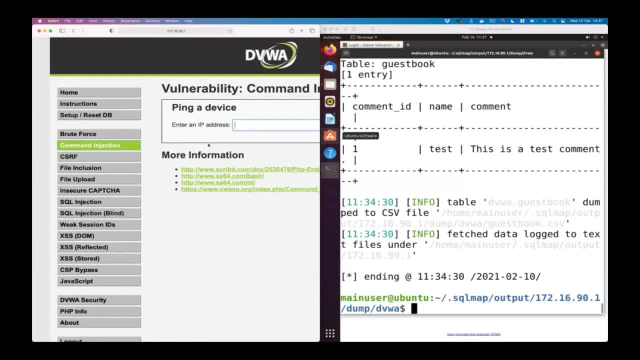 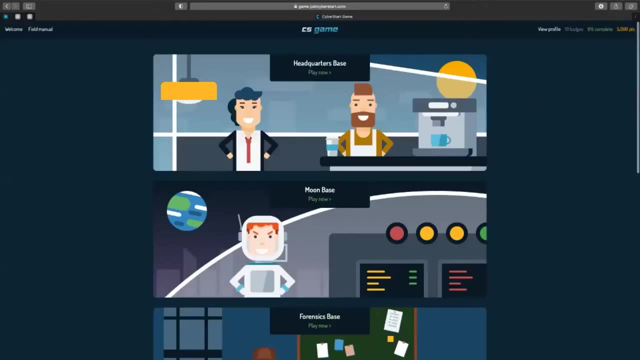 And this just shows you how much they have to think about and the richness of tools available to us as attackers. I hope you enjoyed this and over to Caitlin. Okay, Hi, everybody. I want to go ahead and jump off of everything that James just showed you. 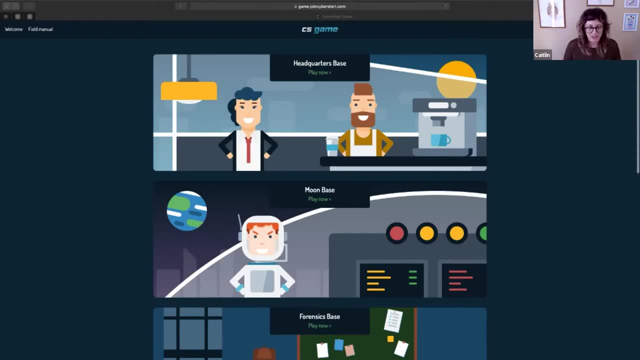 And I'm going to tie some of that stuff back into some of the challenges that you're going to come across in cyber cert game. Some of you may have already seen some of these. I'm going to the first one. I'm going to demo is going to be a little bit of that SQL injection. 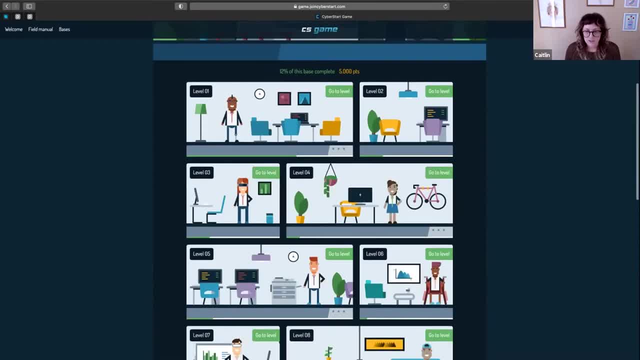 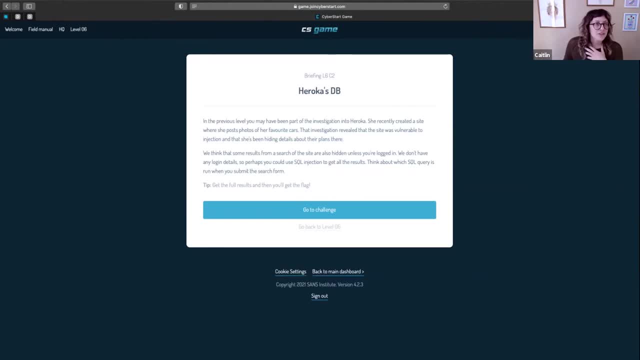 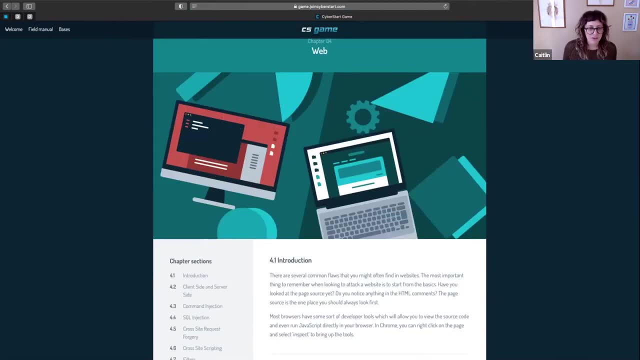 So the first challenge is going to be in level 6 and it's going to be challenged to. So the first thing to know obviously is all of this stuff You can look for in Under web. in your field manual There is command injection. 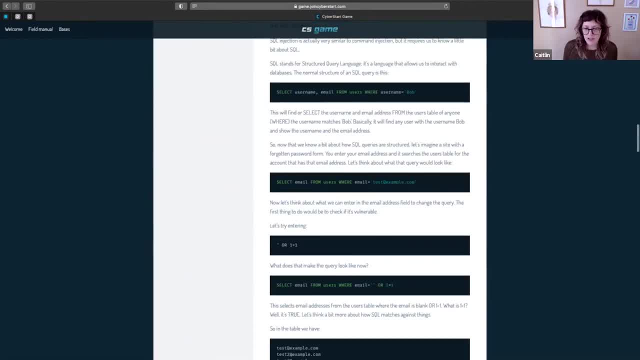 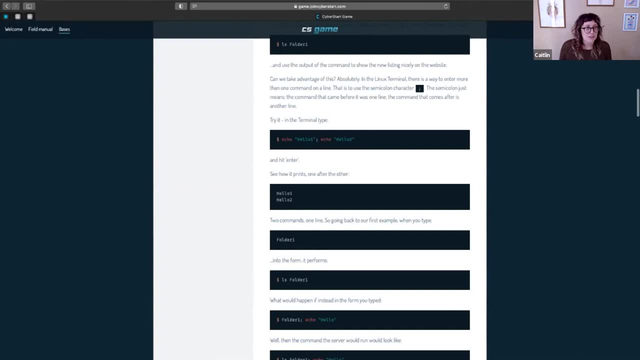 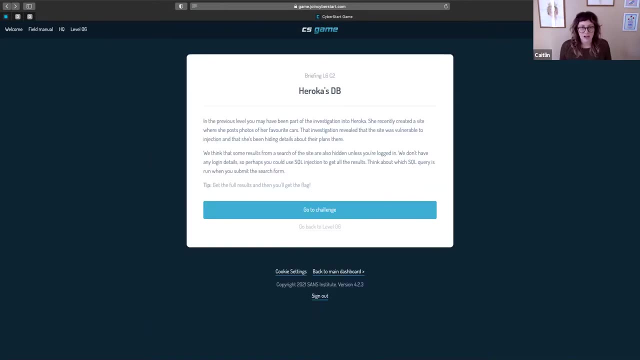 There's SQL injection. here You'll get some more examples, kind of see some usage of things that might be useful when you're trying to solve some of these challenges or exploit some of these vulnerabilities. Definitely a good thing to reference if you're having some trouble, if you're not remembering everything that we're throwing at you in this webinar. 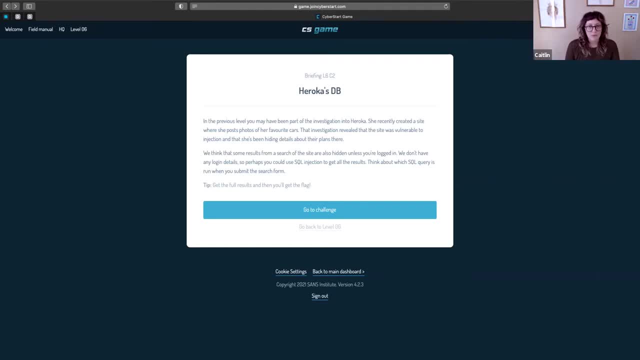 So the briefing for this challenge Is in the previous level and we're going to do that level next, So just keep that in mind. These will be pretty similar challenges. You may have been part of the investigation into Heroka. She recently created a site where she posts photos of her favorite cars. that investigation revealed that the site was vulnerable to injection and that she's been hiding details about their plans there. 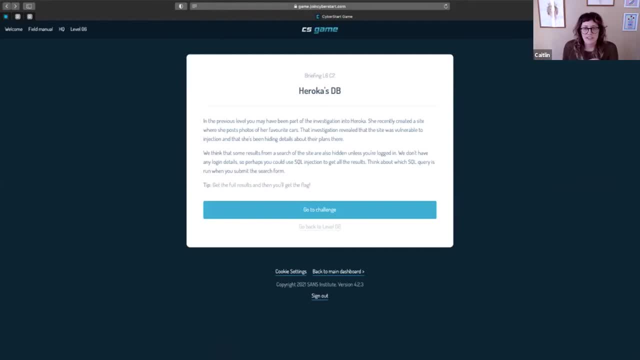 We think that some results from a search of the site are also hidden unless you're logged in. We don't have any login details, So perhaps you could use SQL injection to get all the results. Think about which SQL query is run when you submit the search form. 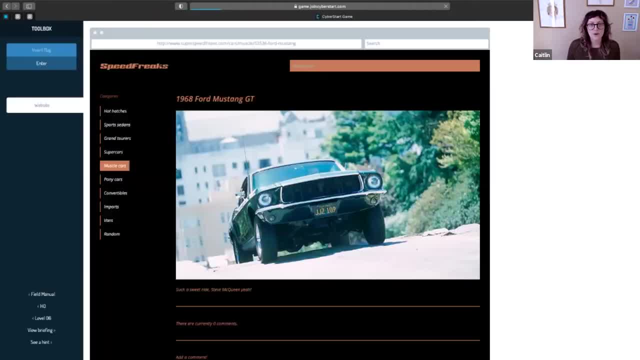 Okay, let's go to the challenge. So, whenever we search from this form, what they're wanting us to think about is the fact that this search is sending some request to a database on the back end and it's returning whatever results it might match with. 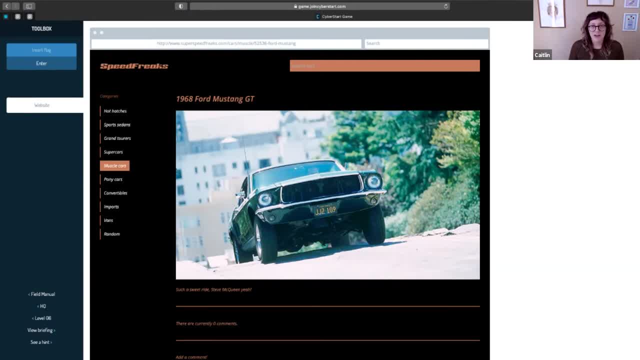 So it's really, really important to make sure that, if you're a developer and you're creating these websites, that this input is very is sanitized before it's sent in. Otherwise, you're able to do things like this and start sending back rather than just sanitized requests. 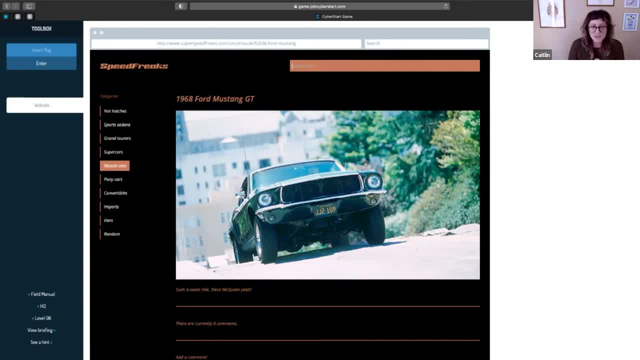 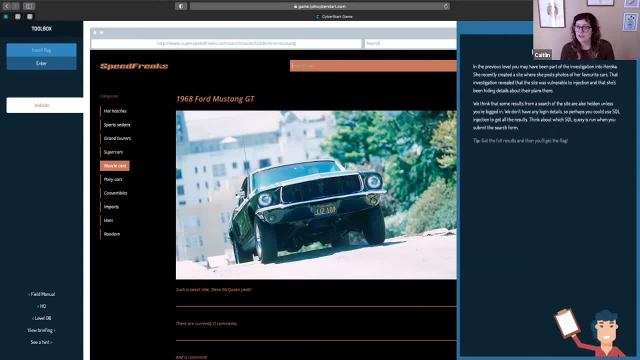 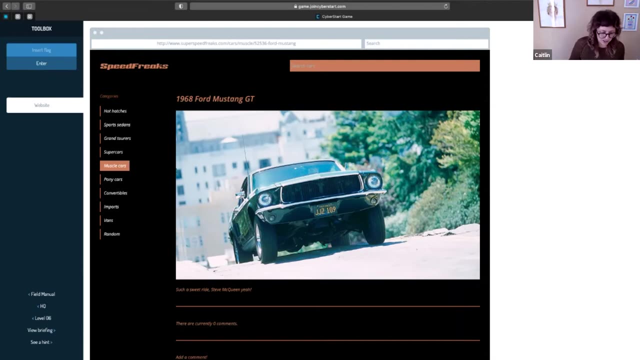 You can start sending back some actual SQL code, So I like to be able to look at the briefing whenever I'm doing this too. Okay, so we want to get the full results, So I would start any kind of like injection challenge with just something really basic that we've looked at. 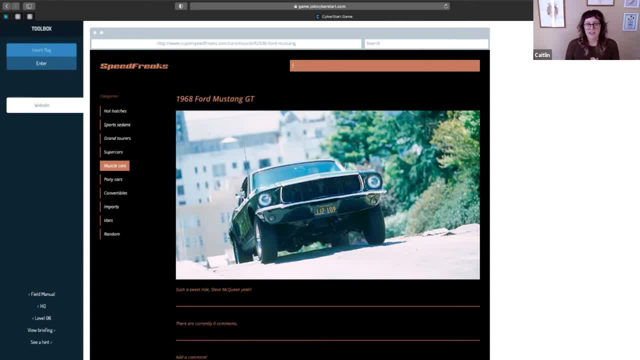 So we know that we need an escape character, right? So that's going to, that's basically going to jump us from sending some like string or some safe input back to that database to request it, And it's going to end the line and it's going to have us sending back actual code if the website is vulnerable to that type of thing. 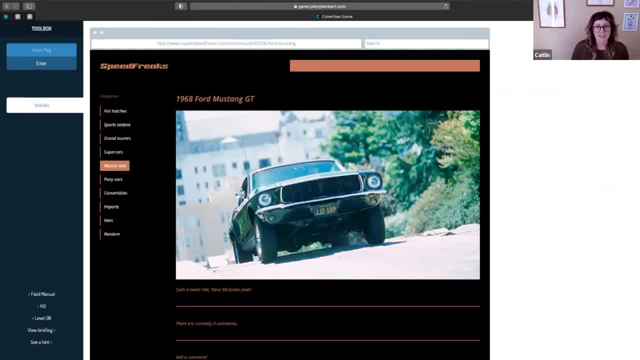 So we have Our escape character right there and let's go ahead and try that, This test to see If we can get something. when one equals one is always true. So basically what we're saying is: do this or do something, or if this thing- that's always true- is true. 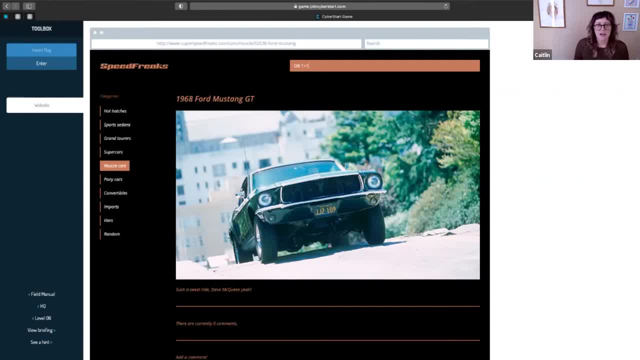 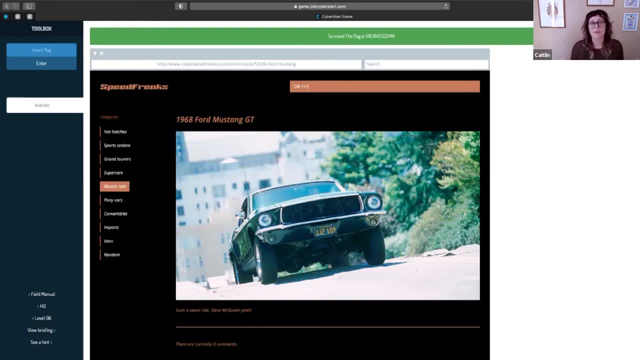 Give us back everything that we're requesting. Let's see. Okay, That was successful. We were able to talk to the actual database and send it data like SQL code, And now we've gotten this flag right. So that one was was much simpler than the stuff that James was doing. 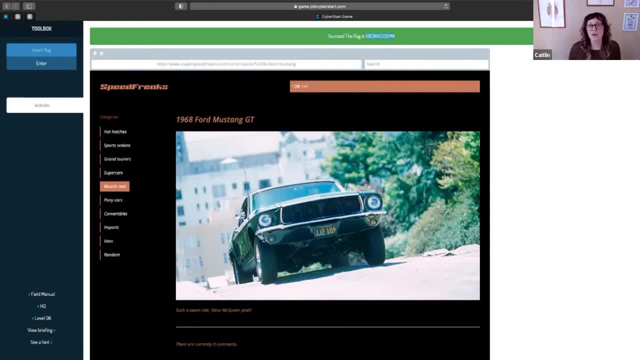 But a great example of how you would use that and how you would also test just to see if a website is a vulnerable to that, is these kind of simple SQL commands and then you can build on them further if you're able to get like a list of what the tables are named or a list of different fields in those tables. 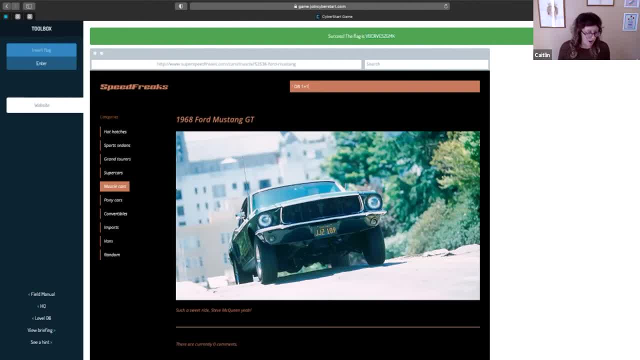 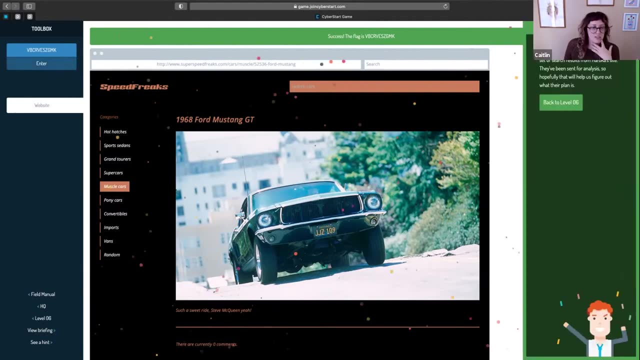 You can start asking for really specific stuff So it can be really really powerful and really really dangerous. If this stuff is not, is not well protected, Okay, so let's go ahead and get our confetti here. Great. The other challenge that I wanted to walk through with you, another kind of a quick one, but it'll be. 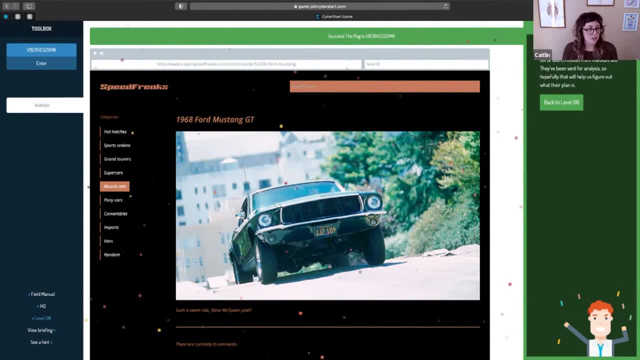 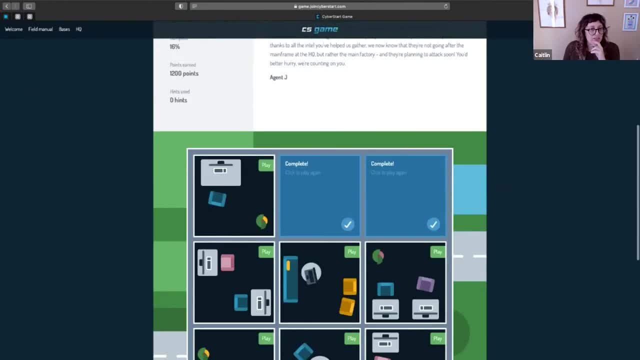 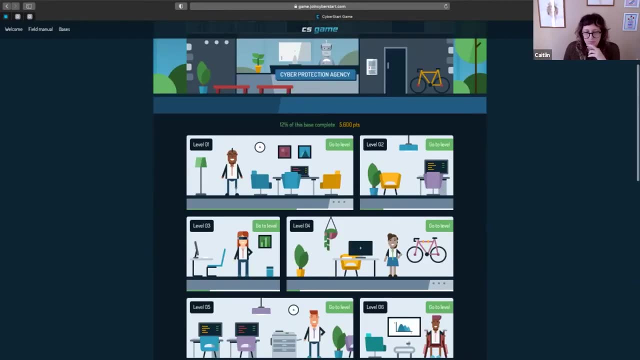 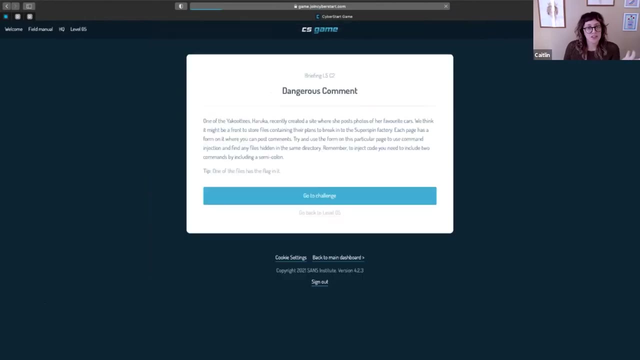 a command injection challenge which, again, you just saw James demo some more advanced versions of- is going to be in level five, So let's jump back to HQ. Okay, and this is going to be level five. challenge two, and it's going to be: 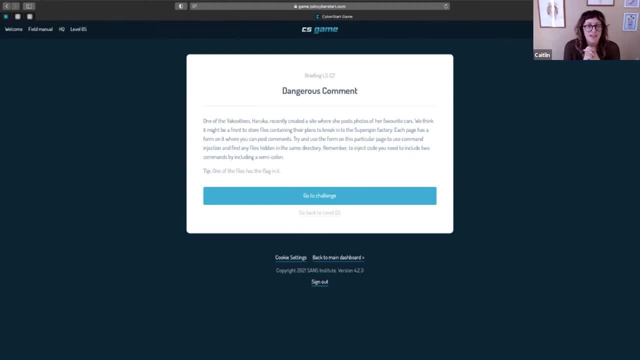 pretty similar as far as the way that this website looks. So one of the Yakutis, Haruka, recently created a site where she posts photos of her favorite cars, which we just saw. We think it might be a front to store files containing their plans to break into the super spin factory. 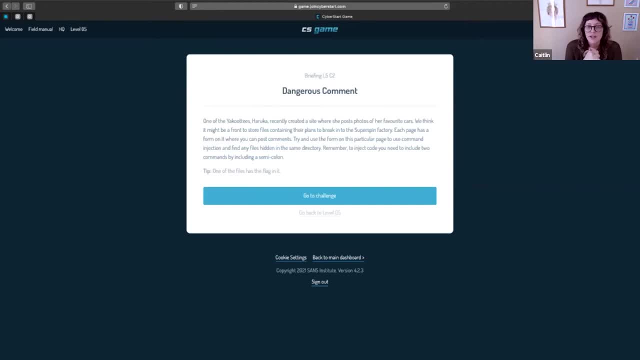 Each page has a form on it where you can post comments. Try and use the form on this particular page to use command injection and find any files hidden in the same directory. Directory- remember to inject code You need to include two commands by including a semicolon. 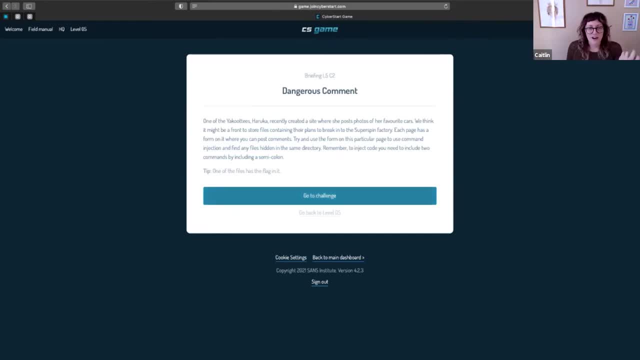 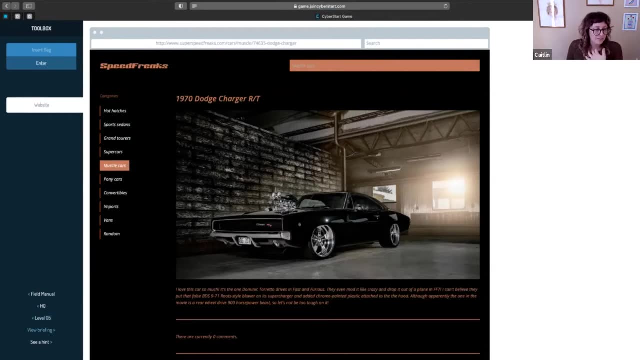 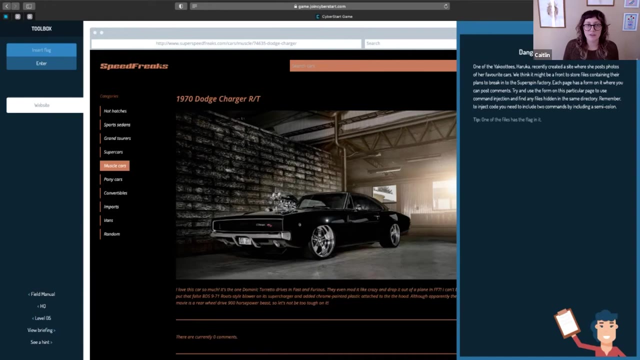 Okay. so we need to try and figure out How to find this file and read this file that has some you know, some code for us or some flag. So same side this time, instead of using the search input field to do a sequel injection to send some info back to that database. 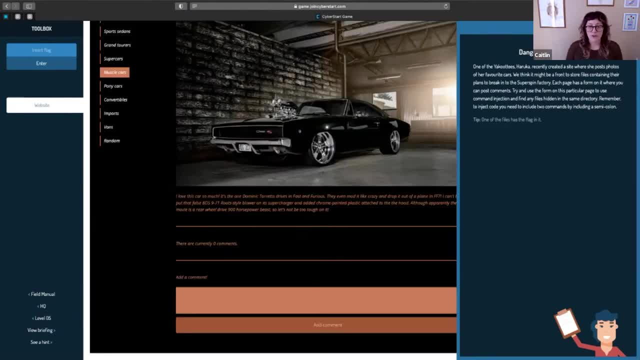 We're going to go to the comments and we're going to try and run code directly from some kind of shell. So the way that we want to Test this, we are assuming that there's some kind of code running in the back end And we're going to throw a semicolon in and this will tell us again if there's any kind of vulnerability. we should get some sort of input back. 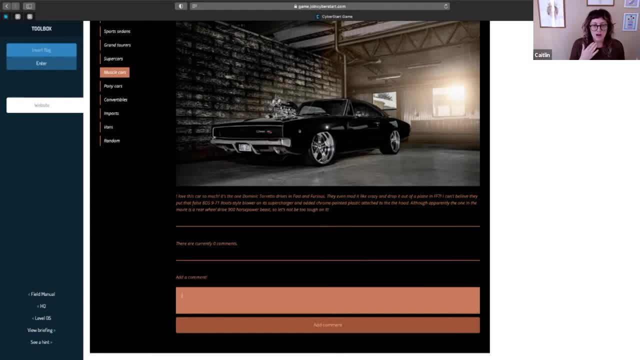 So let's just a command that we know very well from doing all of our command lines interface challenges, and let's just see if we can get a listing of Where we are and all of the possible files or other directories in the our current working Directory. 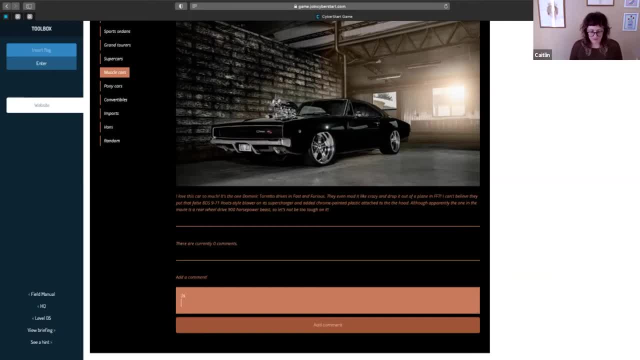 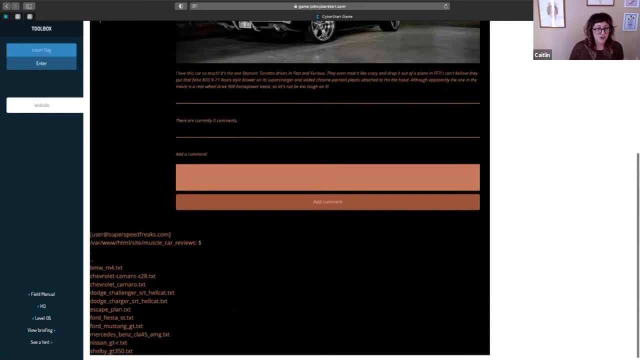 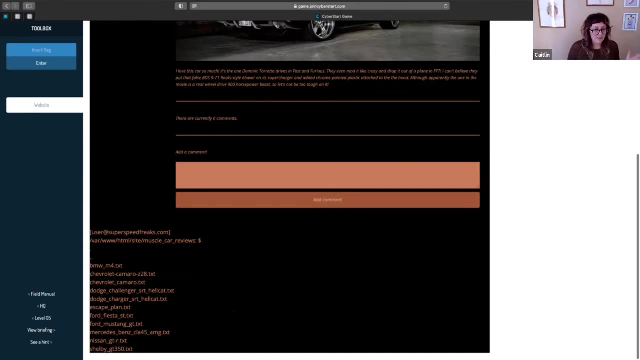 So let's use LS, that old favorite, And let's go ahead and See what that gets us. Okay, great. So now we know for sure that this website is vulnerable to these command injection attacks, And we've gotten a list of all of the files that are in this current directory that we are in. 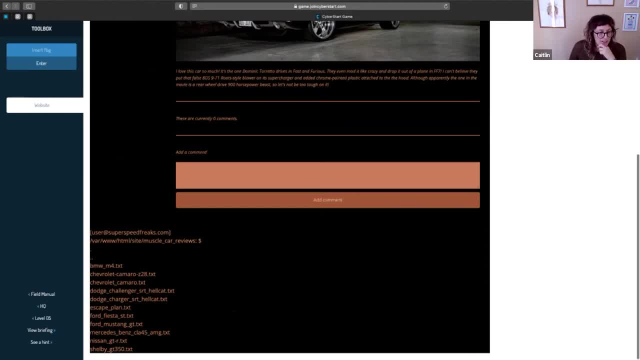 So these all are look fairly normal Until you get these are all cars, right. They're all different, Different kinds of cars, except for this. looks fairly suspicious right here, This escape underscore: plan dot txt, very conveniently named right. so Let's go ahead and try another command that we know. we know that if we want to view these readable text string characters in a file, we can use cat and go ahead and get just a readout of that file, of those file content. So let's try cat. 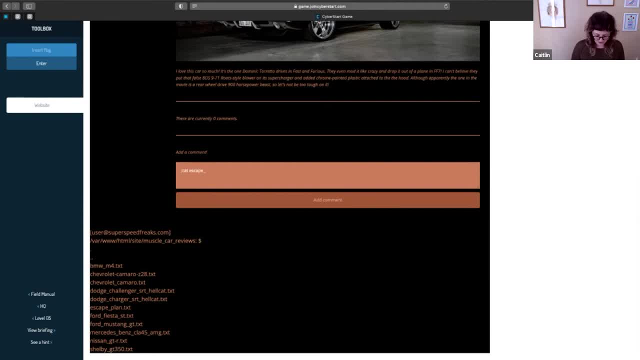 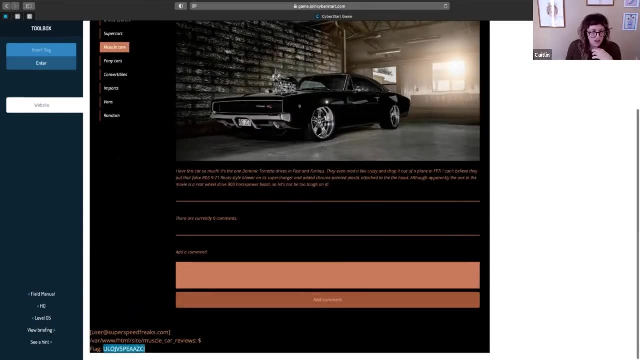 And then it's Score: Okay, great. So that worked for us. So we were able to again Run commands like if we were in a terminal on the back end of this website, which is great. You can probably also think of ways where this would be super dangerous if you're able to kind of 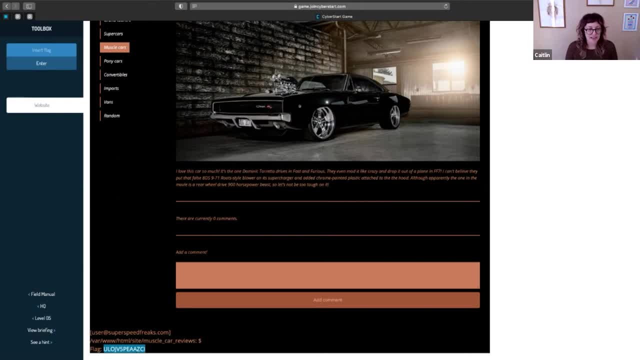 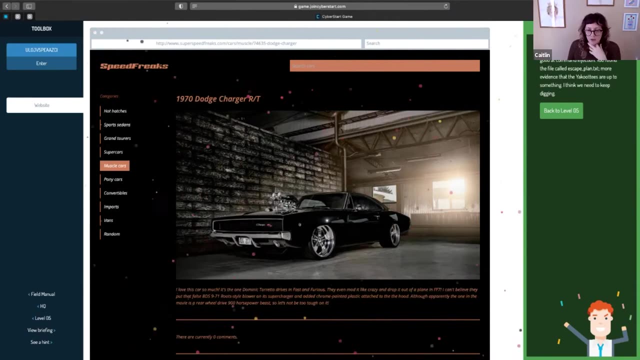 Navigate around the, The back end of a website and see and execute commands- Obviously very, very bad stuff. So again, let's get that Great. So that's kind of those are the two challenges that I wanted to show you that I thought went really well with what? 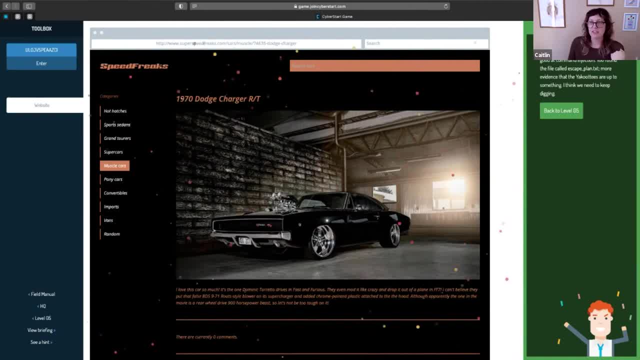 With what James was telling you about and could tie that back into game for you. And the thing I want to add is to what James said is: is these kinds of web application Vulnerabilities, especially these injection attacks, are so, so important. 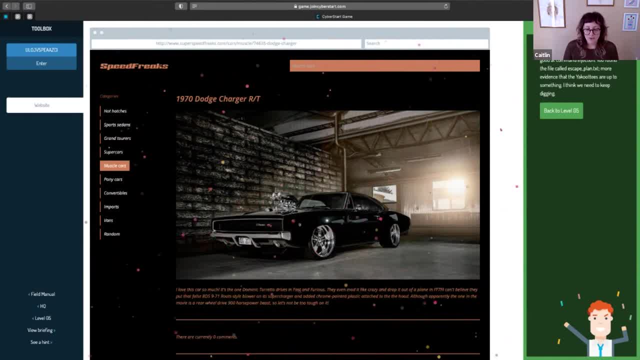 It makes it so important to make sure that, if you are a developer, or if you're trying to check for secure code, that your input is always sanitized, that you don't let anything come through that could possibly escape your code and make anything Like this possible. and these kinds of- And these are one of the most common even today. you might think, well, this is silly Like nobody knows. 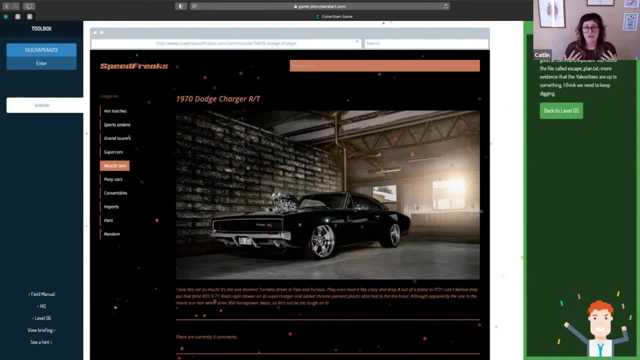 Nobody knows, Nobody does this anymore, But even today there are so many, so many vulnerabilities that are uncovered, which is these kinds of basic Checks. So you know a lot of the big breaches You've heard about in the news where- or SQL injection, target Equifax, Sony, Yahoo, those, all those huge breaches. 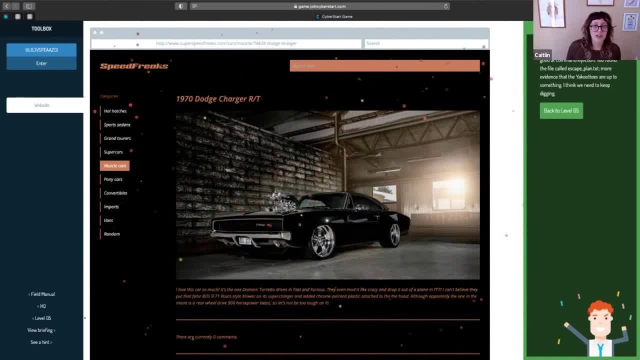 The attackers got in because they were using SQL injection, command injection, And I think I can probably jump off. Let me see, I'm going to stop sharing my screen and we can maybe do some Q AMP A stuff If we've got some questions. 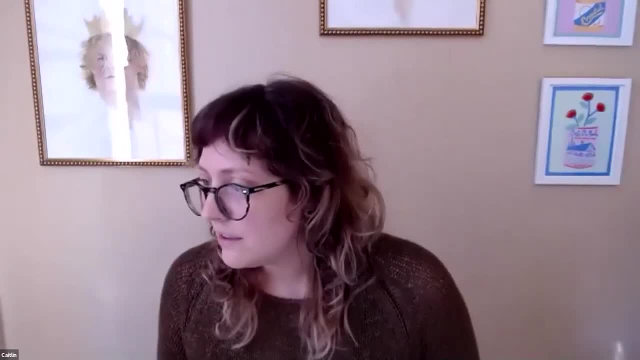 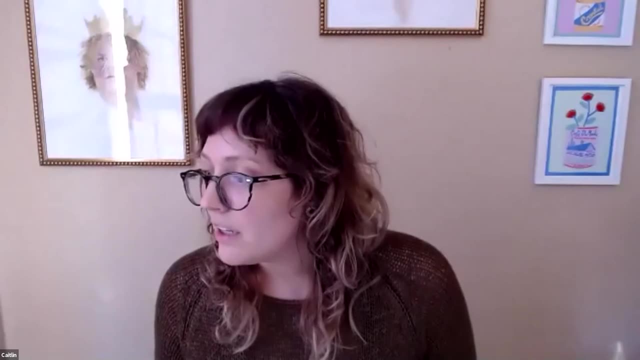 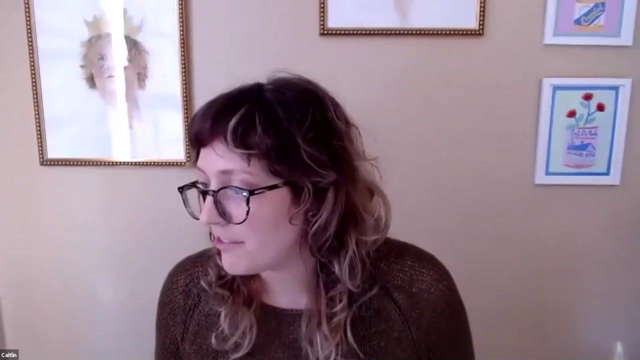 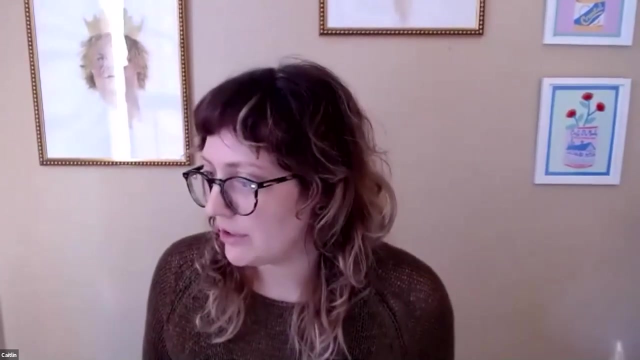 Let's see, I do see this so that the DWA website- you can use it in the US. that's, you're going to clone that from a git repository So even though it has UK at the end of that, You absolutely are able to use that in the US, See. 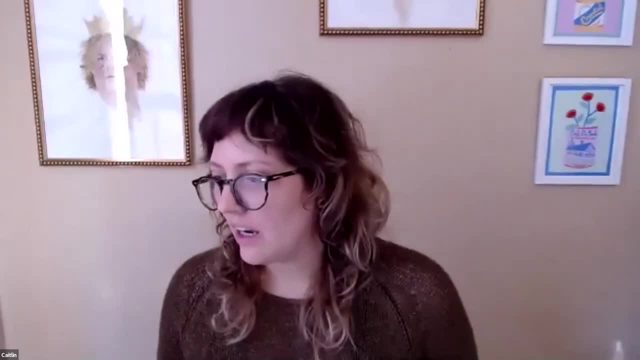 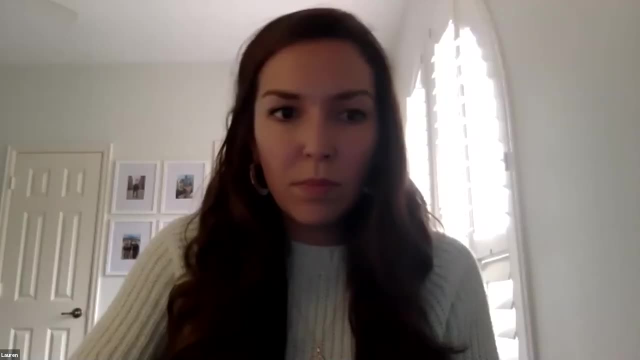 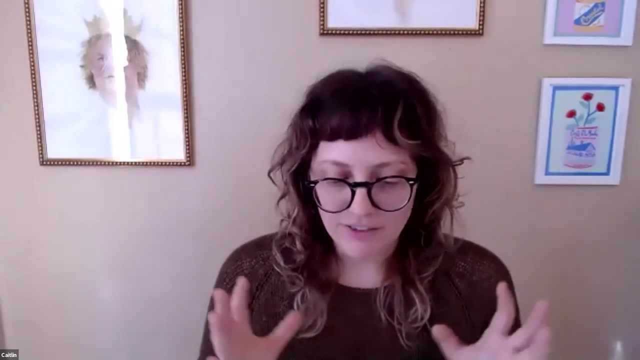 Okay again. so this is a great question. And why do we need that posture fee? So what that does is, in sequel, whenever you use an apostrophe, What it's doing is it's exit. It's called an exit character And what that's doing is it's exiting from any kind of 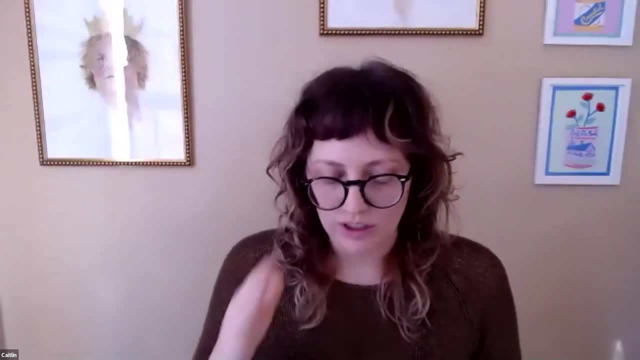 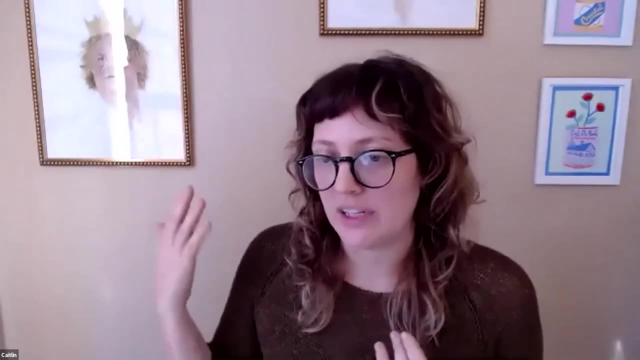 When it sees that it doesn't Think that it's just a string or just something. but I'm what it will do is it sees that and it knows to exit whatever it's doing and return to executing SQL code. So if you use an exit character like that or escape character, 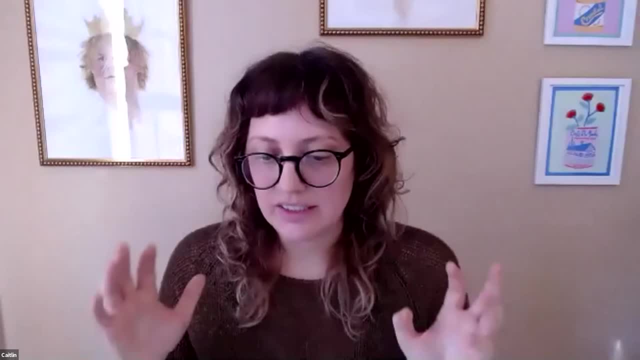 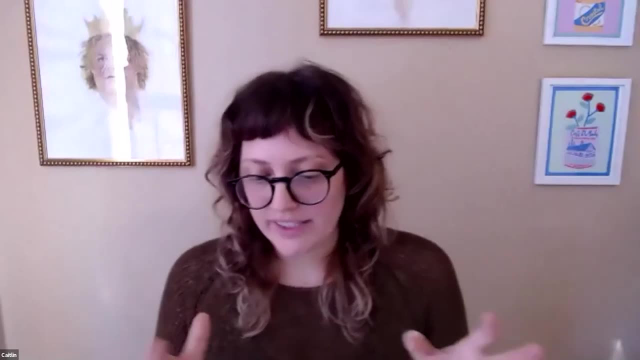 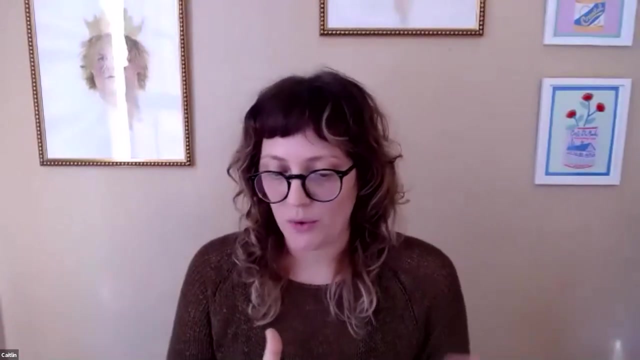 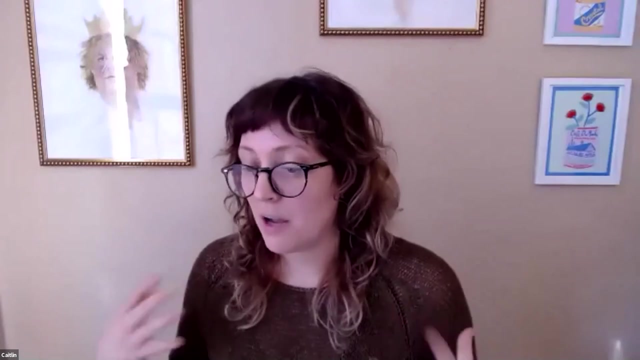 You are able to then start typing in actual code. So you could have typed in Some search request and then a, An apostrophe and then some code, And what it would do is it would search for that search request and then everything after that apostrophe. It's going to execute like you have been. you're giving that sequel database a command. so 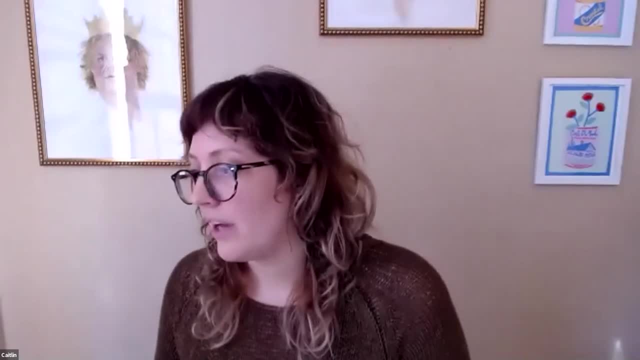 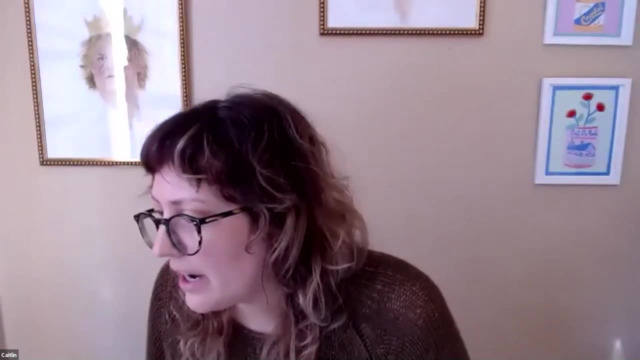 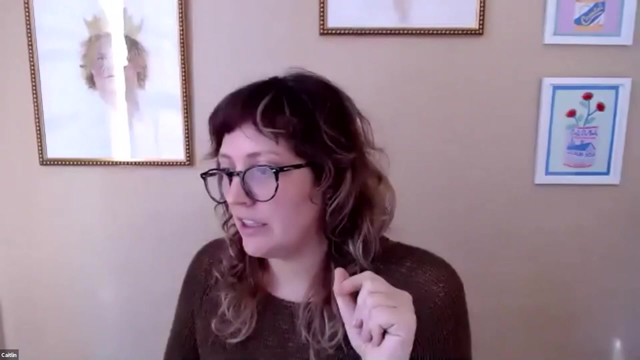 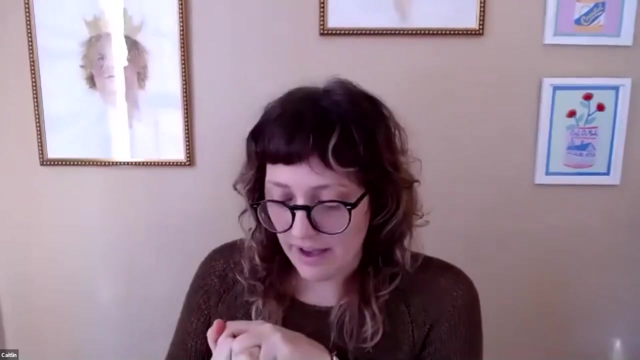 It's. that's where those characters come in- and a first sequel. That's often that apostrophe. I'm not sure what the Blurry text was about, but I've given you a little Clues. if you want to go back and do these challenges, you should be able to just kind of follow along with what I did and look at the field manual and figure out what to type in there. It's all. it's all there. so 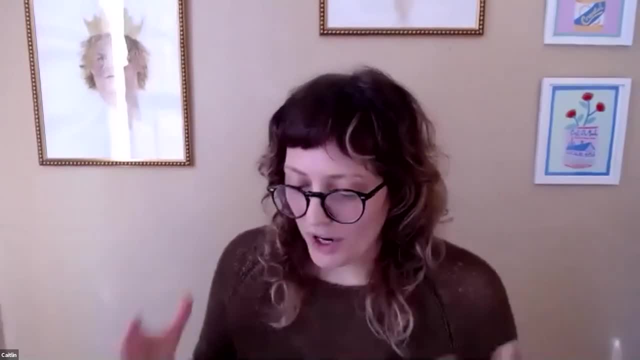 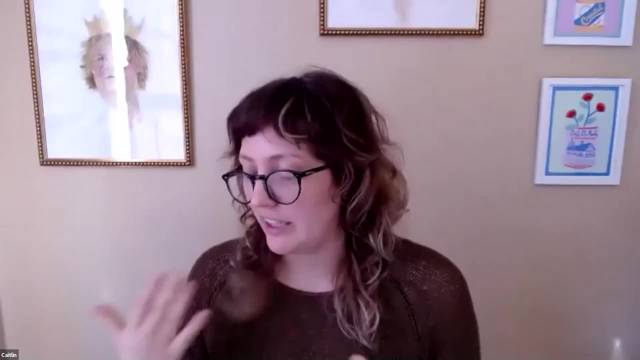 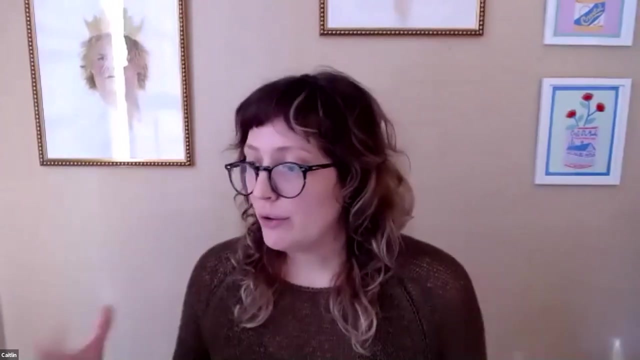 As far as a shell. A shell is what you're running. basically, what a shell is helping you do is it's giving you this really nice interface for you to be able to more directly talk to your machine. So in Windows that's going to be, or Linux that's going to be, your terminal you're probably used to. if you started game. you're used to seeing a lot of command line stuff in HQ. 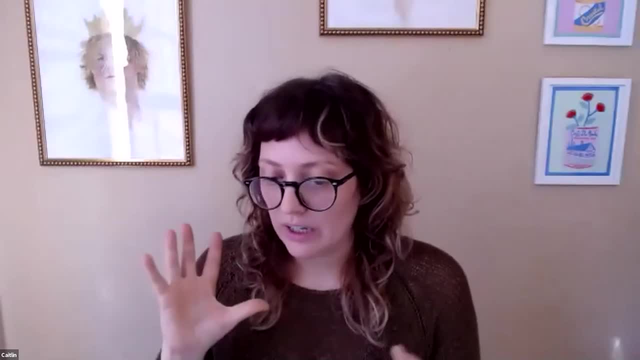 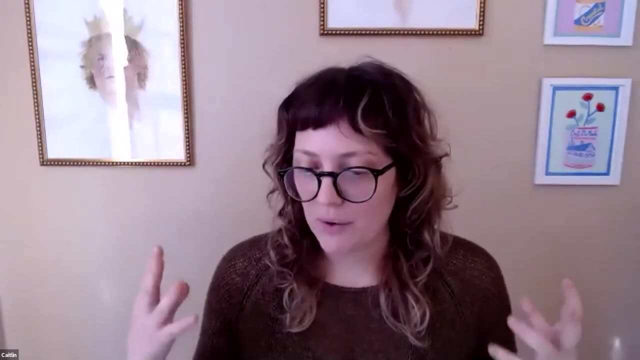 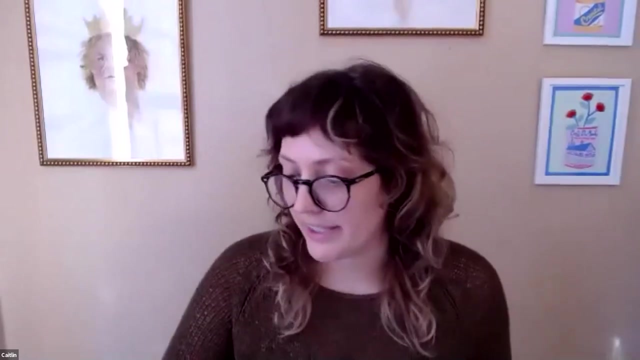 Your. that's where you would type in things like LS or cat or, you know, CD to change directories. it's going to help. It's basically a place where you can navigate around your system and tell your system more directly to do things. that allows you to communicate with your computer very closely. 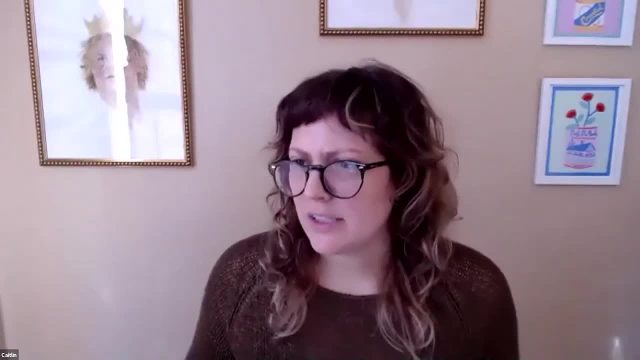 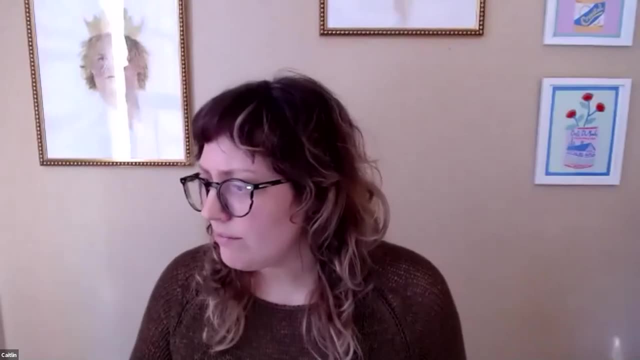 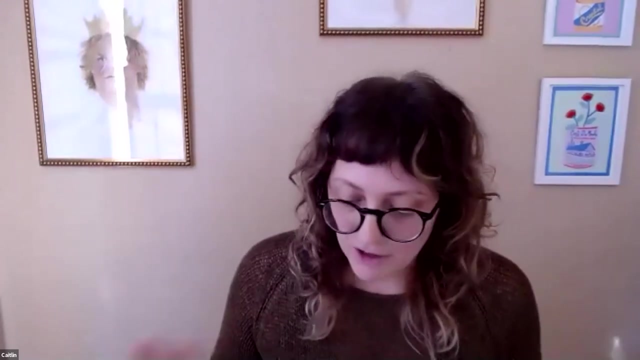 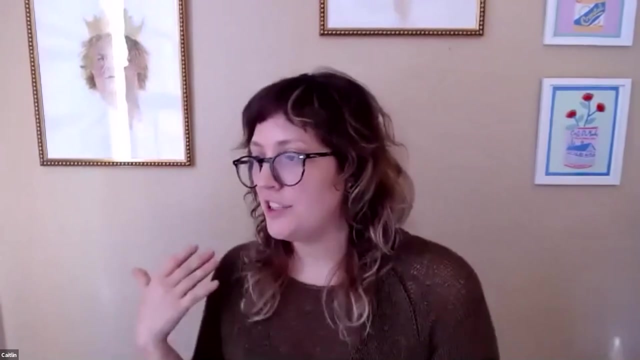 In Windows I want to say there's this: I know there's PowerShell and I forget what the more basic Windows shell is called. Okay, so, as far as basis for the competition, I would say everybody should start with HQ base right, because that is a really nice intro into how the challenges work. 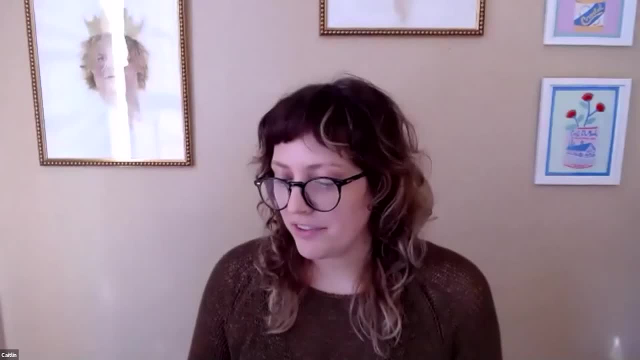 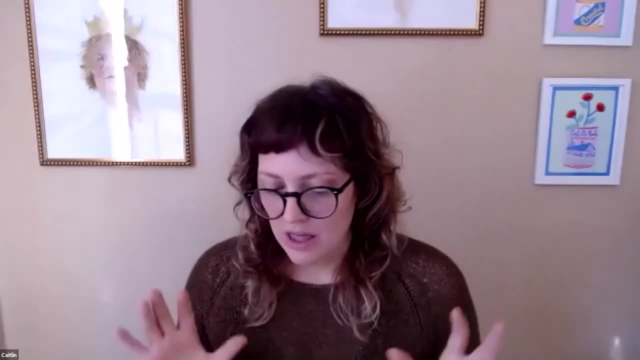 How you're going to find flags and input flags And it really gets you warmed up and kind of like going in game as a platform. The moon based challenges are all going to be Python, So they're going to introduce you to a little bit of Python coding. 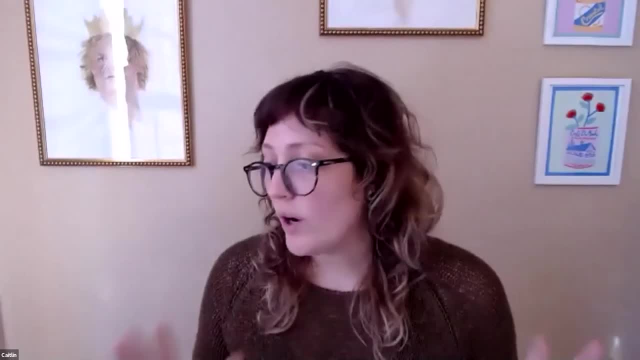 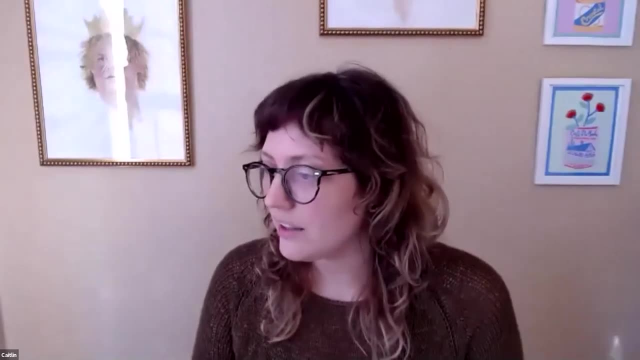 And again they're going to go slow and they're going to get harder. So if you wanted to start there with a little bit of coding, You can do that too. I would still probably recommend starting with HQ, just because it's A little bit. 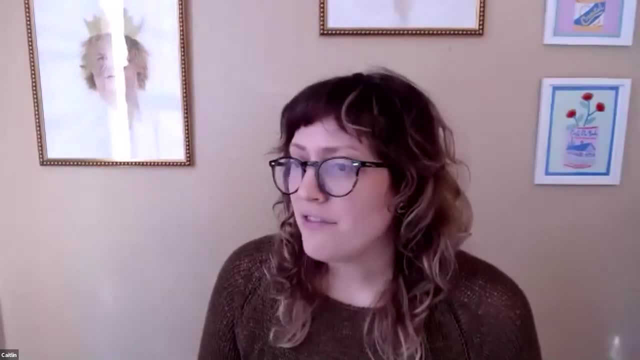 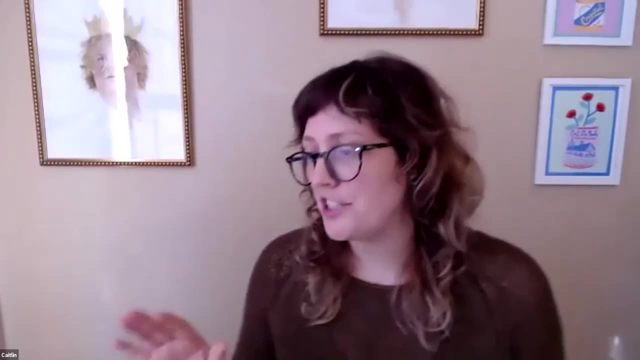 I think it's a little bit more of a of an intro, and then forensics is is once you've already got your code, You've gotten the hang of some of the other stuff, And once you already have your virtual machine downloaded and stuff, That's when you can do forensics. forensics is one of the more advanced spaces. 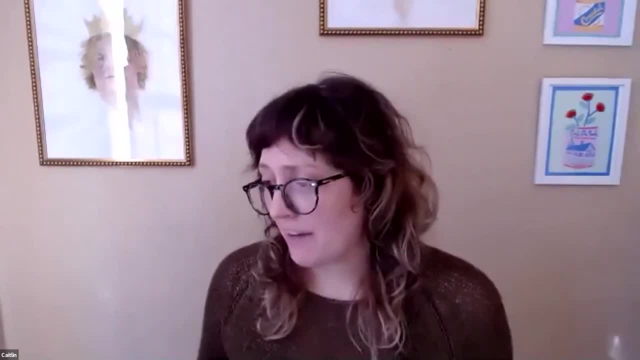 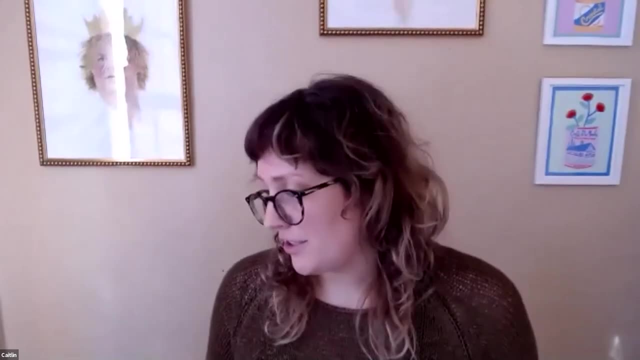 You're going to go right into a virtual machine there with moon base. you'll never have to use a virtual machine with that Python base. with HQ. You don't have to worry about the VM until like level six or seven. So that's why I would start with one of those two bases, because the forensic stuff is a little bit more. 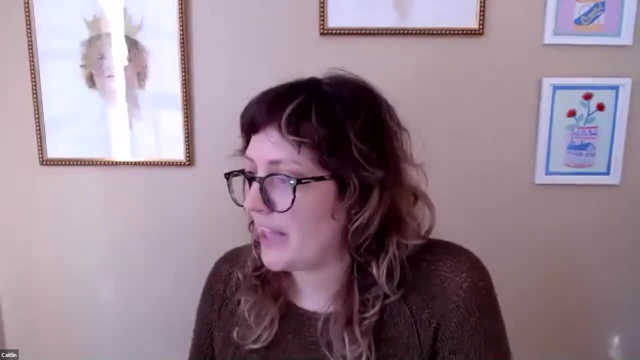 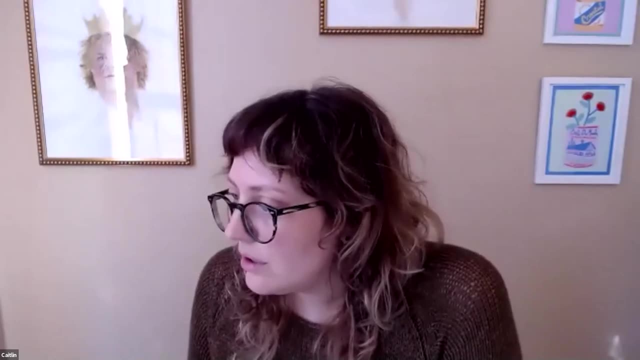 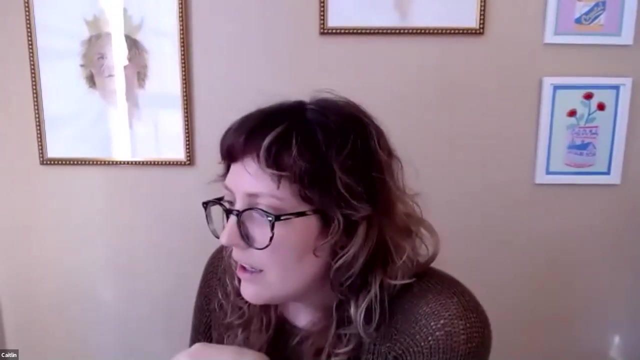 Advanced, although I think there's a little bit of Steganography at the very beginning That you can do without the VM. Okay, What else can I answer here? Okay, so I'm seeing this is a really good question about types of careers in cybersecurity. 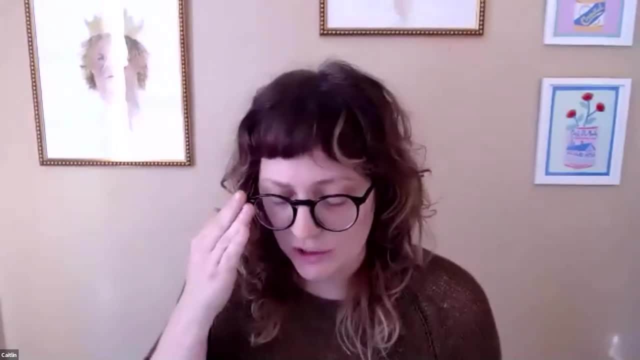 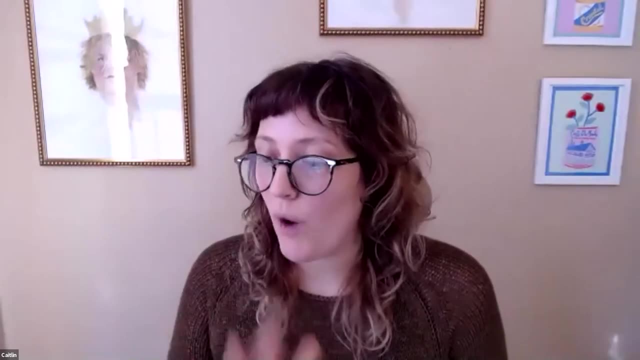 So one of the types of careers that we can kind of tie into from when we talked about today is web application security. So from that end you can do things like be a web app penetration tester, So you can get hired by companies to go in and try to find these. 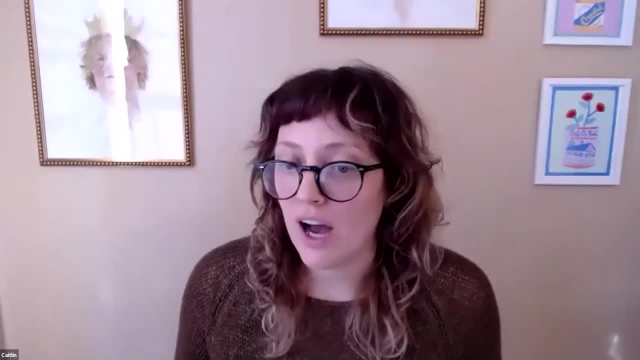 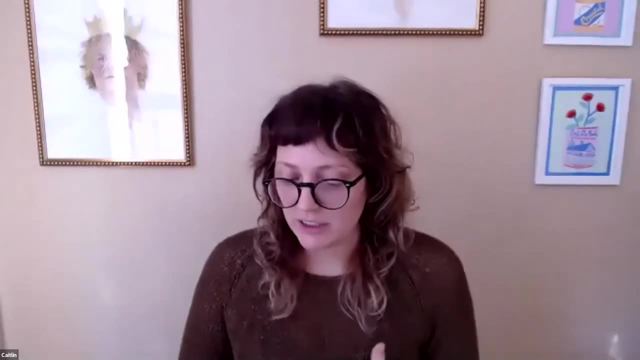 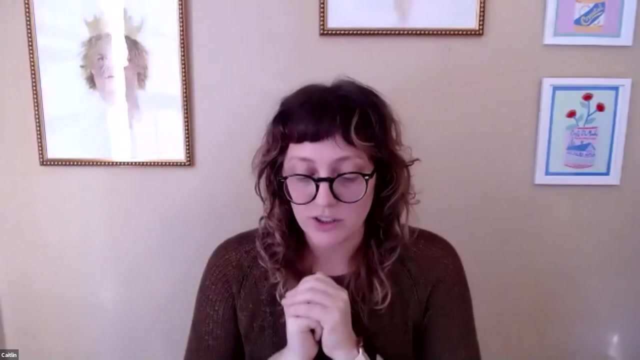 Application flaws and they'll pay you basically to exploit their vulnerabilities and then they can go in and fix them before attackers can actually find them. That's very similar to things that you would do if you were doing bug bounties, which is basically you're kind of like an independent contractor for a web app penetration testing. 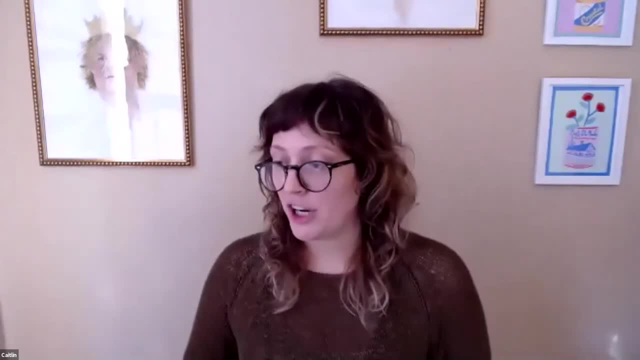 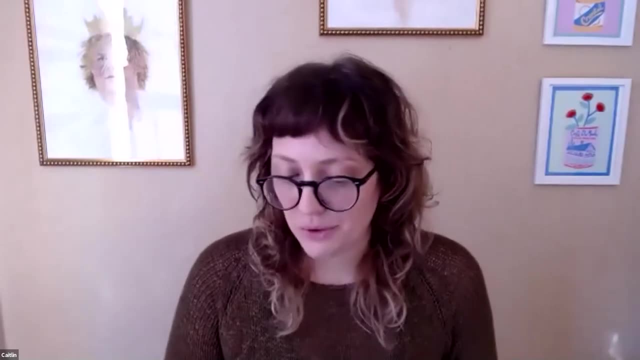 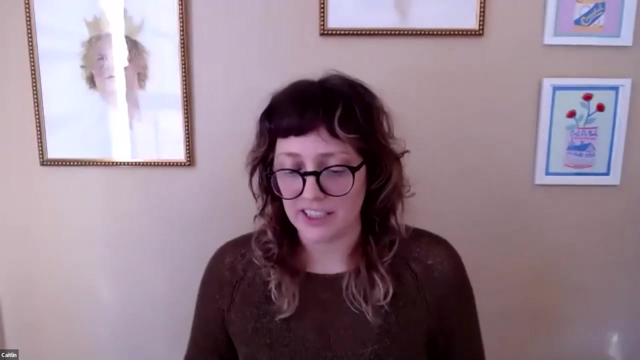 you can Work on secure coding. If you decide that what you really like is programming, you can get very into Doing like DevSecOps and doing secure coding stuff and then completely different than that. There's so many fields It's. I know it's when you're first starting. It's actually kind of. 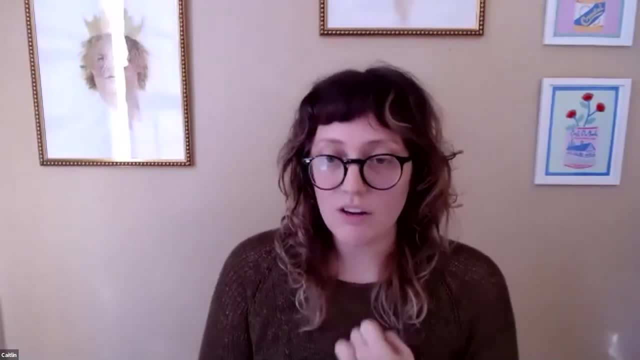 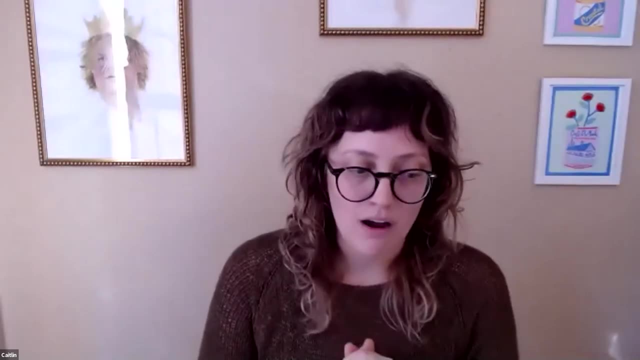 A lot right, It's a little overwhelming. There are things like forensics where you can or you will be like kind of digging around systems and Looking for- Um, looking for things that are hidden or looking for basically what you're looking for in forensics. a. 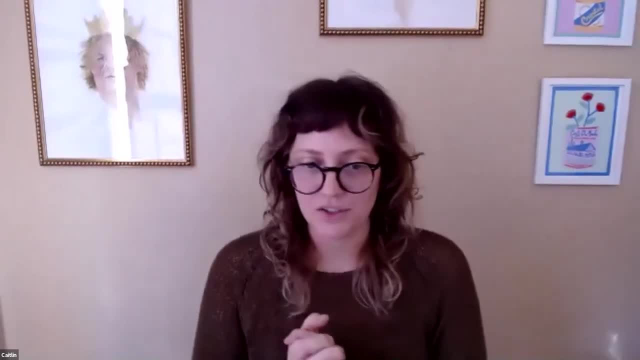 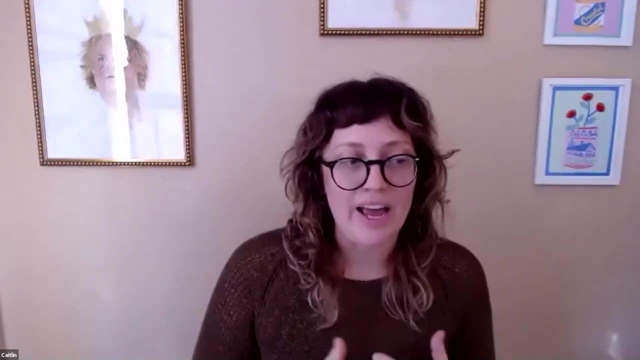 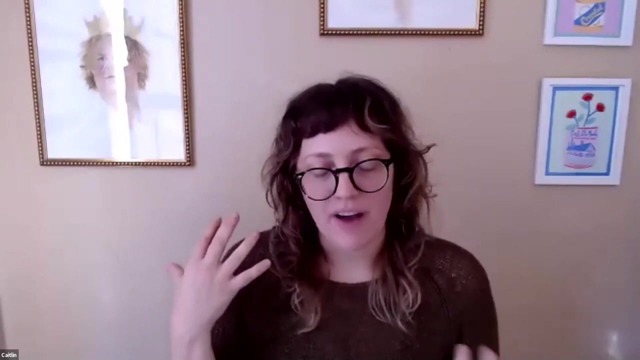 lot of the time is a picture of things that have happened in the past. So what you're trying to do is put together pieces to solve a puzzle about, like why things happened, why a system was exploited or how it was attacked, or you're trying to find files that are hidden. So if you, if that, 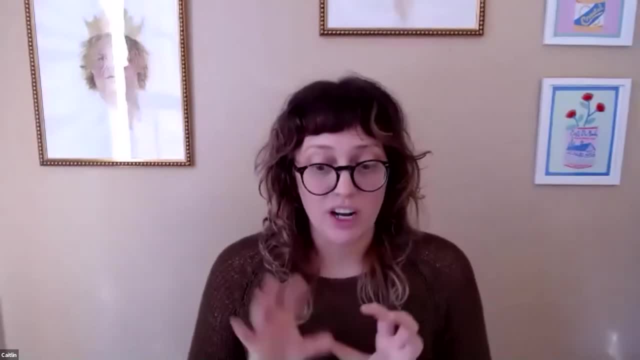 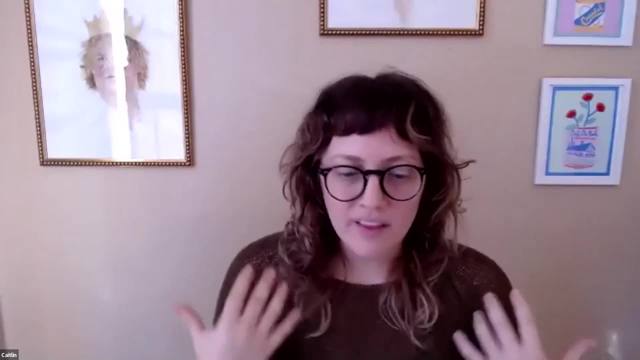 sounds like something you would like. if you really like digging into things, that's a great one. Another one that is really fun if you like to to dig into things. a lot is reverse engineering, So a lot of reverse engineering. you'll be looking at malware and seeing how malware and viruses work. 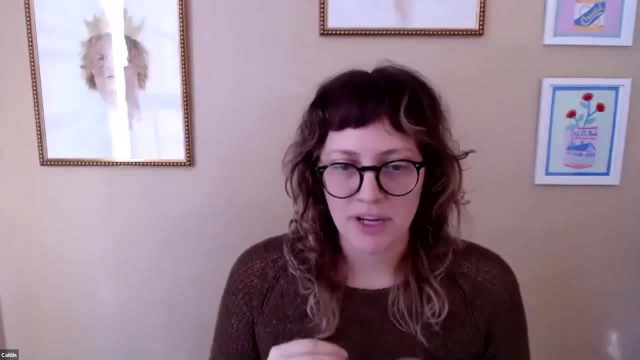 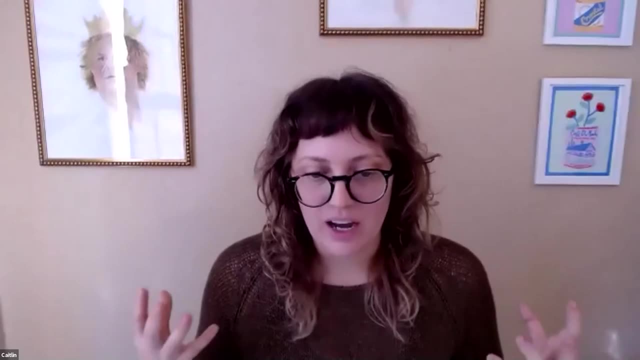 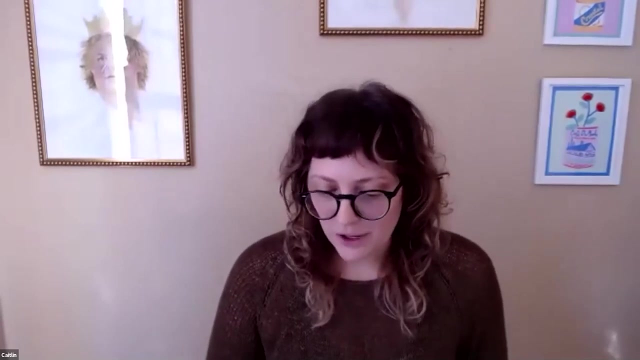 and going through them and trying to pick apart, like sometimes, where they came from or who developed them, what they do, how we can patch our systems to make them not vulnerable to those things. There's also network penetration testing. There's all sorts of like defensive or blue team jobs, where 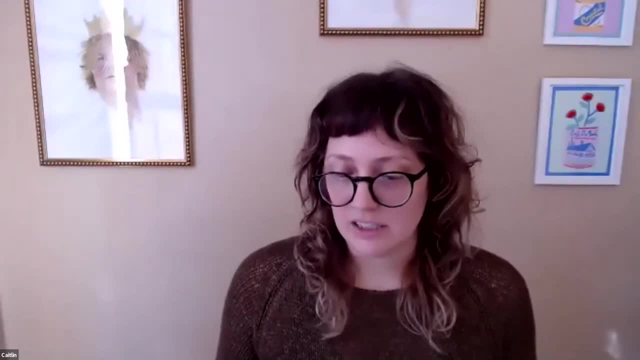 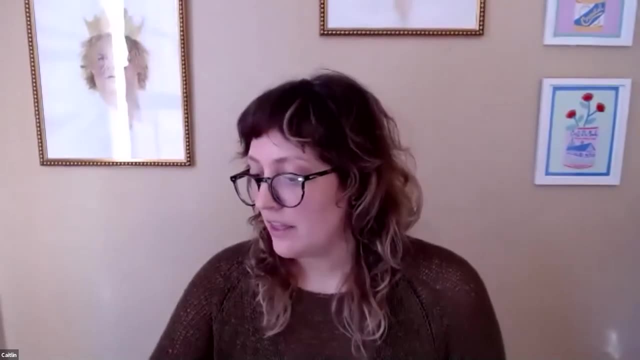 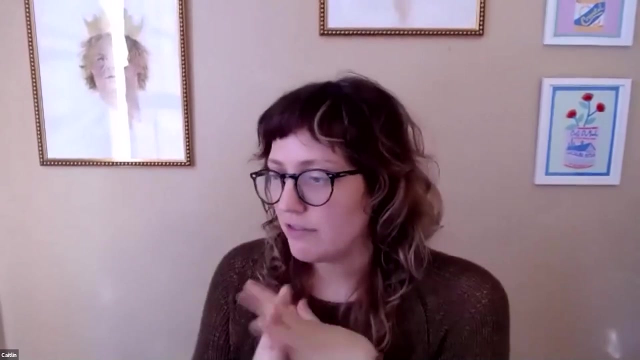 you're trying to make networks and systems invulnerable to attacks. So that would be like systems administrators, things like that There's really. I mean, the great thing about security is, if you're in any way interested, I'm sure you'll find something that like scratches that itch for. 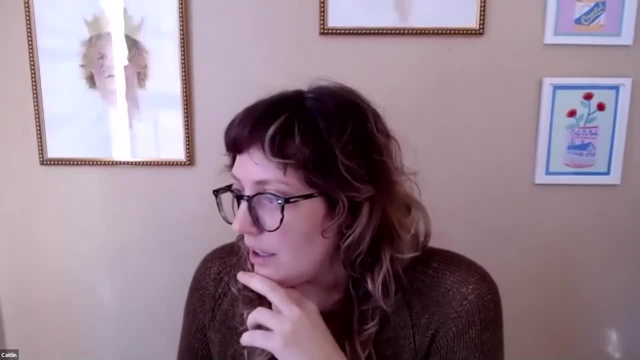 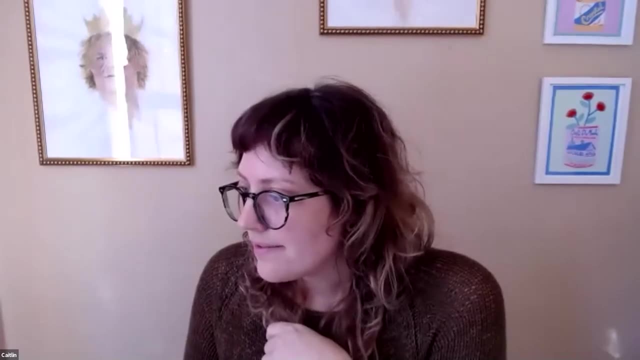 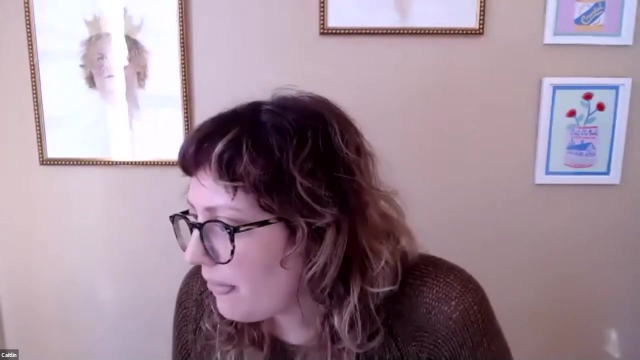 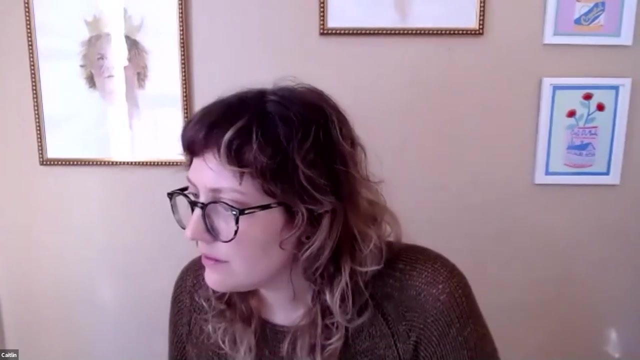 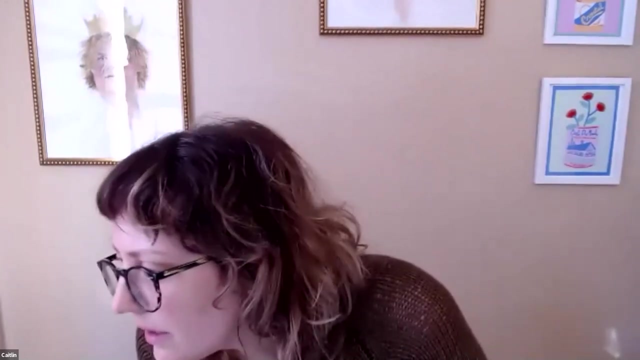 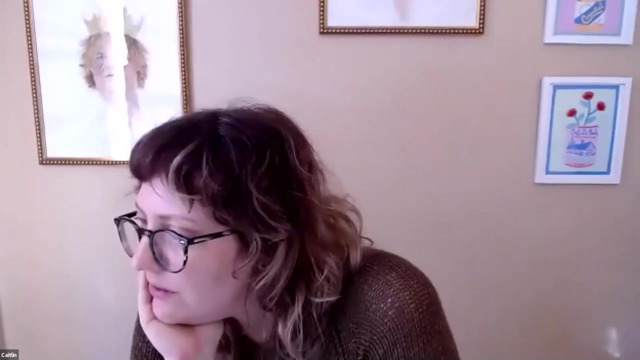 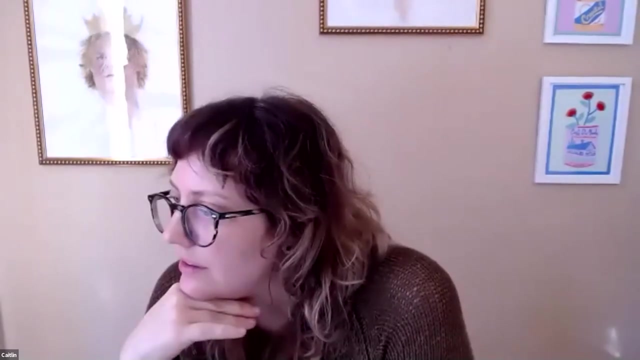 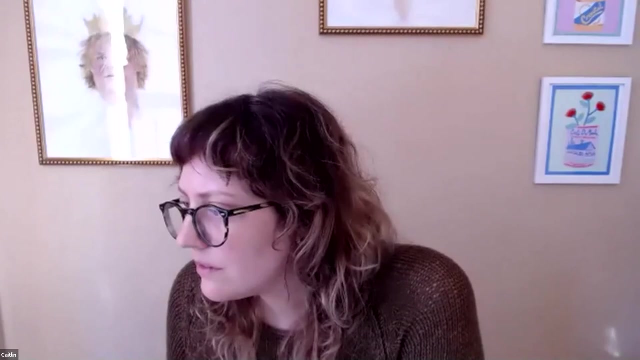 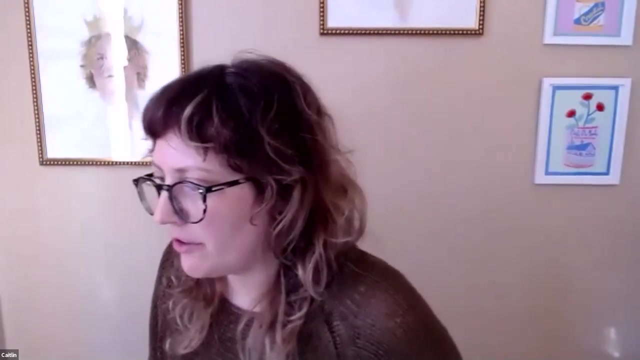 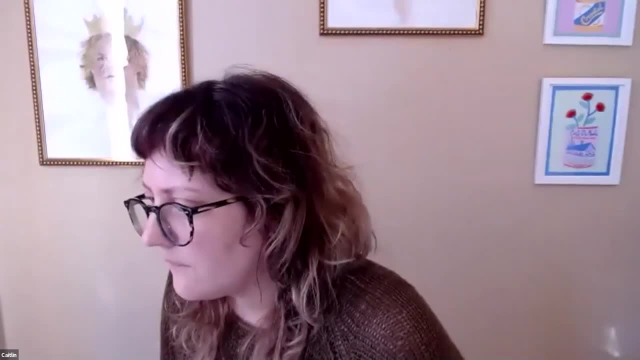 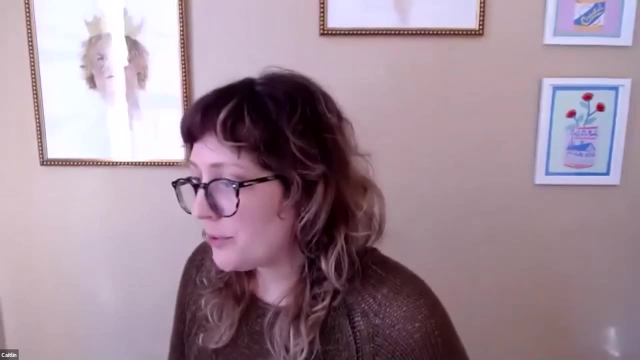 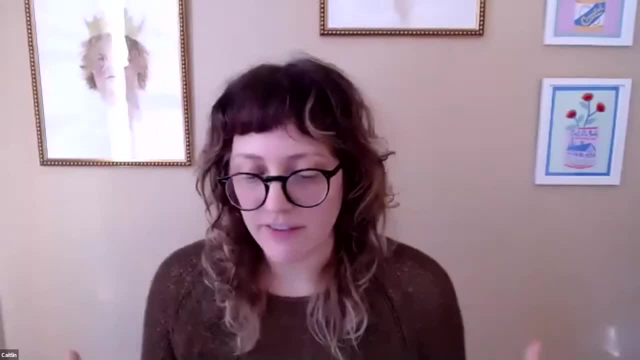 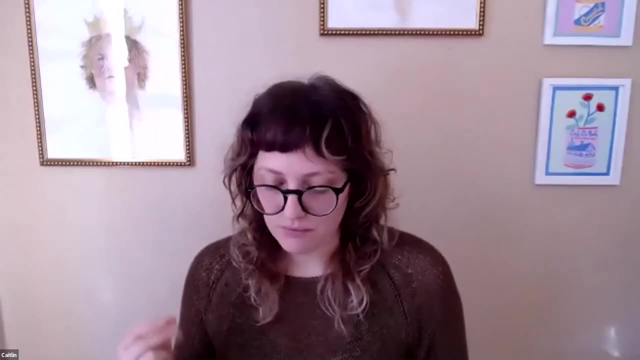 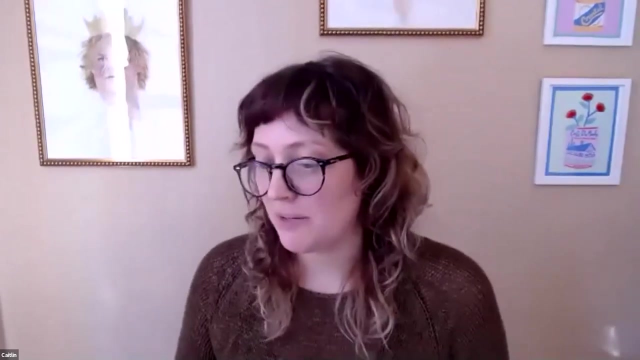 The next place that I would look- either whenever you're trying to find more resources for learning this stuff, or whether you are wanting to- um, um, just uh, solve challenges- is gonna be your search engine, So Google is going to be. 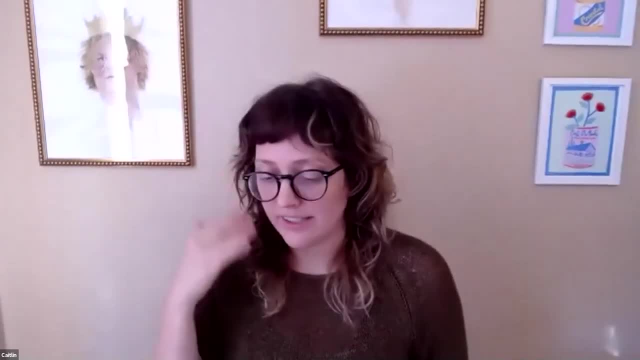 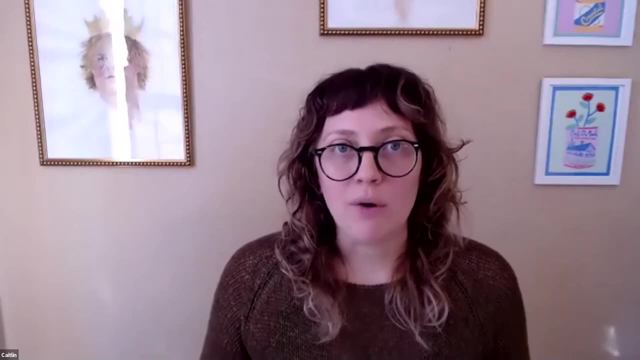 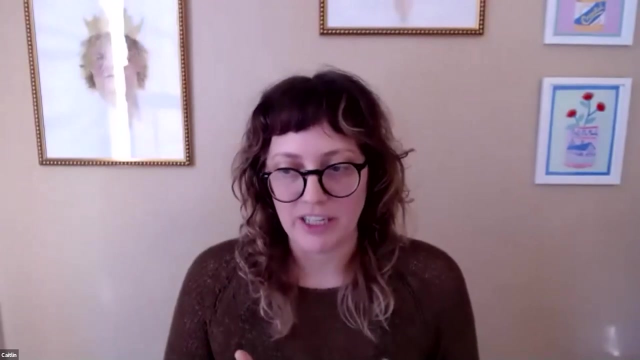 super, super powerful, And one of the really, really, really important skills that game is going to help you with is learning how to create powerful searches so that you can find exactly the information that you want And you figure out how you can apply that information that somebody else has posted about some other situation to your situation. 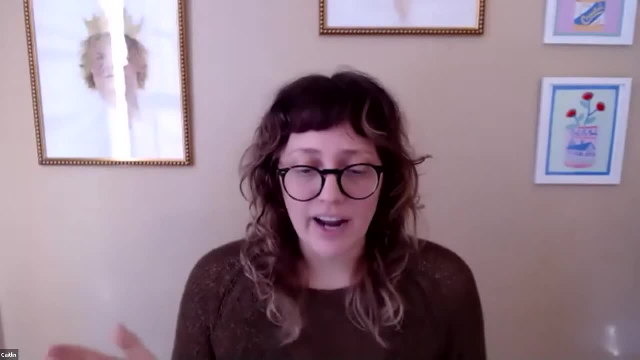 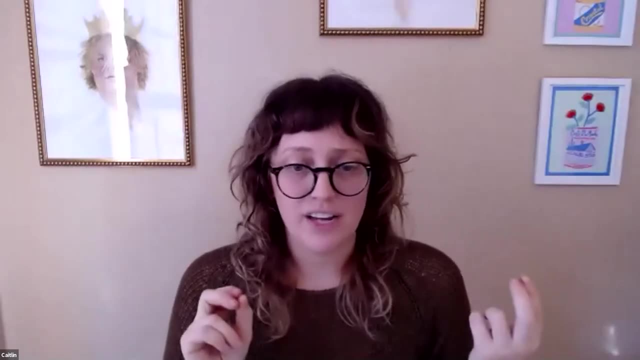 This is really, really big. It kind of feels like cheating, but really in every aspect of tech, uh, Google is like very, very, very important, So developers and programmers use it all the time to figure out problems. Security people use it all the time. 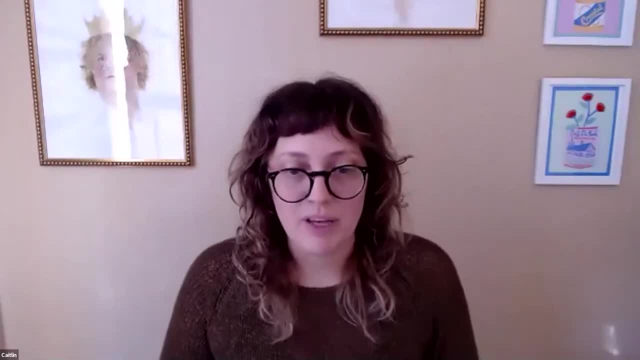 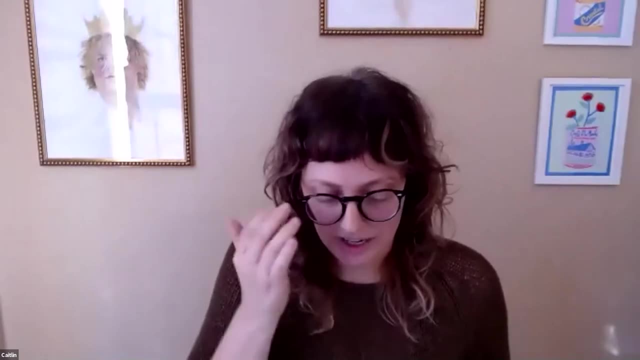 You have the, you know the knowledge of, of people all around the world at your fingertips at all times, So you can really find answers to almost all of your questions there. Some other, um, if you want to, when you finish game. 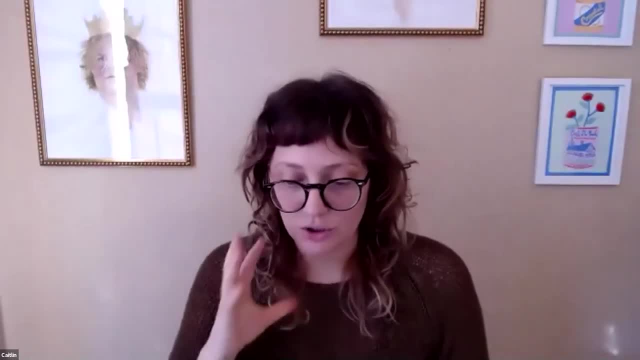 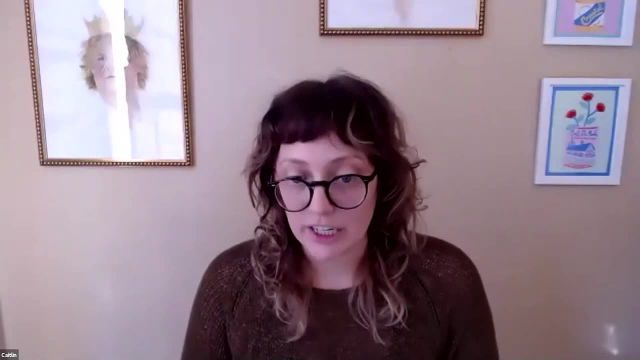 get deeper into some other kind of challenge or or learning opportunities. Um, I always like to recommend: hack the box, the box or over the wire. Those are both very good, Um, but you'll be more equipped for that stuff, Uh. 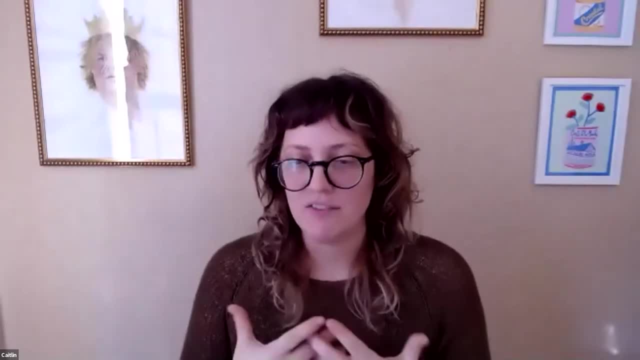 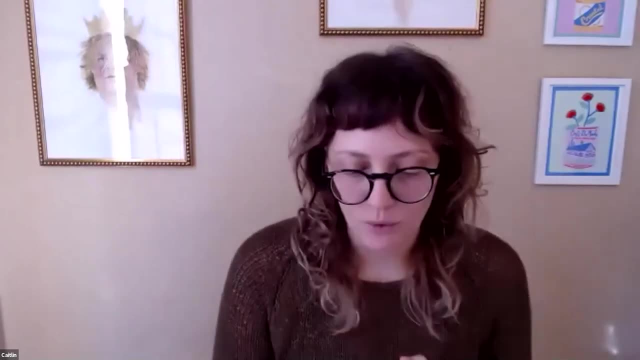 whenever you start doing a little bit of game. it's going to be similar. It's kind of a gamified um approach and it'll teach you some different skills. They're not going to have things like forensics and stuff like that. 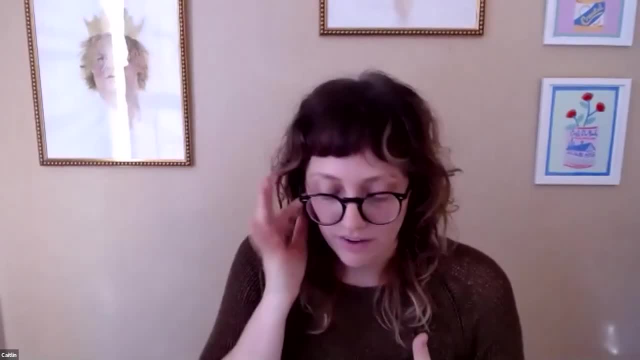 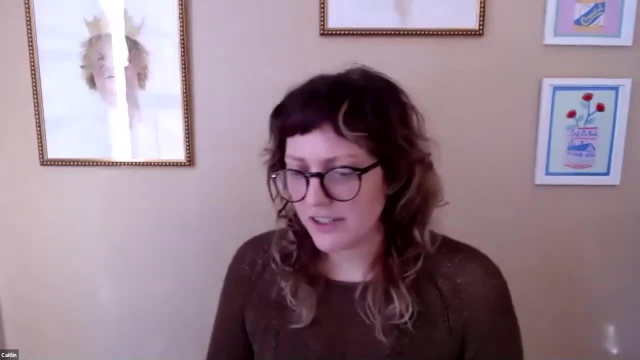 or probably Python programming, but they will have a lot of command line stuff, Um, and that's another place you can look for those kinds of of resources. As far as reverse engineering malware, unicorn has a really, really great guide that I like to get started. 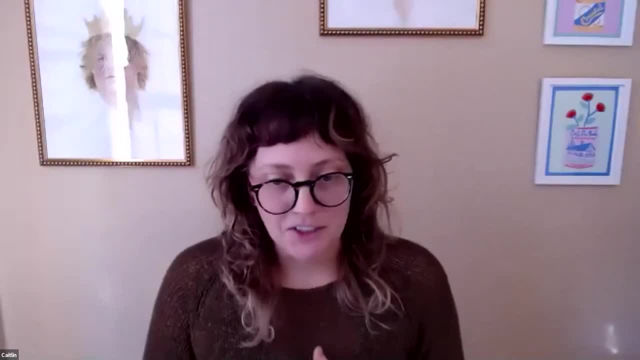 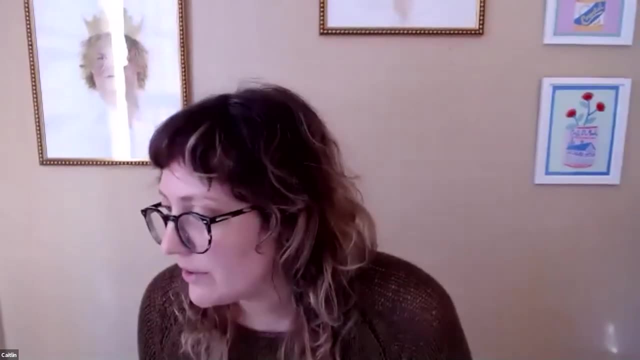 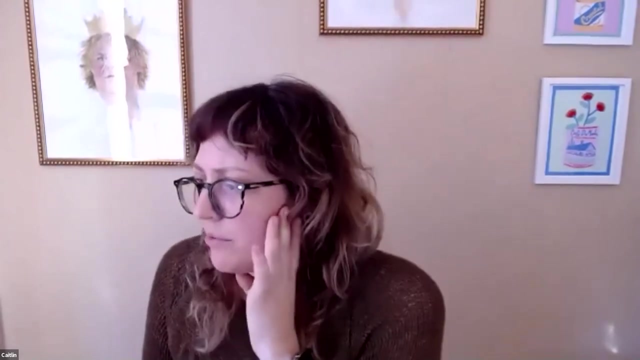 There's some really great books. Um, one of them is practical malware analysis. that has a ton of labs with it, but, um, those are. those are my favorite resources for those kinds of things. Um, I don't know about the Mac with the M one chip virtual box issues. 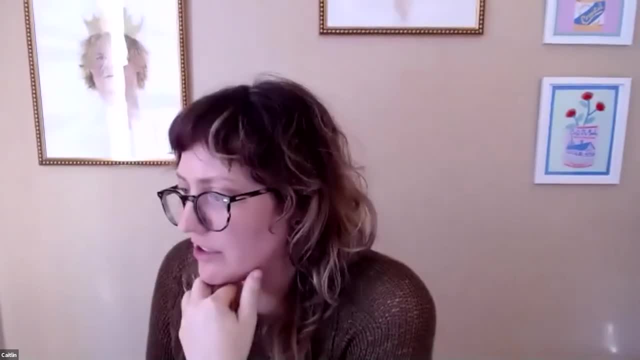 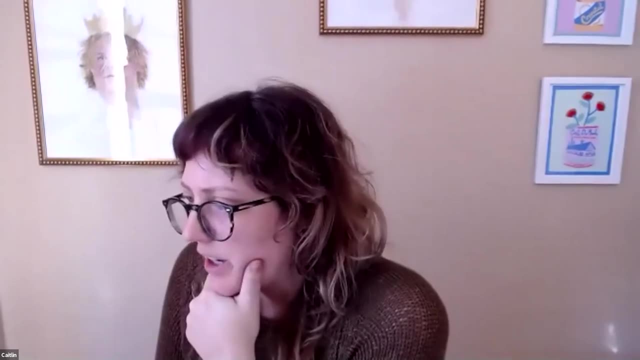 Um, I haven't heard of. I know they were having issues with Docker. I didn't know they were having issues with virtual box. Um, that seems. I think that would be something you could ask. uh, send a support email for red team. 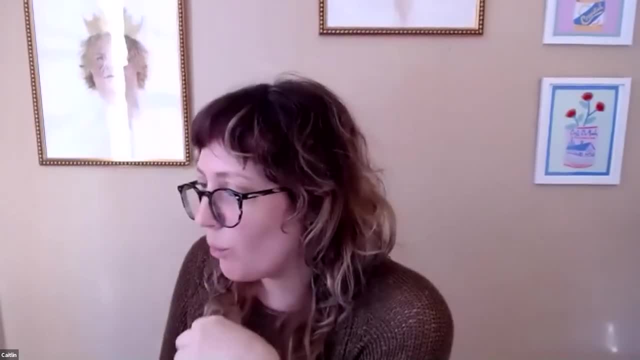 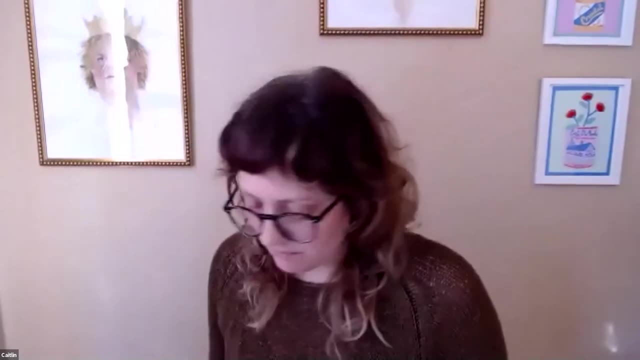 Jobs are kind of difficult to get only because everybody wants them, Cause they're like the super fun, like kind of rock stars of, of security. Um, they get all the attention even though everybody's doing a ton of work. uh. 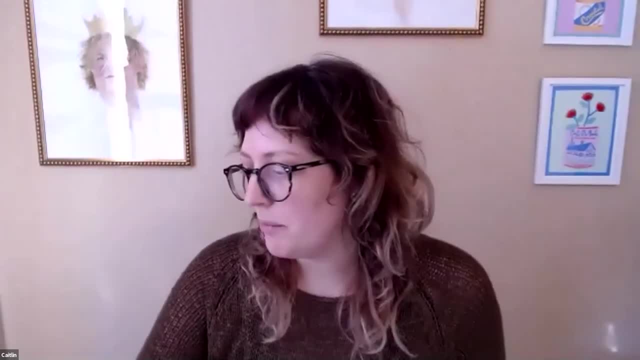 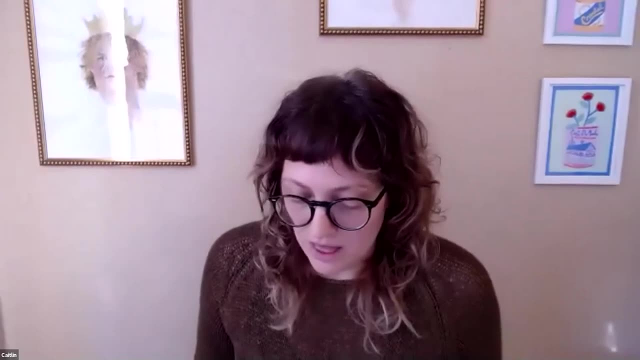 behind the scenes and and really the blue teamers get a little bit less of that upfront appreciation, even though they do, uh, a lot of what I would say is most of the really hard work. Um, red team stuff is difficult because they're often looking for people with 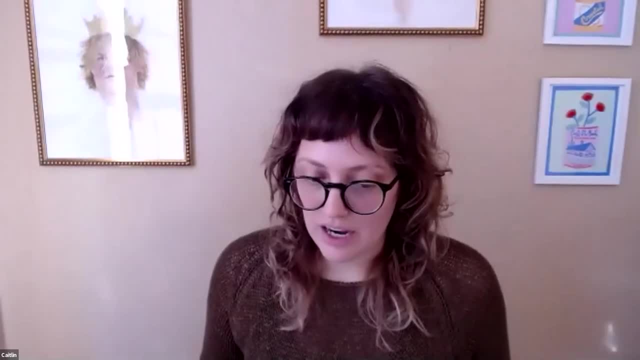 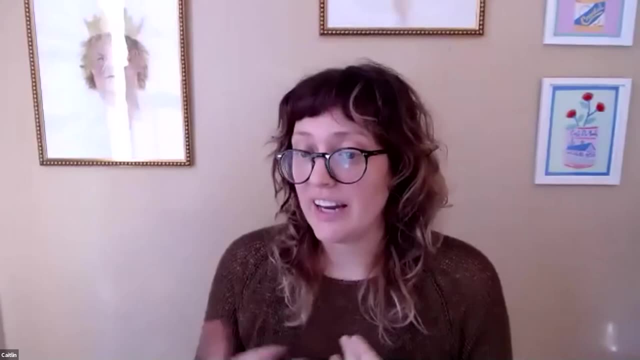 experience and they want, um, there's not a whole lot of jobs for it. So the great thing about things like cyber start game is you're getting experience in kind of some red team stuff. You're getting experience with learning how to exploit these vulnerabilities. 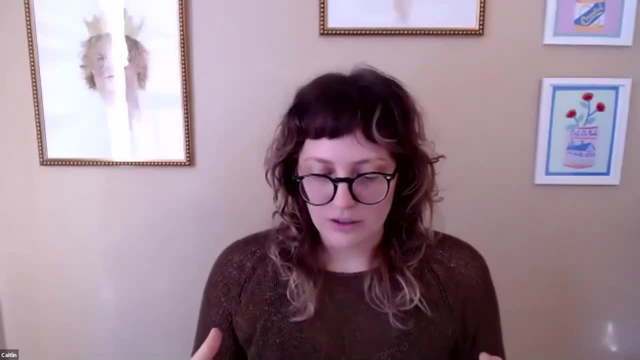 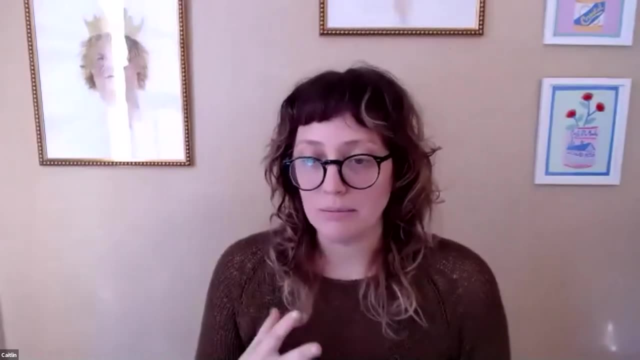 So once we kind of uh give you this little jumping off uh platform, you can keep researching and keep looking and and start researching places that will hire you. Um, SYNAC has a red team. that is basically um. remote and contractor based. Uh, there's lots of of bug bounty um companies. uh, that will um find other corporations that are looking for people to um look at their security. So it's definitely possible Uh. 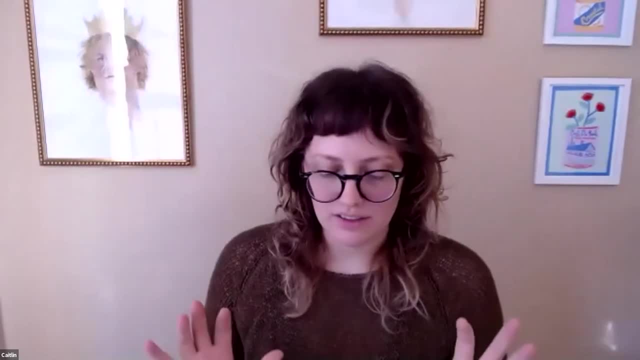 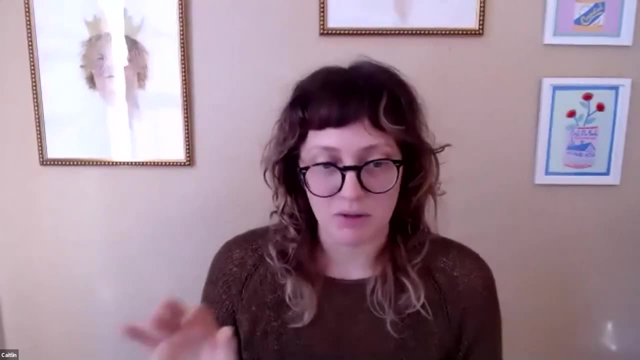 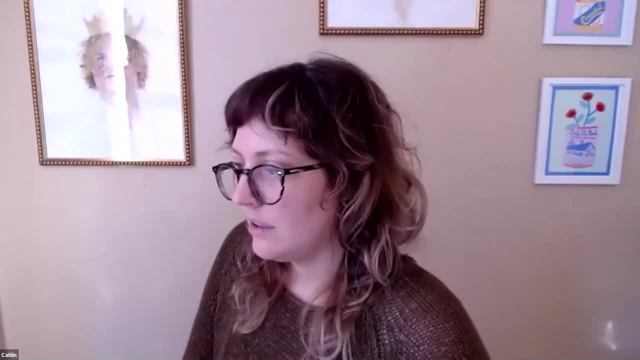 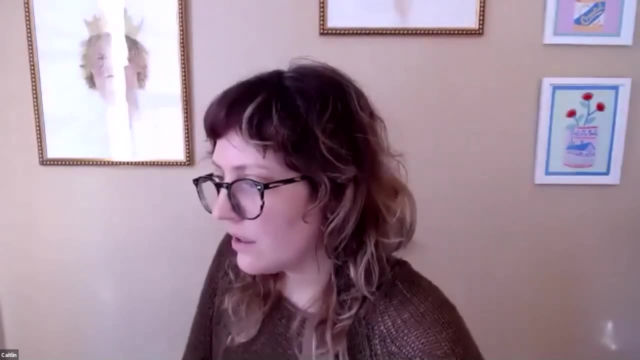 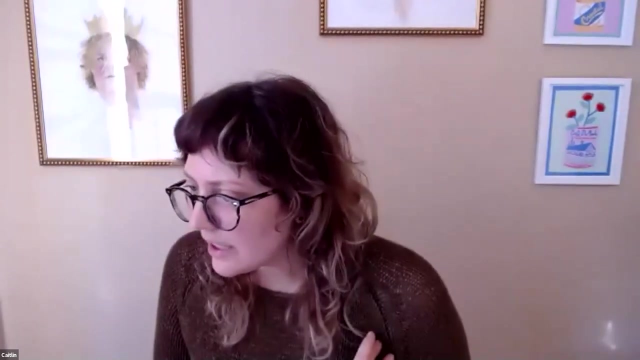 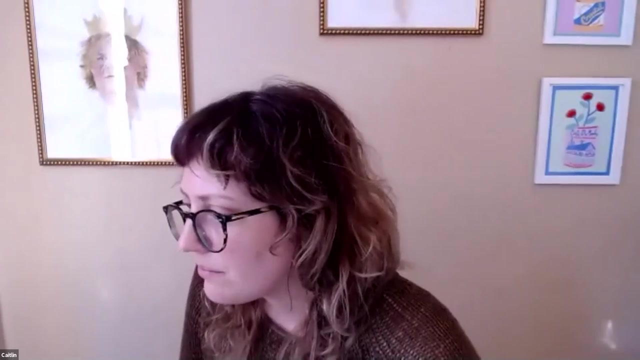 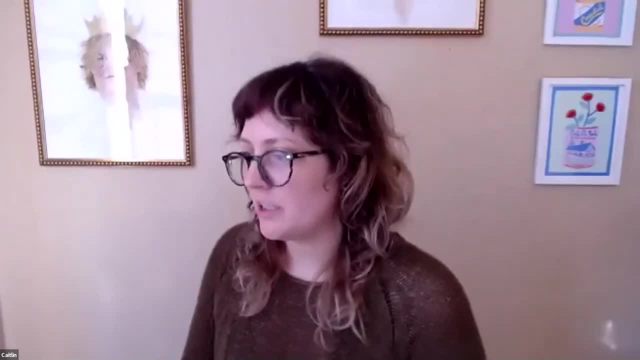 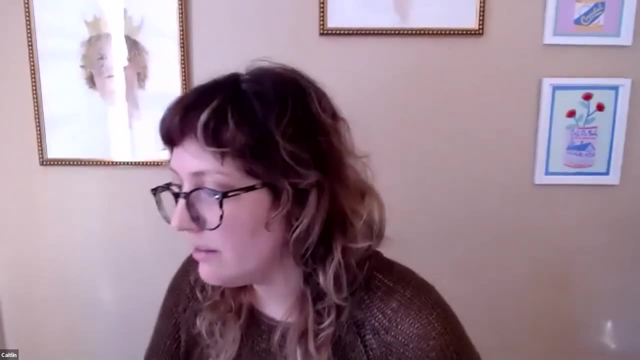 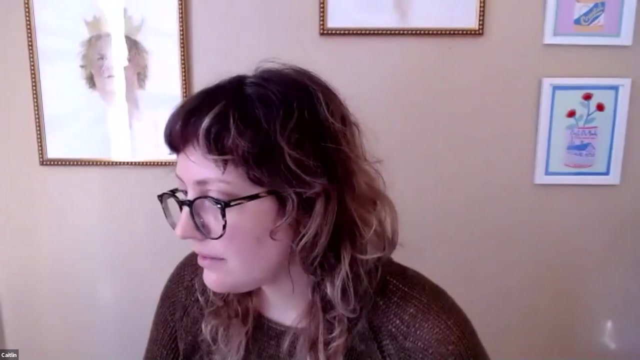 so career opportunities or careers with most opportunity and highest pay is a great question. for Google, That's going to also vary by where you live or where you want to live. That's another question that I always get asked about the question and do I go out of my way? 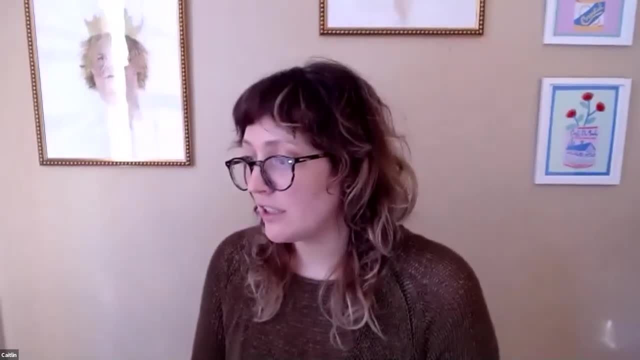 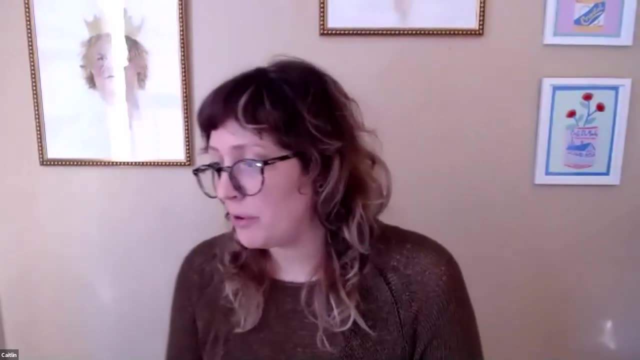 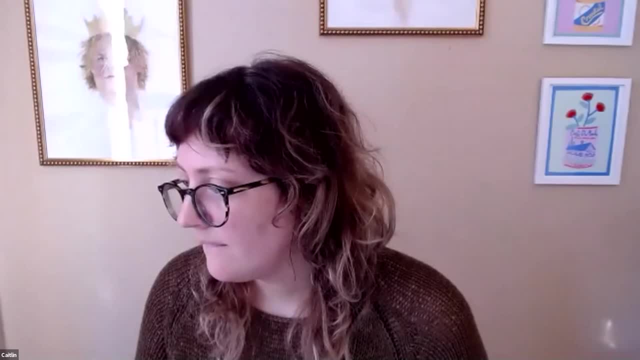 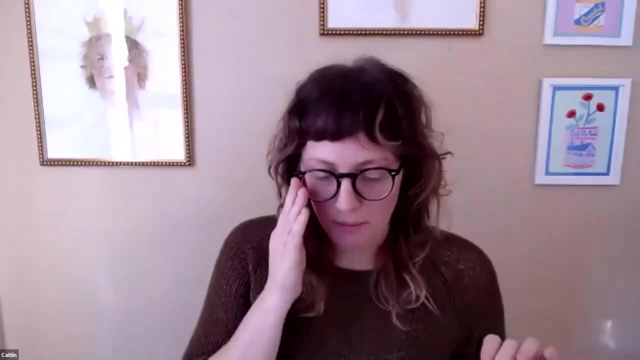 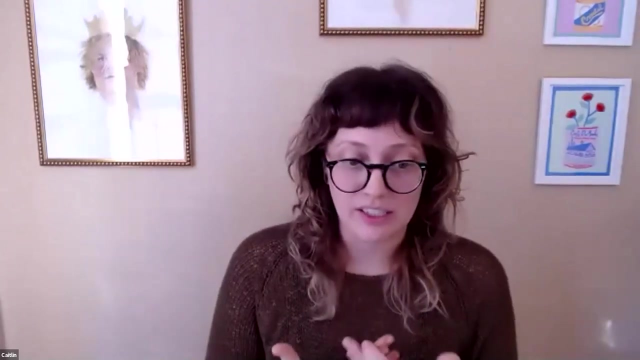 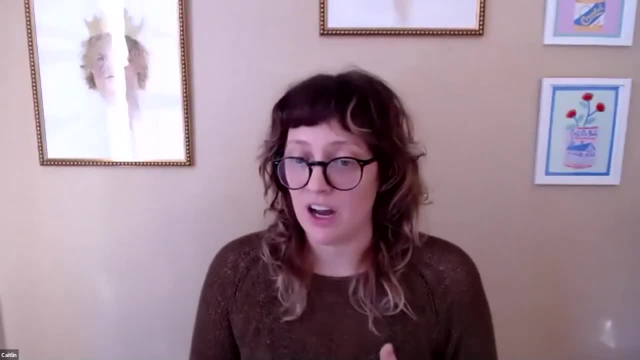 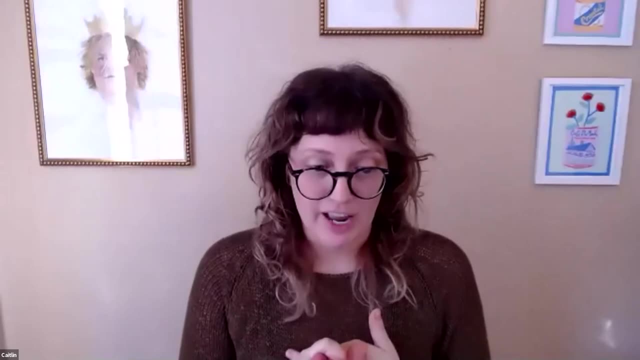 when I was looking at internships. a lot of times they're unpaid internships when I was in college. But there are like no unpaid internships in development or in cybersecurity And if someone tries to get you to do an unpaid internship, I would say you shouldn't do that because there. 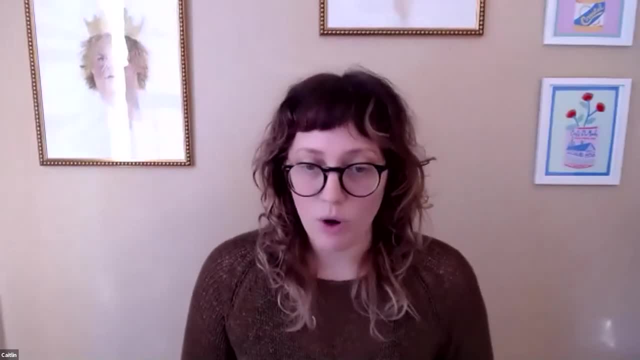 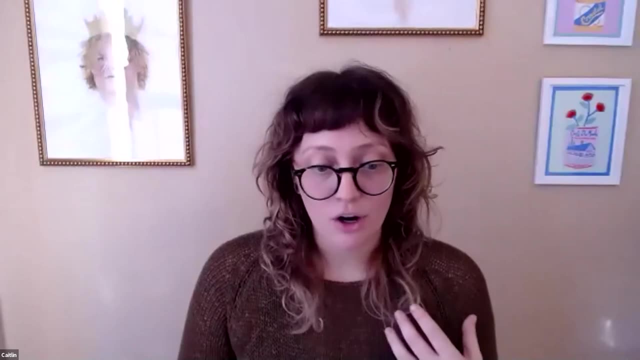 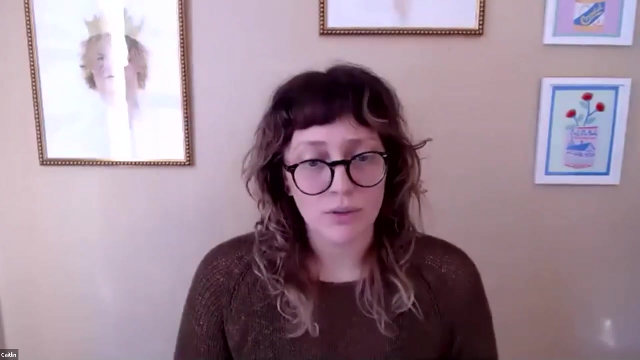 are so many opportunities to get paid for your work while you're learning. Most big corporations do internships, like Amazon, Apple, Cisco, Google. They are all going to have huge, huge internship programs And, honestly, also a lot of little like local places will have internships too. So 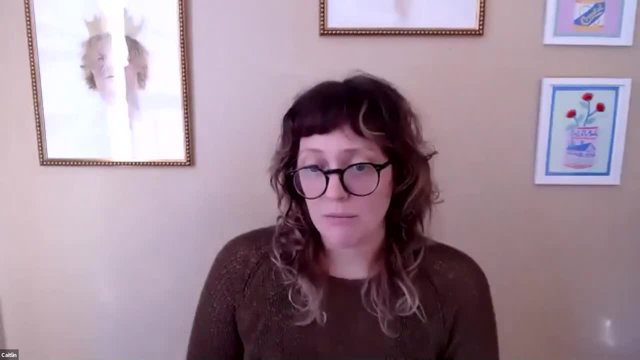 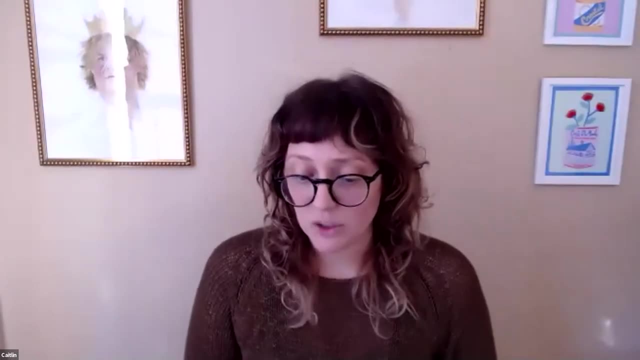 what I would do if I were you is just reach out to them, ask them about their intern programs and go from there. Do some research on the kinds of places that you would like to work for. So if you're looking at different security programs, 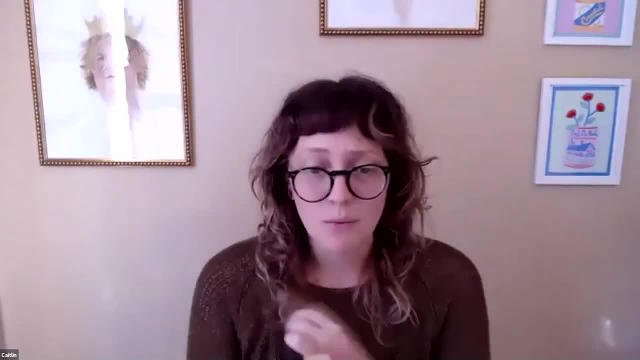 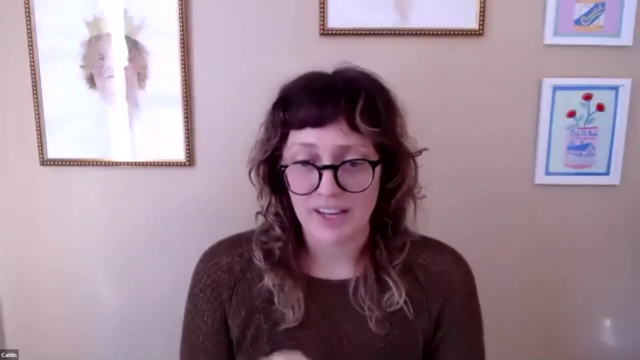 internships you can do anything from. like I know the New York Times had one. So if you want to work for somebody that's not doing exclusively security, you can do something like that. There are actual security firms that have them, like Drago's has them. So just do a little bit. 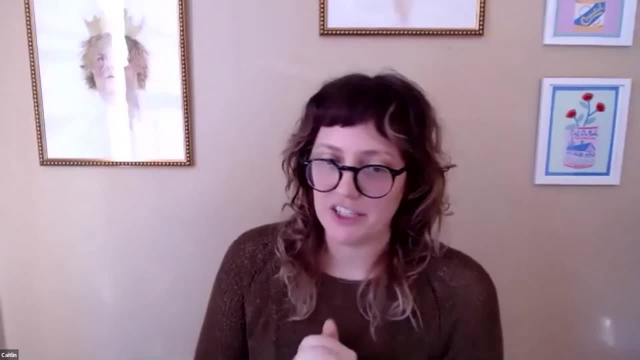 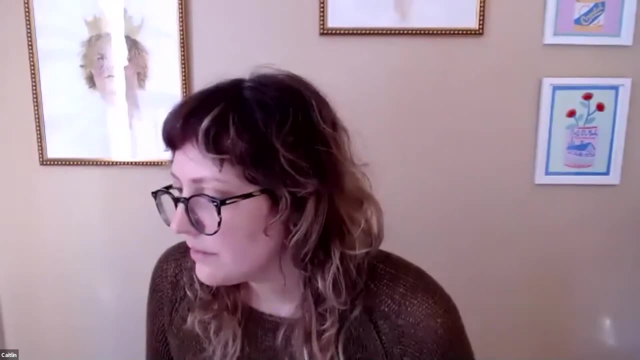 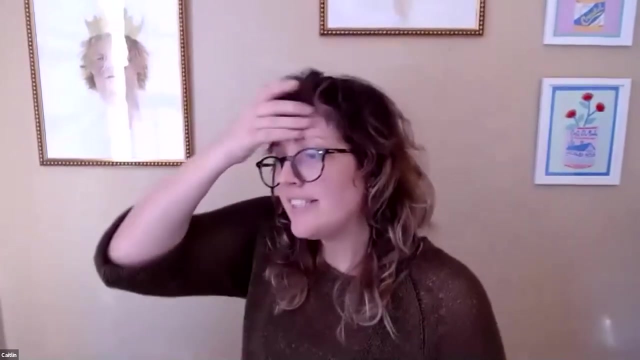 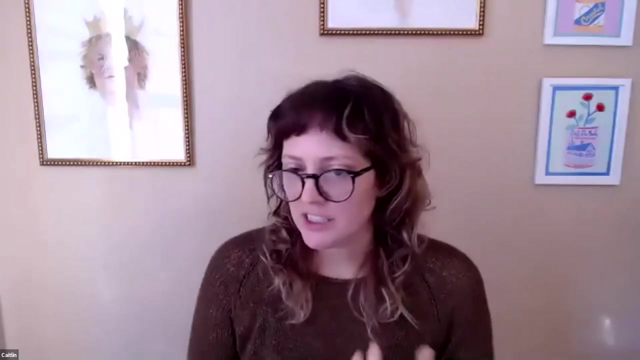 of research, see where you want to work, And I can almost guarantee you they'll have an intern program. So I'm just going toalles Doo, Oh, okay, Red team and blue team. So whenever I say things like red team and blue team, red team is more. 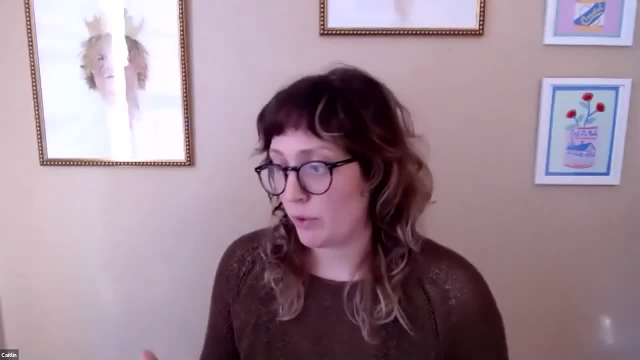 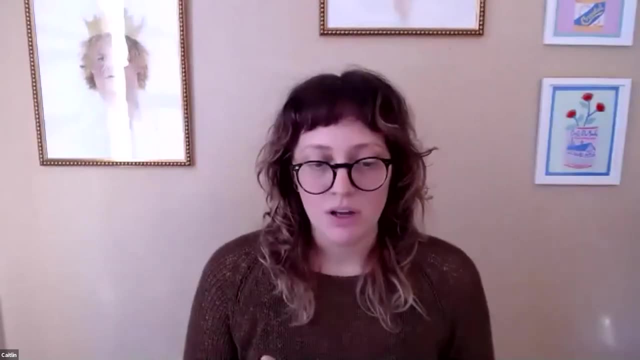 of the offensive security. So things like network penetration testing, Web app penetration testing, those are red teams things where, if you are a red team security member, you are going in and you're trying to exploit things right. So you're trying to break into places You're not supposed to be. Blue team is the exact opposite. Blue team is trying to keep everybody out, So you're doing all the defensive security. 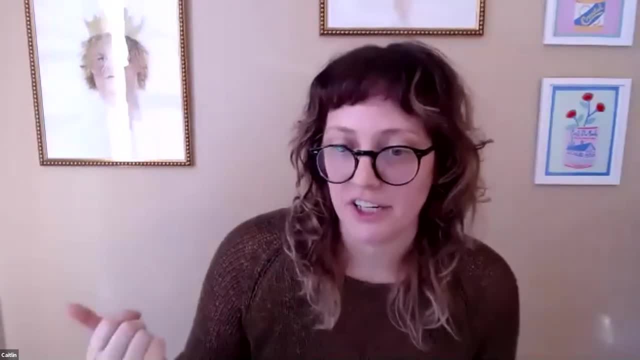 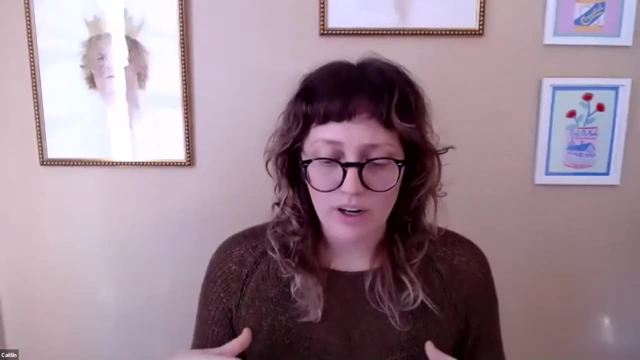 there And you're trying to make sure that there are no gaps or holes in your security. There's no vulnerabilities there where attackers can get in, So they're on opposing sides there. I think more and more there are a lot of purple team positions too, So you're doing a little bit. 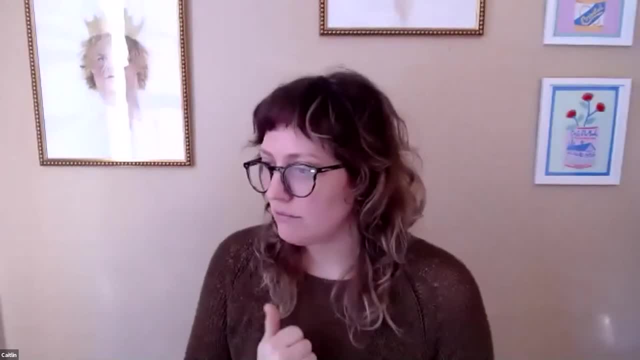 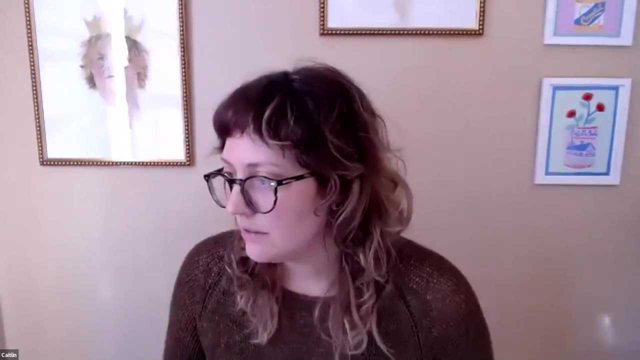 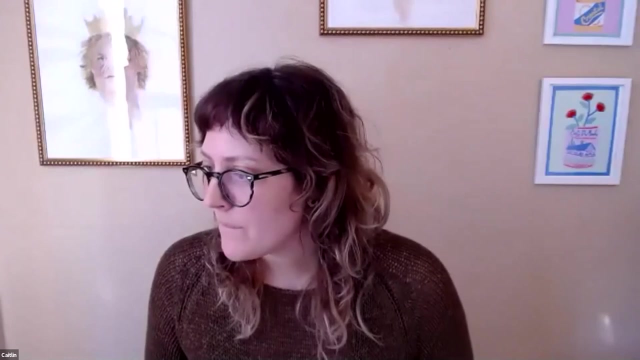 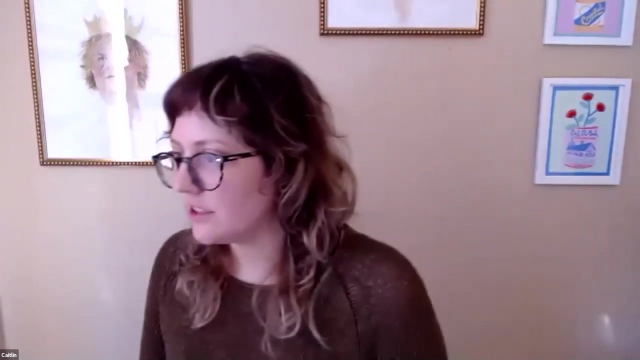 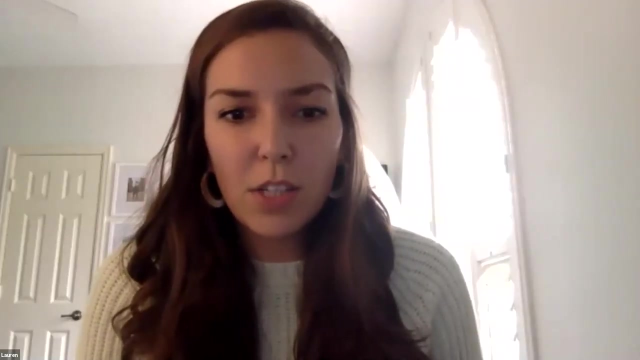 of both. I think that is becoming more and more common, So I hope that answers that question about blue and red team. I don't know if support thought or any other questions that they think I should jump in on. Yeah, And also if anyone has any questions, technical questions, that. 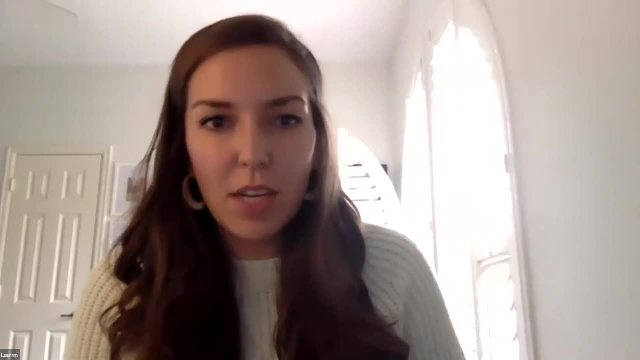 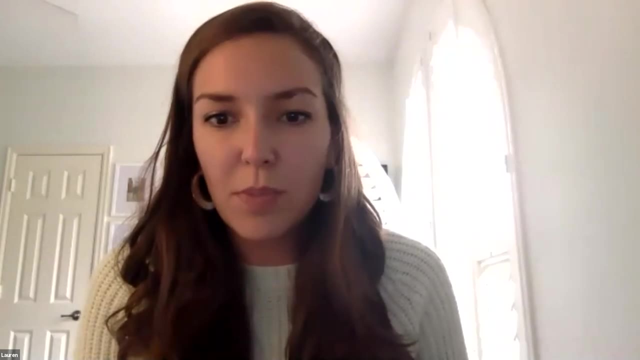 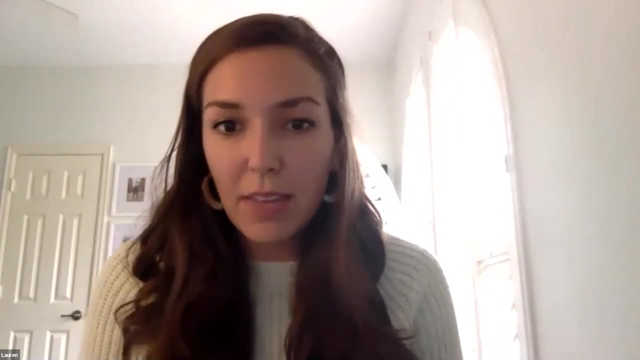 weren't answered, you can always go and post that in the community, The CyberStart America community. I did see one question about how do we get the scholarships For one. you have to complete at least 20% of CyberStart game to qualify to compete in the. 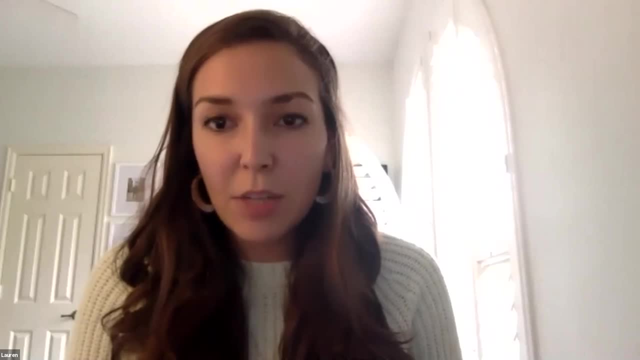 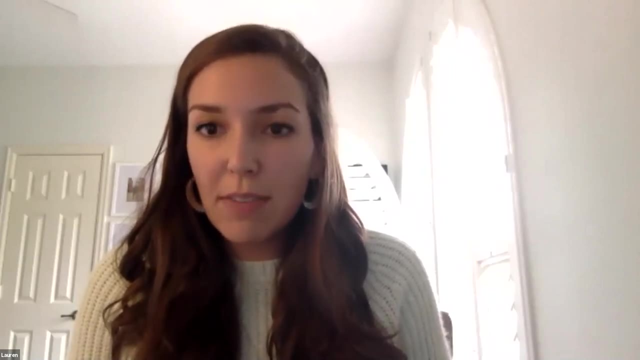 National Cyber Scholarship Competition And then to actually become a scholar, we're going to take the top 600 who perform the best in the competition And in order to receive that scholarship you do have to be a high school junior or senior, But if you are a finalist, that can be freshman to senior, So you don't have to be a junior or senior to become a finalist. Just wanted to get that question answered. Let me see I'll jump back on and see if there's anything that I can answer really quickly. We're. almost at time. Let's see. If you want to travel, I would say some good careers would be. incident response, which I didn't mention before, would be a big one, But if you're a senior, you can be one because you'll be going to um different places to help them, uh, deal with incidents, um what that? 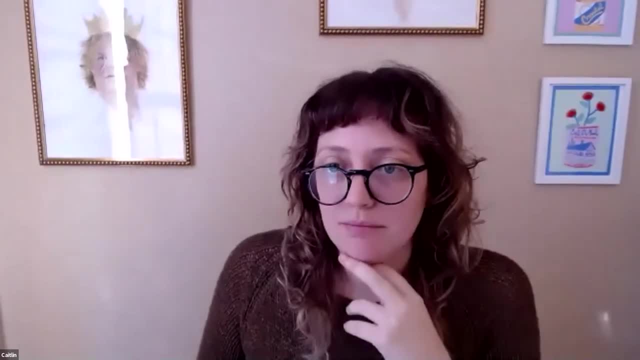 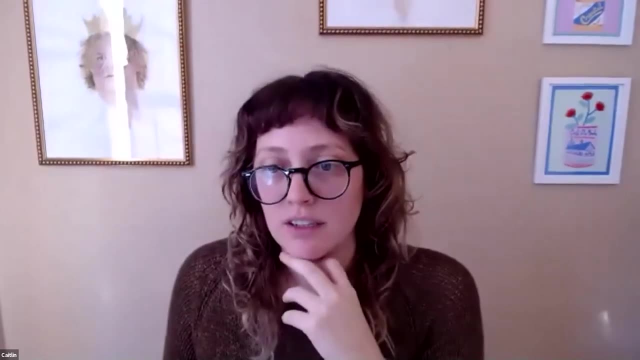 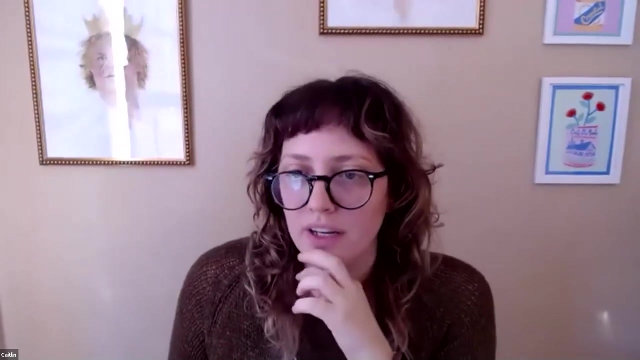 would be. that's a great one. i think a lot of um jobs allow for some travel, but that is the one that comes to mind first. um, as far as intern programs for high school students, i don't know the answer to that, so for sure there are in colleges and the great things about what you're. 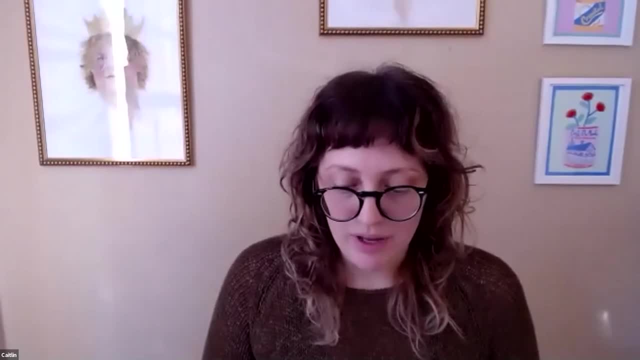 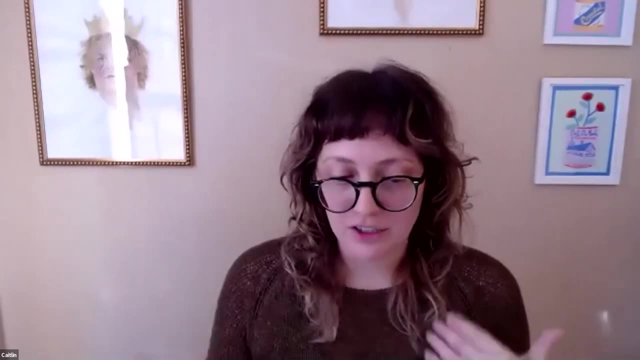 doing now with, and what we're doing with cyber start game? um, is you're going to have a kind of a jump start on other people who are who are in college looking for their interns? like right, internships right away? um, again for high school internships. i would just google it and i would. 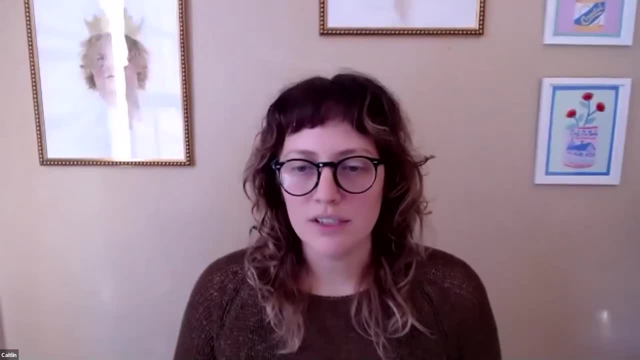 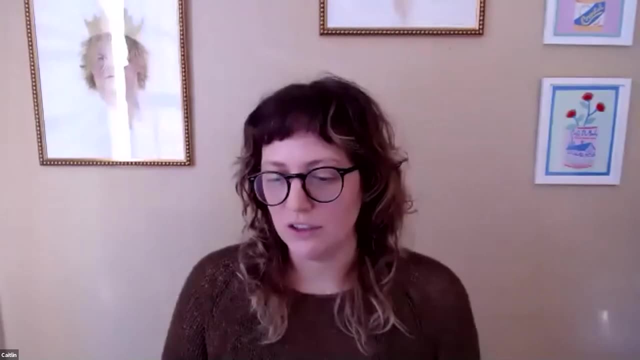 also, there's nothing wrong with reaching out and asking a company if they're willing to take on high school students. the only thing that can tell you is that they can't do that right now. right, so there's nothing to lose there if you're interested in interning with somebody- and i think a lot of these internships that would take high. 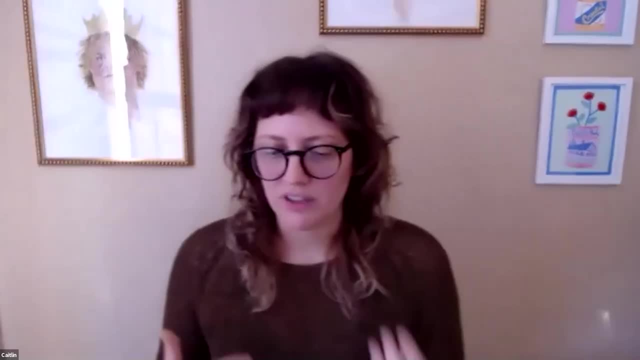 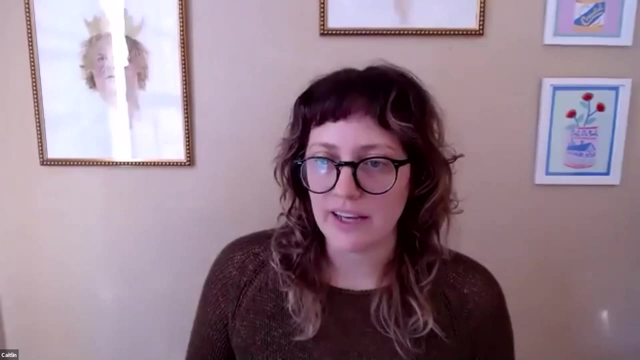 schoolers would probably be places that are local. i don't think. i think that maybe one of the things that keeps uh high schoolers from being able to intern is that ability to travel and live on their own. but if you're able to find a company locally that can do some sort of um it or security. 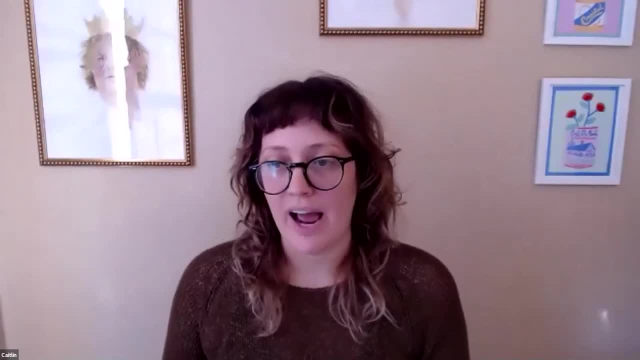 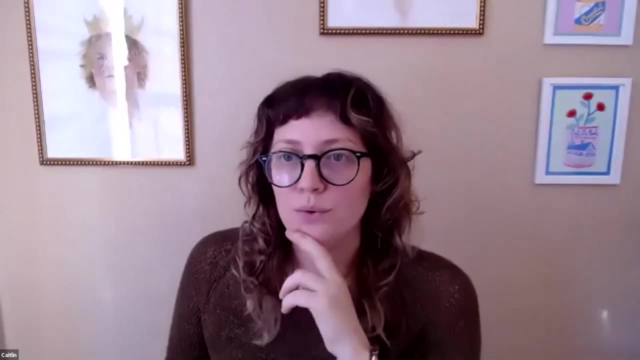 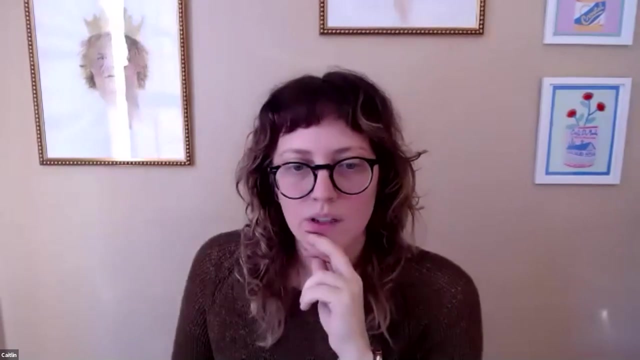 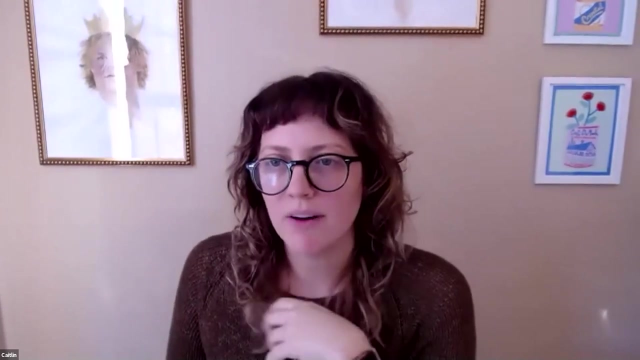 internship. that's a great place to start. a good person to ask um. i think that's a great place to start. i think that's a great place to start. um, i think that's a great place to start. okay, i see this question about how to get the scholarship. is that what you just answered, lauren? 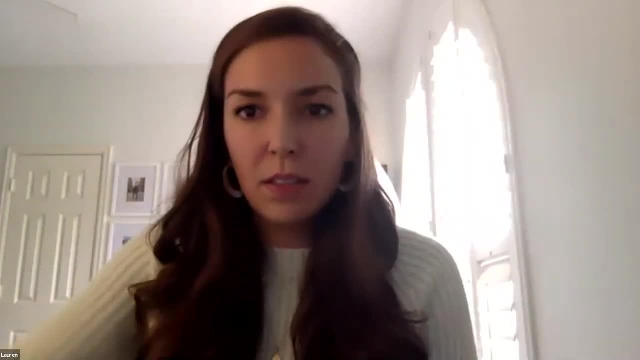 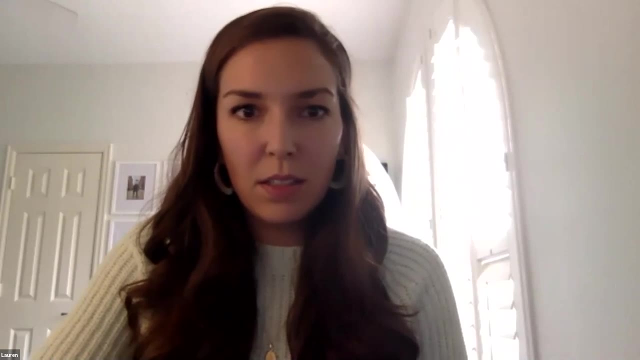 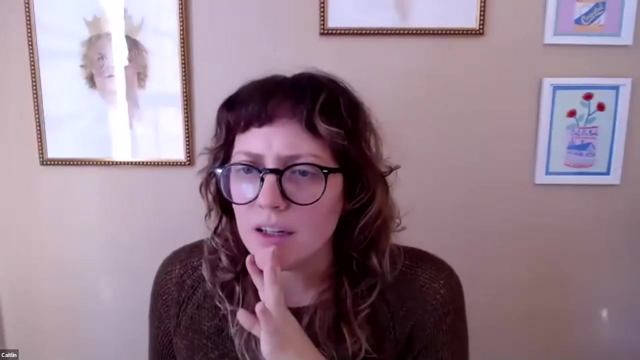 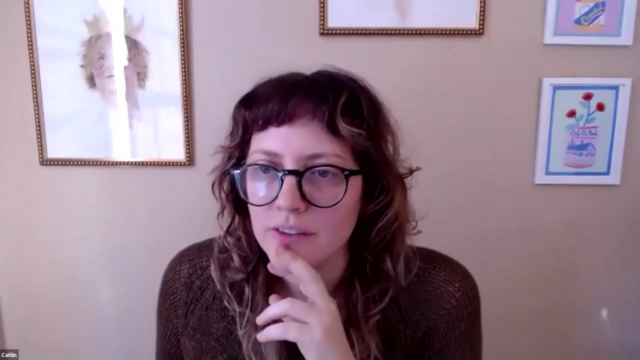 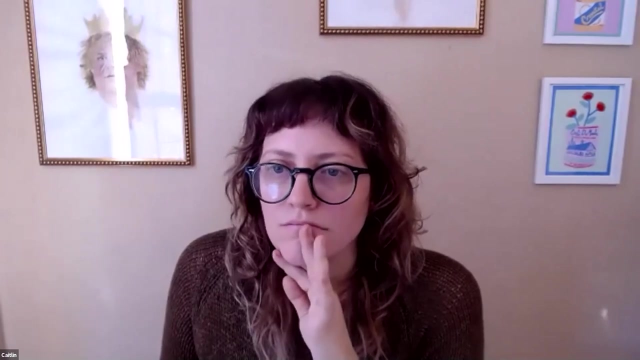 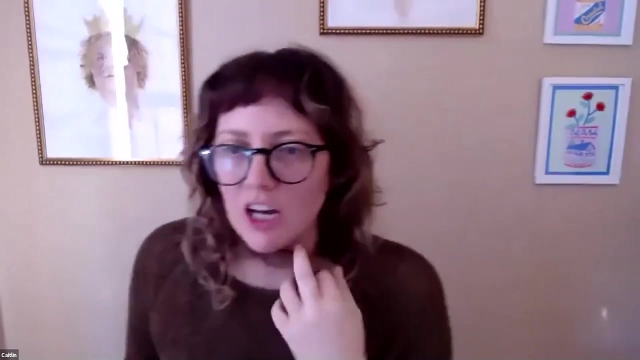 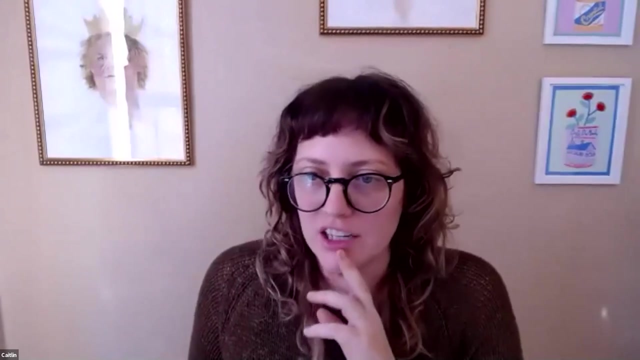 okay, great, yeah, do you see any other questions you can answer, caitlyn? um, i am not seeing any thing that i think is a quick one. i'm just kind of scrolling a beginner friendly cyber job. so a lot of sock analytics jobs are going to be kind of entry-level beginner and beginner jobs, security analyst jobs. that. 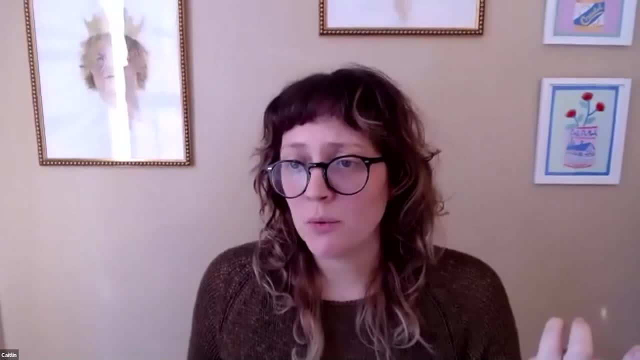 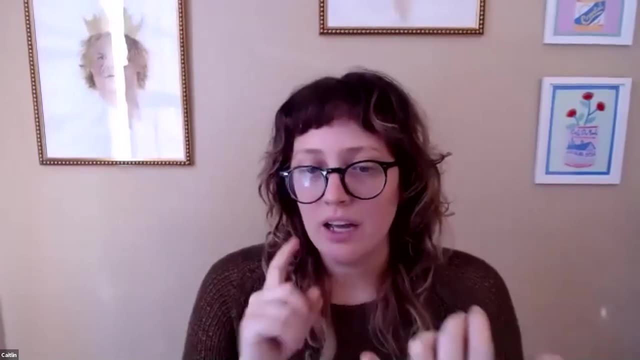 kind of stuff is often open to beginners. but there are also companies who are willing to take on um beginners in anything if you look, if you look hard enough. so there are people who are willing to train you um in things like, uh, you know, forensics or red team stuff or incident response. 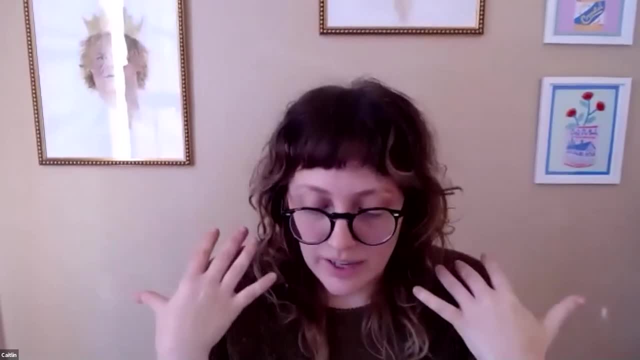 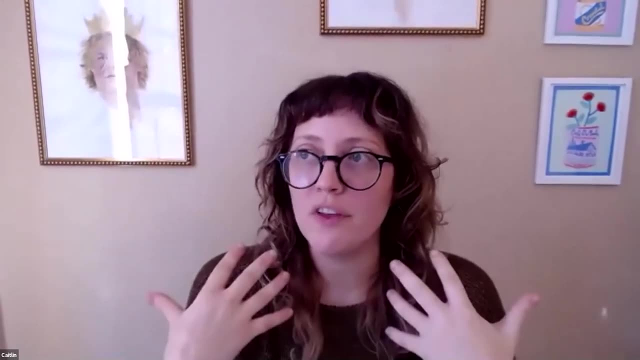 um, if you have a, what you really need to get good at illustrating is how your interest and why you're passionate about it and why you want to do this. and then there, if you, if people know that you have the interest, the desire to learn and that capability, they're going to be a lot more. 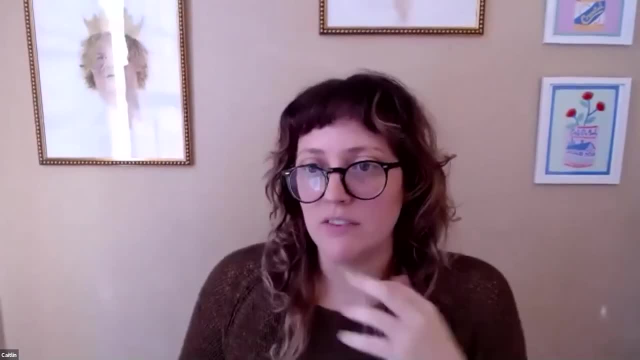 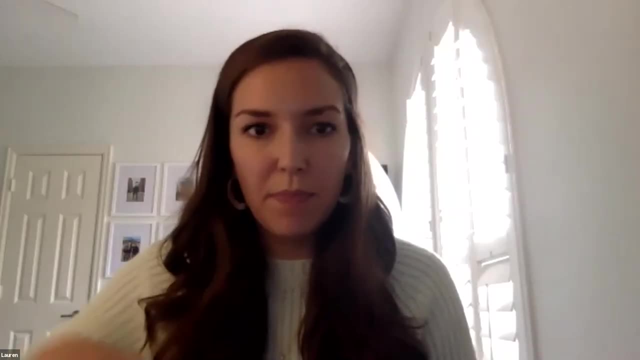 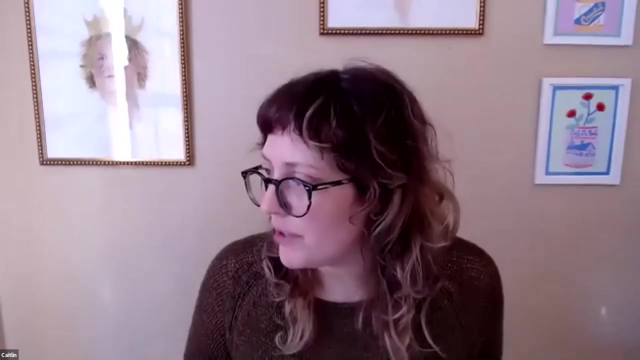 willing to, uh, invest in you regardless of your level of experience. i think we can probably call it there. we can wrap up, we go ahead and share that one last slide. yes, um, and then also, i think this is being recorded right, so anybody who missed what i was doing, i'm going to put it in the chat box. 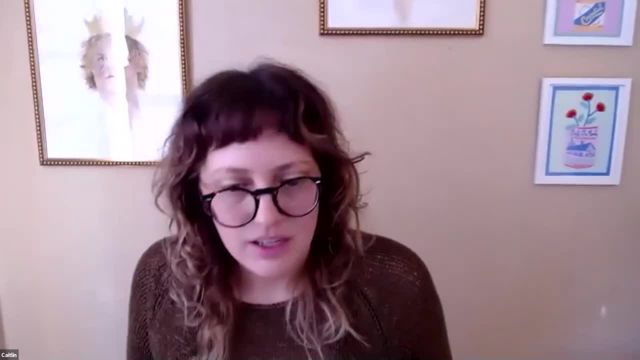 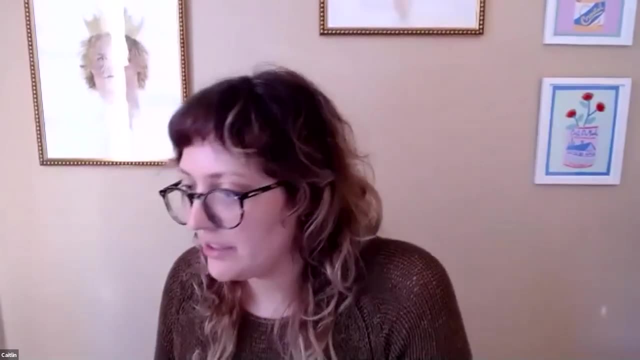 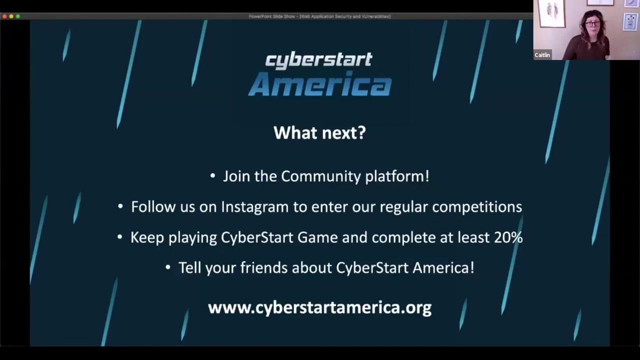 so anybody who missed what i was doing in those challenge walkthroughs can certainly watch the recording and try and catch it again. let me find my screen share all right. so i saw a lot of questions in the chat box about joining the community. if you didn't receive that email, go ahead and send a an email to support cyberstartamericaorg, because after you register for cyberstart, you should receive an email inviting you to the community platform. so if you didn't get that, just go ahead and send them an email and we'll get you invited right away, because then we'll also 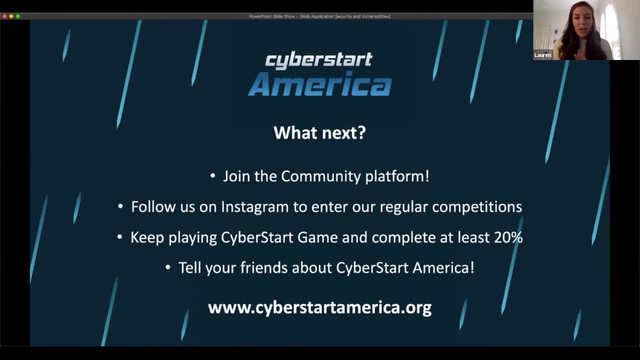 probably post the recording there as well as uh answer any other questions, uh, and then, like i said earlier, follow us on instagram, that's at cyberstartusa, and then you'll be able to take part in the campaign and you should be able to even have the opportunity to get a chance to join the. 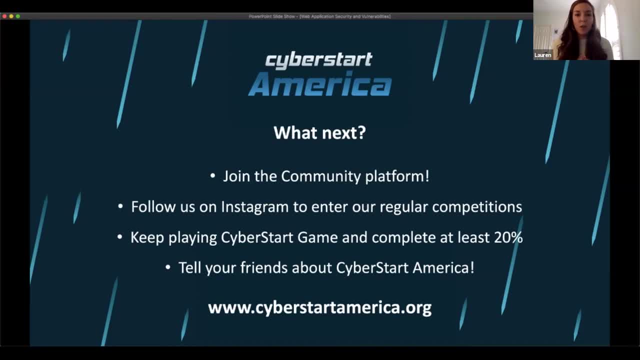 number of customers that you've got to have to enter the content of a song, so just look out for that. a lot of you will be able to take part as well and then follow me on instagram and then i'll email you to don't forget to subscribe to the community to help me single off on that. so 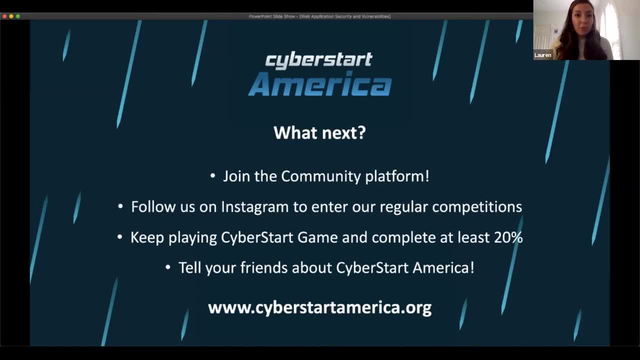 that you won't miss my next video. i hope you have a great day. take care everyone, and i will see you next time. bye, you can also be on the stash at cyberstartamericaorg and 6th. Continue to play CyberStart game until April 4th And then, last but not least, tell your.